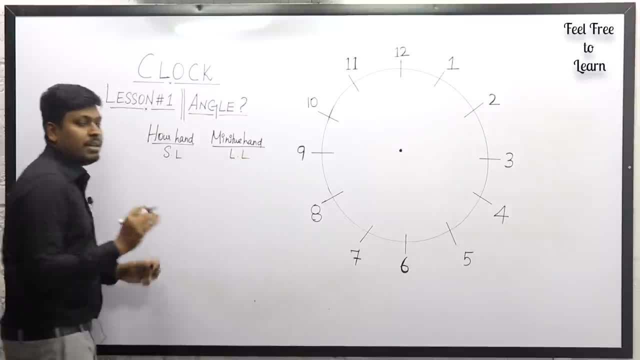 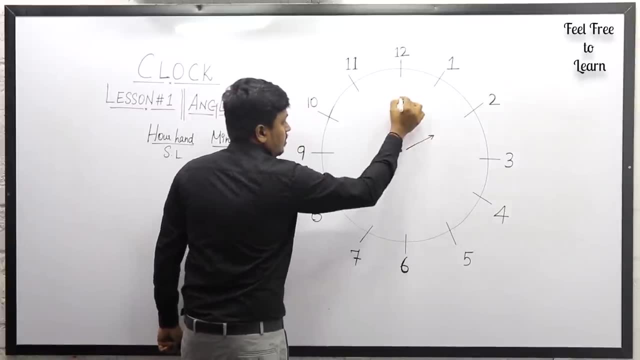 smaller in length and longer in length. we usually call it as a minute, and or else I can do one thing. I can just make a time as two o'clock, right? So two o'clock, So here you can able to see this: two o'clock right. 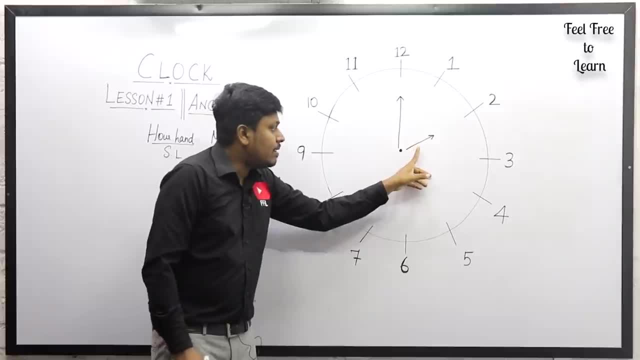 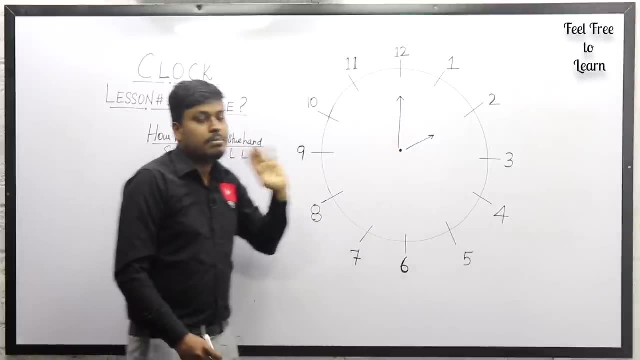 In this two o'clock where this is called as an hour, and So here hour and points at number two and minute and longer in length. we usually call it as a minute and So minute and points at number twelve, understood. and second thing is: first, let we learn what is the basic of a clock. 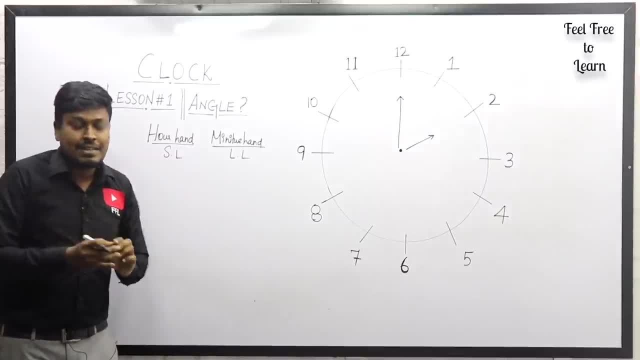 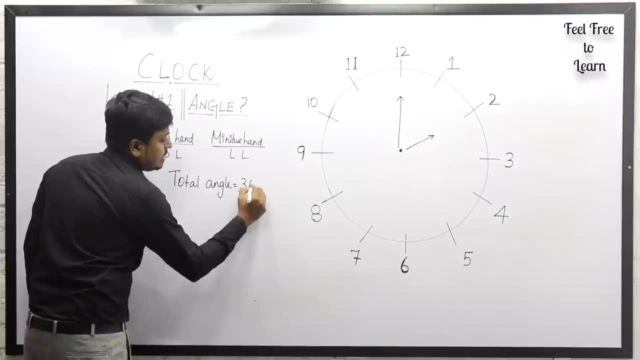 you know that clock in a circle, so which has a 360 degree, so the total angle. so total angle is 360 degree because of a circle. we are saying that the total angle is 360 degree and remember that this 360 degree, the total circle, right? so this 360 degree, 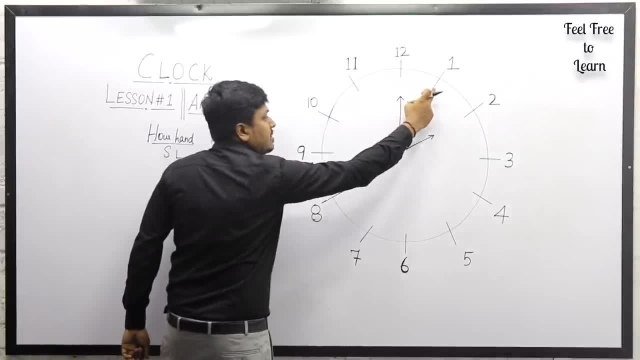 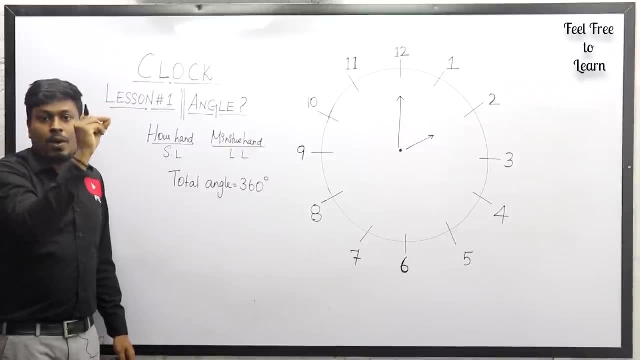 is divided into how many parts, 12 parts. you can able to see 1, 2, 3, 4, 5, 6, 7, 8, 9, 10, 11, 12.. so we can say the total 360 degree clock is divided into 12 sectors, or else 12 gap. 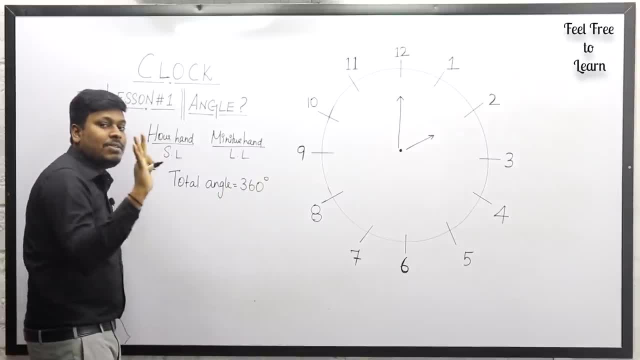 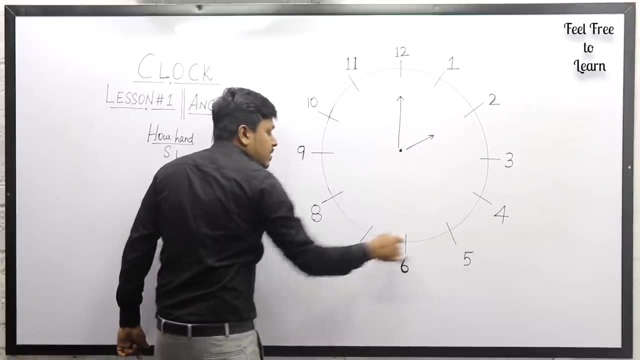 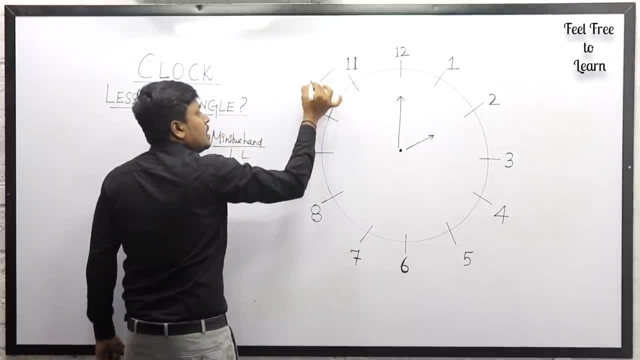 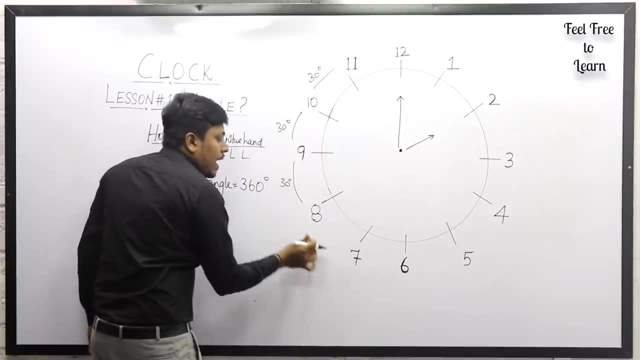 degree: 30 degree, 30 degree, that's what i'm saying. so 11 to 10 to 11, so this will be 30 degree. 10 to 9, this will be 30 degree. 9 to 8: 30 degree. so if you add all the 30 degrees, the resultant will be 360. 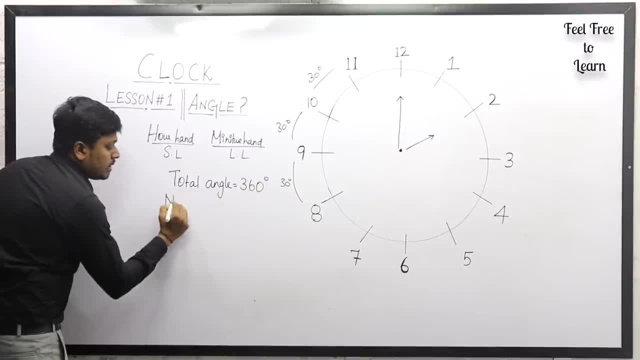 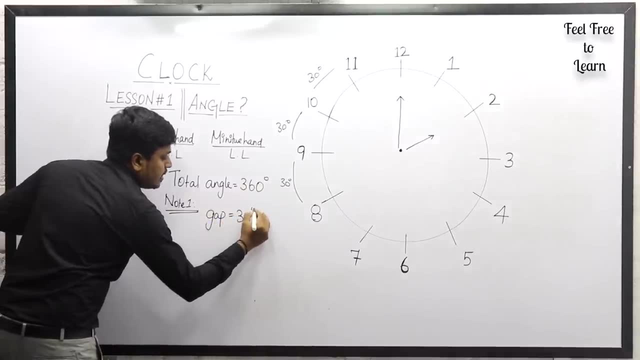 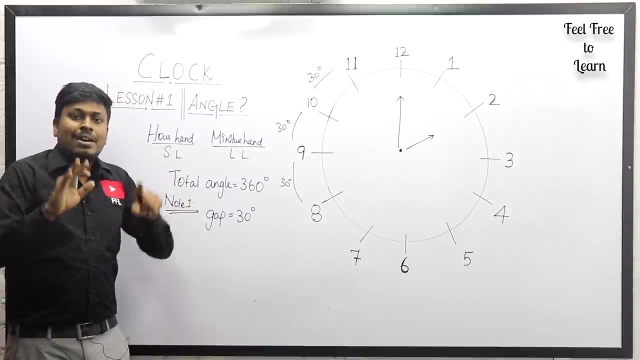 degree. so first note number one. so note number one is what you need to remember is every gap is 30 degree. some students will say it's one sector or some students will say it's a gap, it's you are wish. but remember that where 360, the total circle, 360 degree clock is divided into 12 sectors and 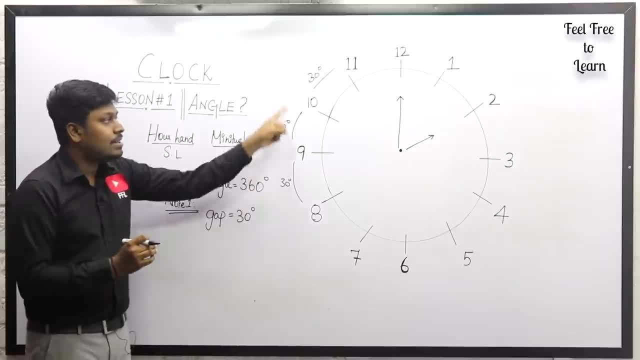 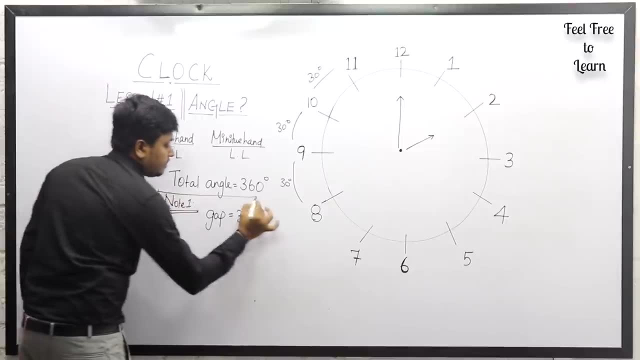 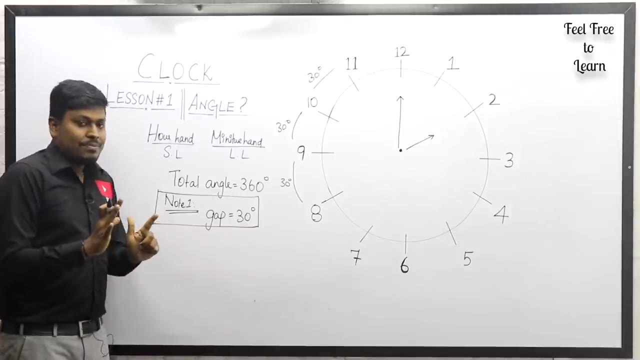 the each gap which determines 30 degree. so 30 degree, 30 degree, 30 degree, that's what we are saying. one gap is equals to 30 degree, understood? so this is note number one, first point. and the second important thing is remember that from- let me take this as an example- two o'clock right now. 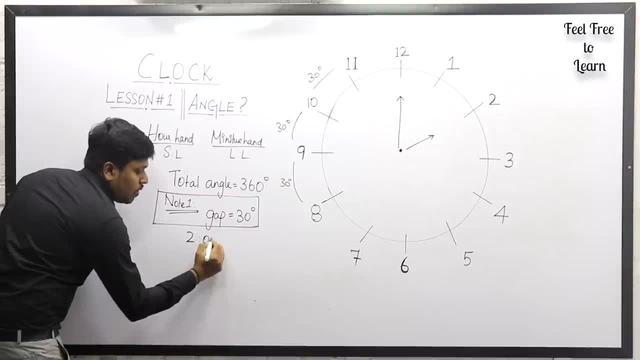 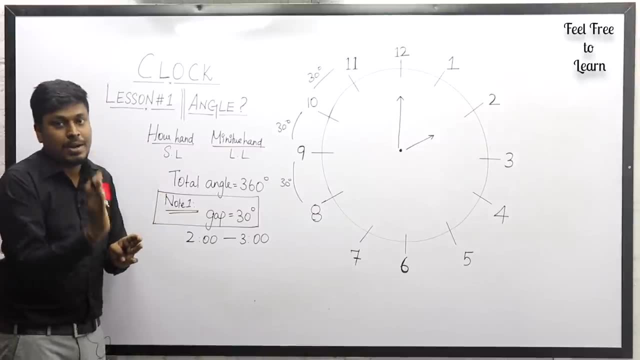 the time is two o'clock right in this. so this is the time when the time is 2 o'clock to 3 o'clock, how much the minute and rotates and how much the hour and rotates. that is most important. you can see from two o'clock in order to become three o'clock, where the minute and right minute and will make a 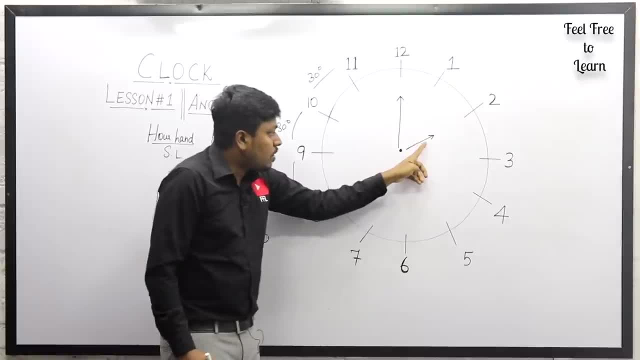 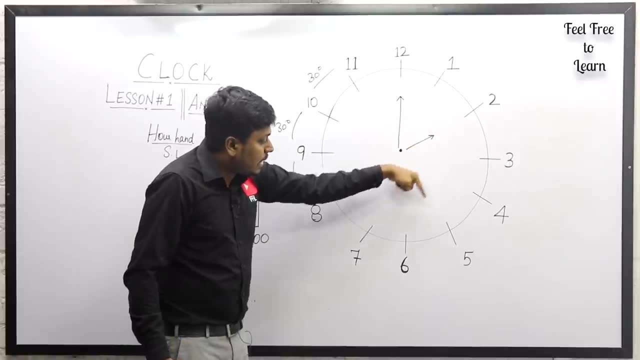 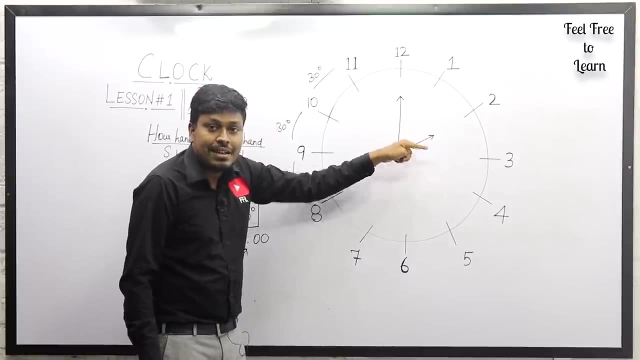 complete rotation, yes or no, right, you know, from two o'clock in order to reach three o'clock. what we how? the clock rotates usually the minute and right the minute and will make a complete rotation, But R and will make only the small distance, which is 30 degree. 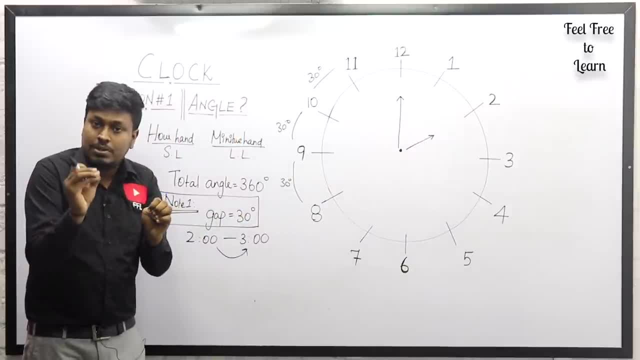 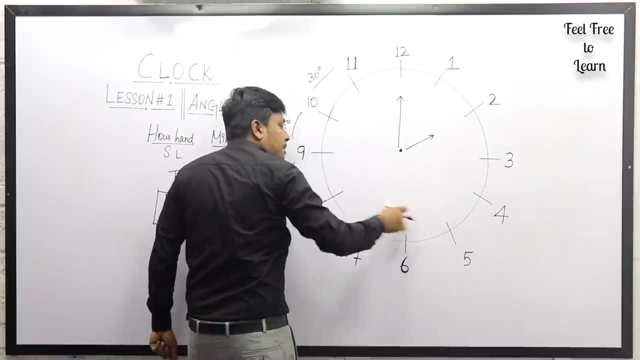 Yes or no Right. Got the logic right From 2 o'clock to 3 o'clock. In order to move from 2 o'clock to 3 o'clock, Where the minute and right This minute and makes a complete rotation. 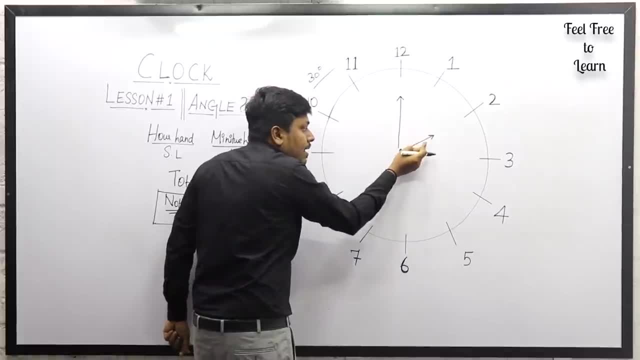 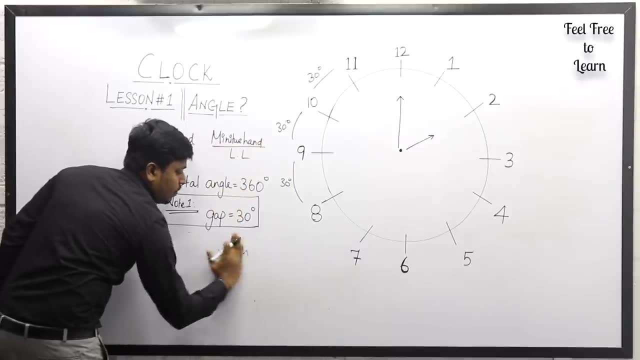 But this R? and is not making a complete rotation. This R? and will make only the small rotation, that is 30 degree. So just listen carefully. what I am going to do is So for 1 hour, for each hour where the minute and travels 60 minutes. 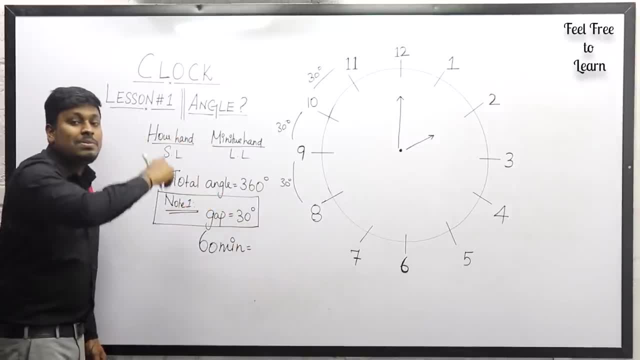 Yes or no. It makes a complete rotation, So minute and moves 60 minutes. complete rotation, But R and will move only 30 degree. Understood this logic. So, friends, minute and makes a complete 360 degree rotation, Which we usually call it as 60 minutes in the clock. 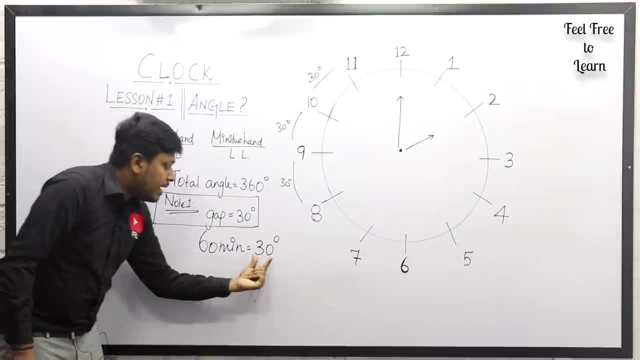 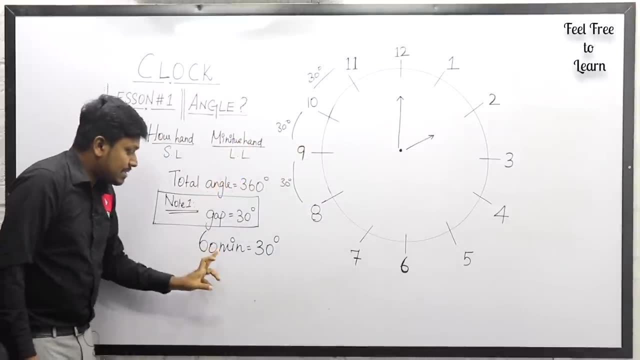 So if minute and moves 60 minutes, Then the R and will move Only this distance which is called as 30 degree. Just now I have said each gap is 30 degree. So 60 minutes minute and moves, Then R and will move 30 degree. 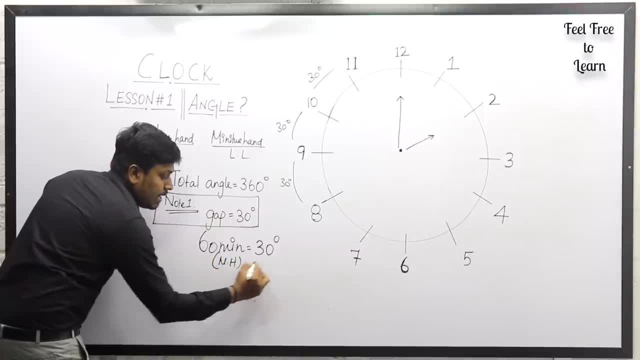 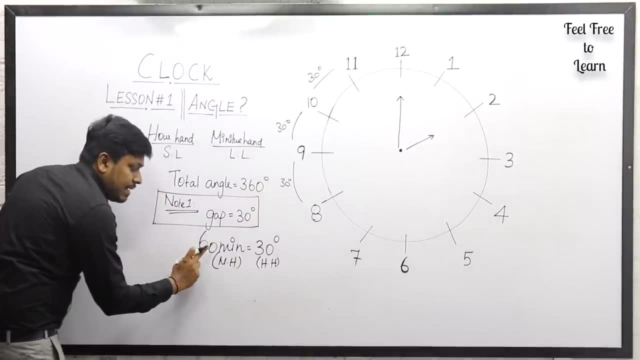 Understood. So this is for minute and- And here I have written for hour and Understood 60 minutes, 30 degree. Another important thing, Just listen here: If 60 minutes is 30 degree, Then 1 minute is equals to half a degree. 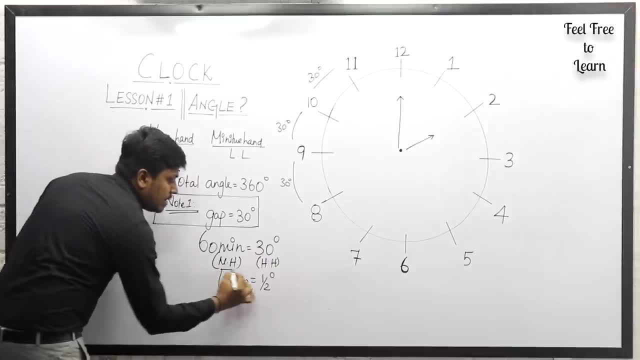 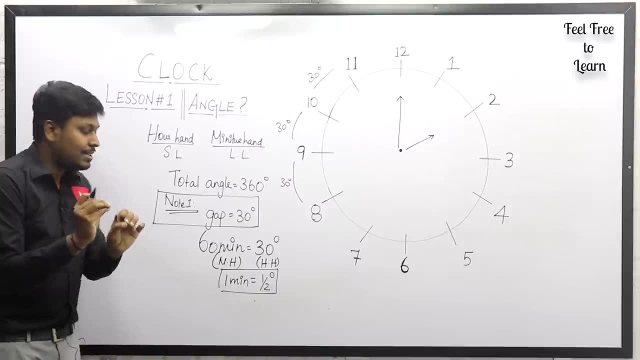 Yes or no, 30 divided by 60 will be half, So 1 minute is equals to half a degree. From this note, where you can clearly able to understand one thing: If a minute and moves 1 minute, Then the hour and will moves half a degree. 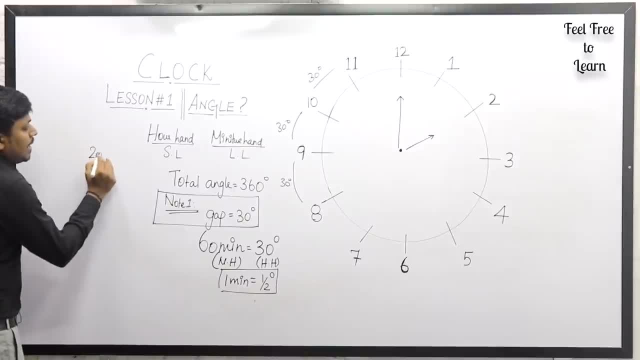 Understood In case: if minute and makes 20 minutes, If minute and right that longer in length, If minute and moves 20 minutes, Then the hour and will moves 10 degree, Yes or no, Because 1 minute If a minute and moves, then the hour and will be half a degree. 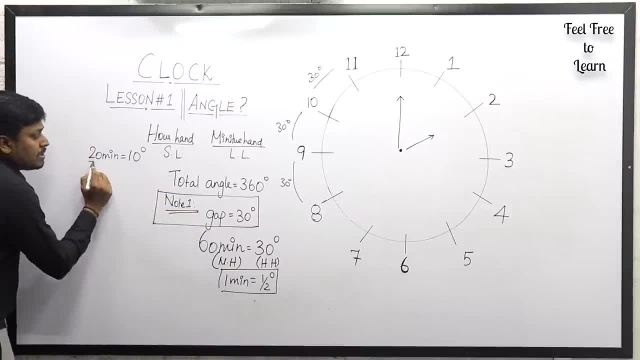 The easy way to understand is If a minute and moves 10 minutes or 20 minutes, whatever be, So half the minute, What is the half of 20, is 10.. So half the minute will be the degree that was moved by the hour and 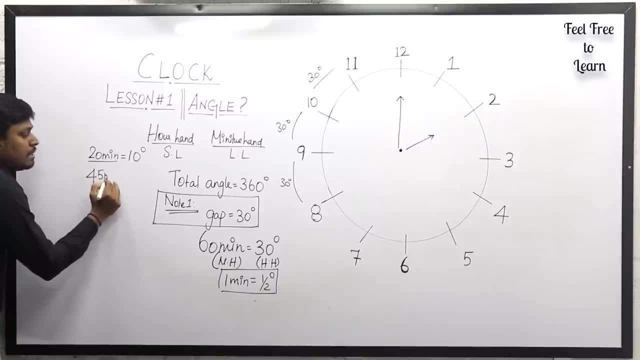 Understood, friends. If a minute and moves 45 minutes- Example- I am saying: If a minute and moves 45 minutes, Then the hour and how much degree it moves divided by 2.. So 45 divided by 2 will be 22.5.. 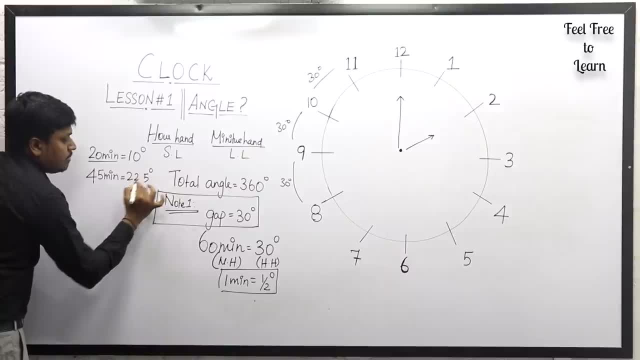 So we can say the hour and the moves 22.5 degree. So this is called as note number 2.. So these two nodes are more than enough to solve most of the question in a clock. So, friends, in case, if you can't able to understand this, kindly rewind this video. 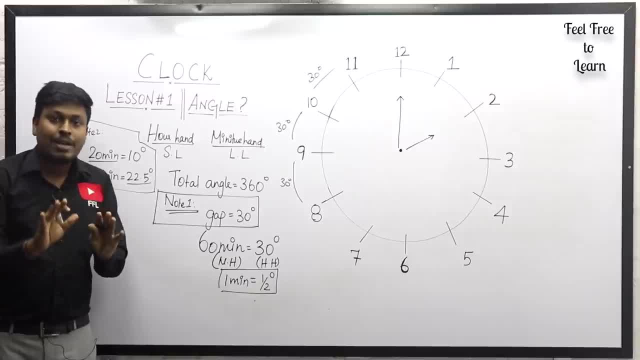 And try to watch again from the beginning. you can surely understand it Right? The note number 1 is where the clock. we know the clock is a circle Which, As 360 degree, and this 360 degree is separated into 12 sectors or a 12 parts. 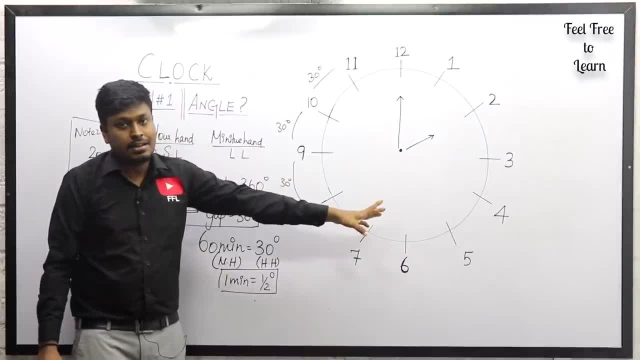 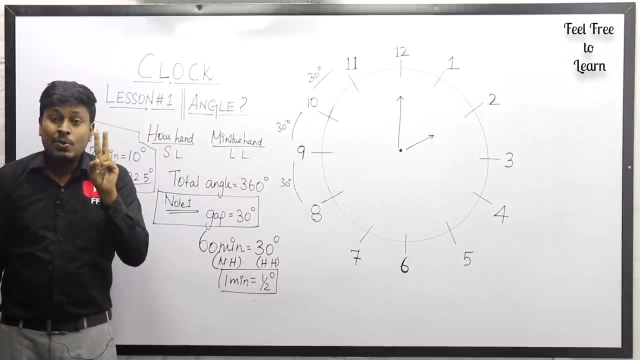 So we can say that each part is 30 degree, 30 degree, 30 degree. That's what I am saying in note number 1. each gap is 30 degree. So this is note number 1, and note number 2 is in order to make 1 hour. 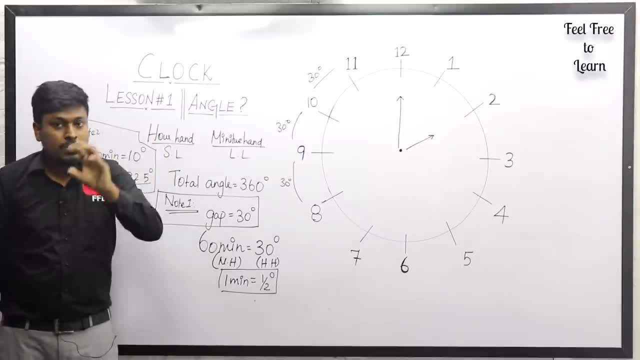 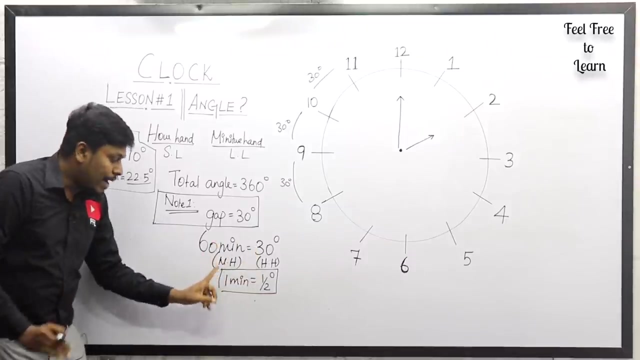 For example, I have taken 2 o'clock here, from 2 o'clock to 3 o'clock in order to make 1 hour, where the minute- and makes a complete 1 rotation, That's is time between- will be the degree that was traveled by the hour hand. So when a minute and move 60 minutes, hour hand will makes only 30 degree. it moves only 30 degree. So what I'm saying is one minute. if a minute and moves, then the hour hand will move half a degree. So from this point where we can say if a minute and moves 20 minute, So half the minute will be the degree that was traveled by the hour hand. 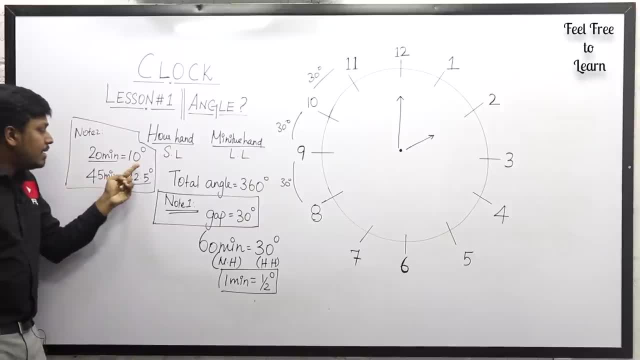 rand understood this minute. half will be the degree that is, travel by the rand, right, if it is 45 minutes the minute and travels 45 minutes, then we can say half the minute, 45 divided by 2 will be 22.5. so this 22.5 degree where the hour and moves. understood, friends, this is one of the 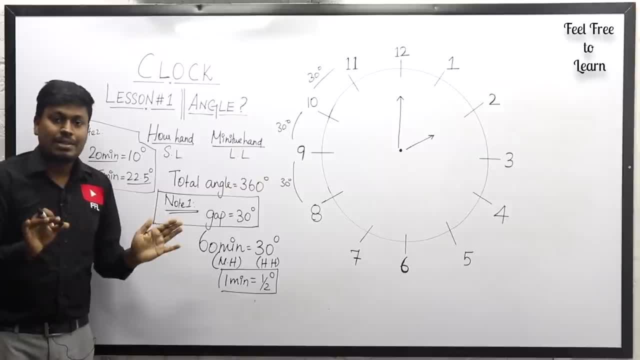 most important logic in the topic log. if you understand this, then solving most of the question will be very, very simple. so once here, i am going to solve 6 to 7 question by taking a random numbers. so after watching this video, try to practice minimum of 30 to 40 question on your own. 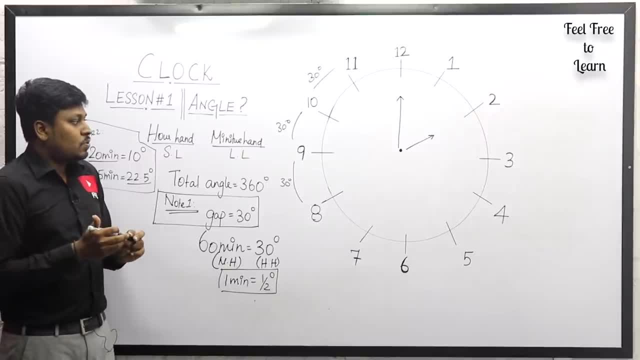 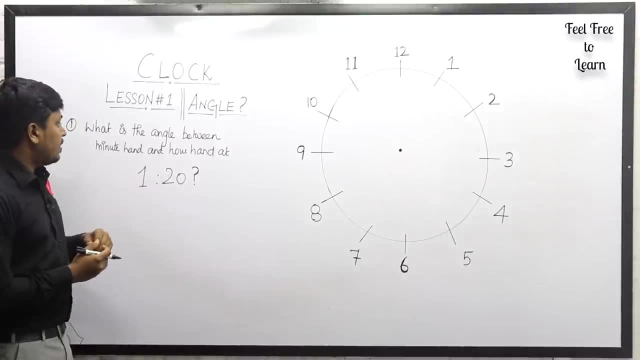 so only then you will get an idea right. so let me move on to all the 8 to 9 questions. question number one: so what is the angle between minute and and r and at 120? so our target to find what is the angle between minute and hour and at 120. so our target to find what is the angle. 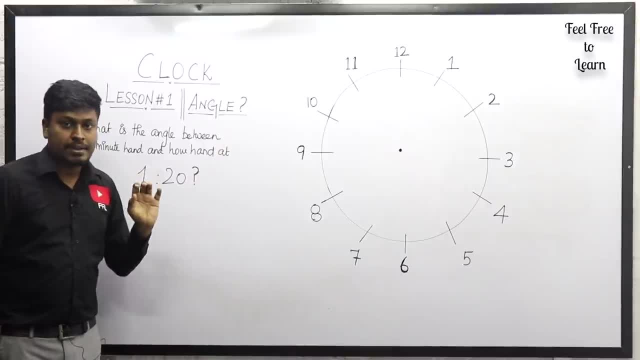 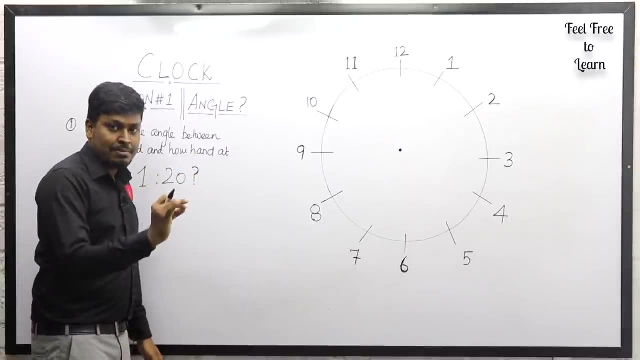 between minute and at an hour and at the time of 120. so first what we can do is we can draw the diagram in the clock right. so after that finding an answer will be very simple. just see here. we know that 1 for our and and 20 will be. 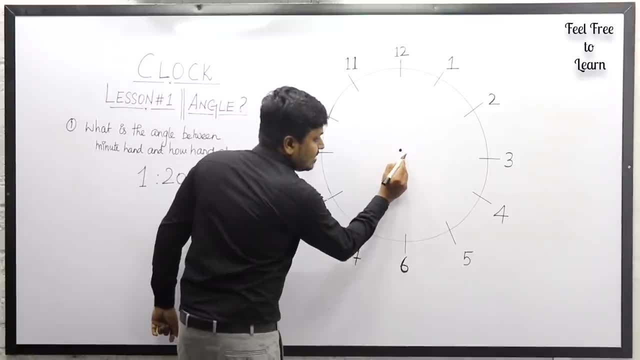 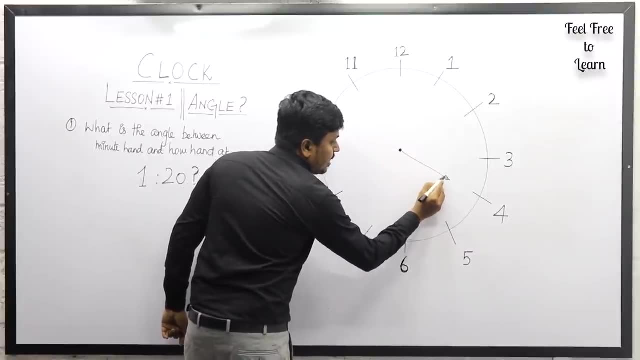 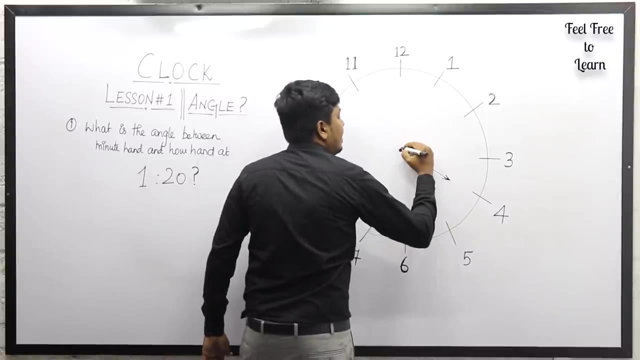 for a minute and so 120 how the clock look likes. just listen carefully because of 120, where we can say the minute and right exactly points at number 4 yes or no when it and. but our and will not exactly. points at number 1. it is. 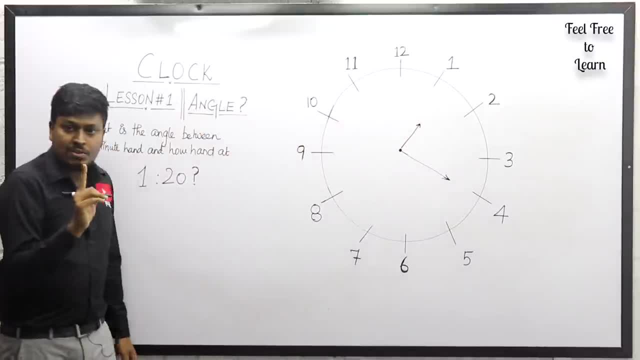 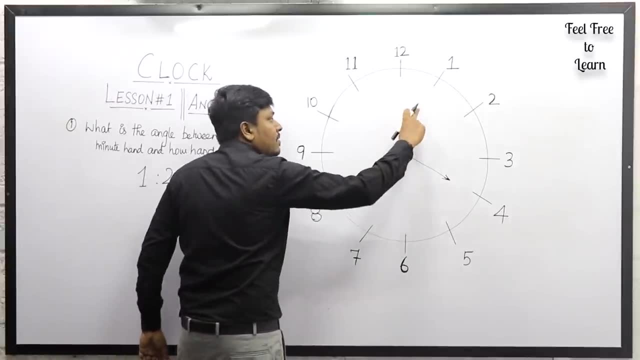 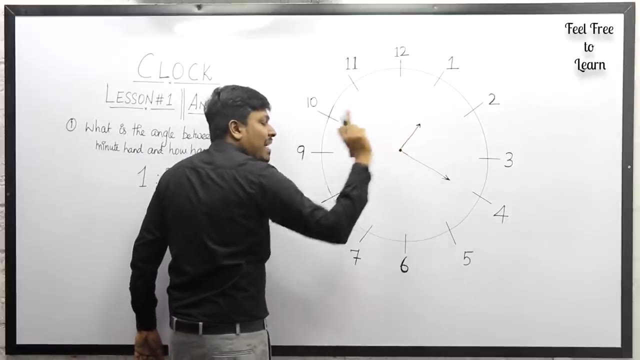 somewhere around between 1 to 2. so friends understood this logic only at 1 o'clock, right, only at 1 o'clock, you can able to see where this are and will point exactly at number 1. but now the time is 120. so in the time 120 where we 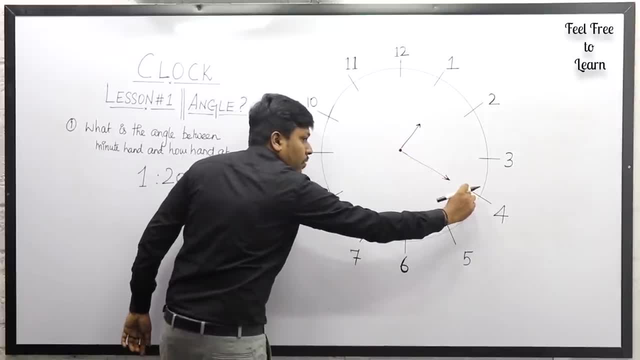 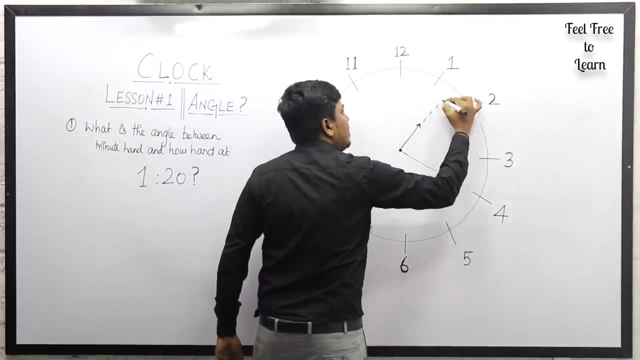 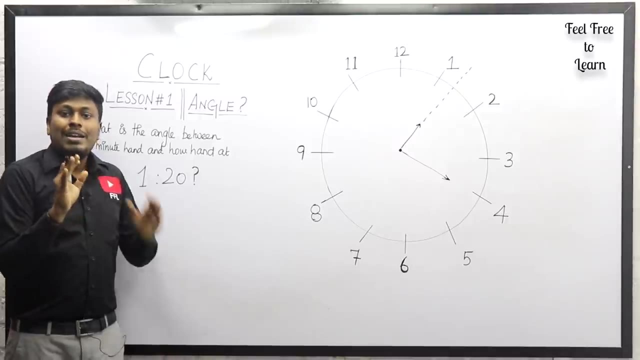 can say the minute and will exactly points at number 4, but this our and will not exactly points at number one. this r and will point somewhere between one to two, understood? so this is the first point. you need to remember this. never forget that. only at one o'clock where. 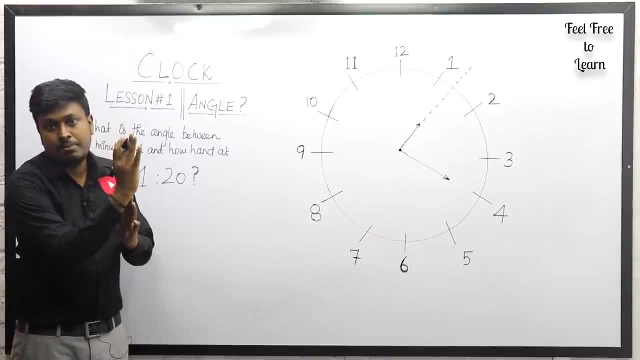 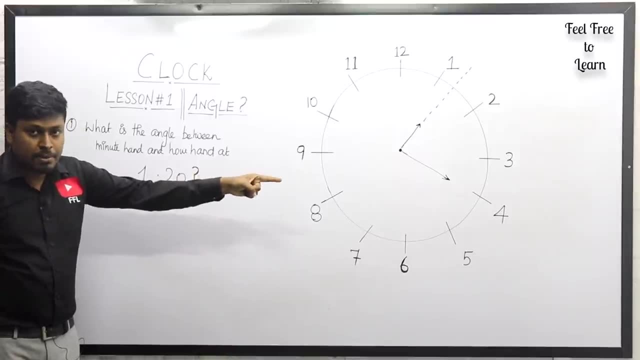 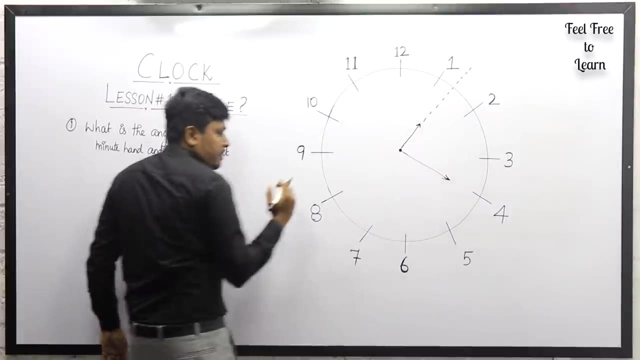 you can able to see that r? and will exactly points at number one, but now the time is 120 right, so definitely we can say minute and will exactly points at number four, but r? and will not exactly points at number one. it's slightly somewhere between one and two. so now what is our target? 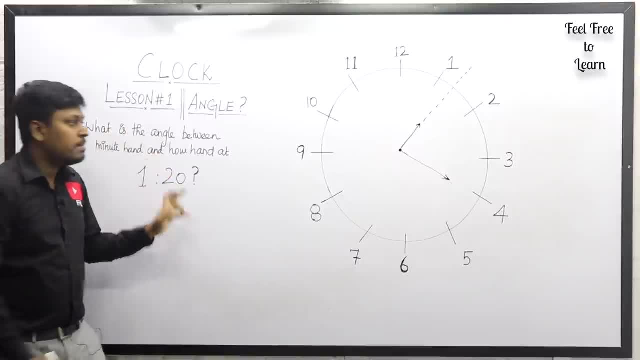 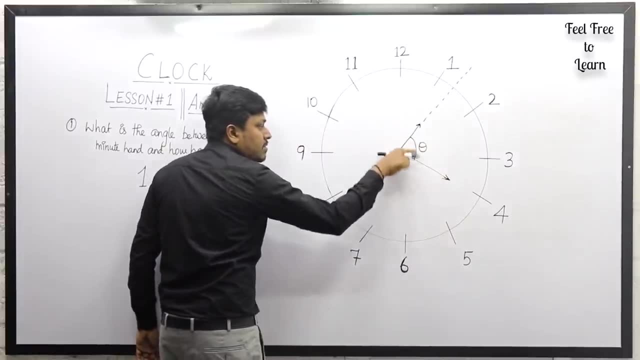 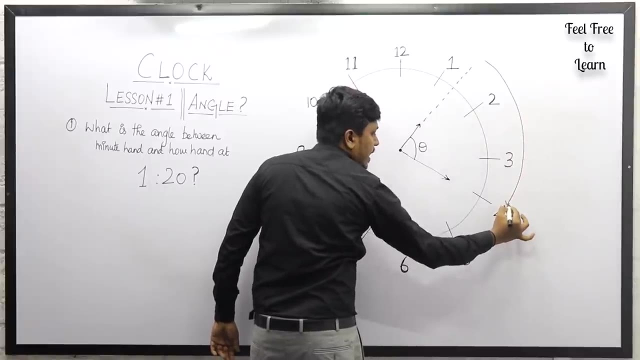 our target to find what is the angle between r and and a minute, and which means our target to find what is the angle of it. so, angle between r and and a minute. this is a target. so just listen here from this point right. so from this point we need to find what is the angle, understood or not? this? 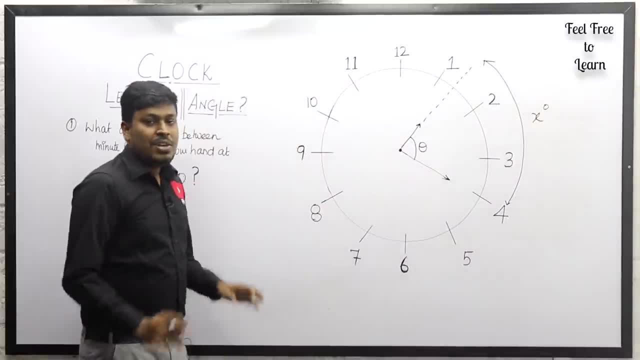 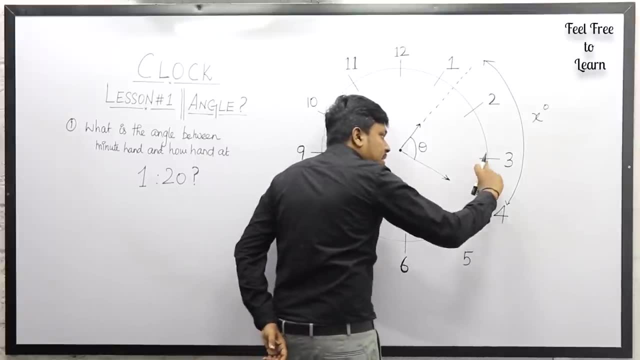 is our target, so what angle it is. understand, and we know that according to note number one, what i have said is each gap is how much degree? 30 degree, so we can say three to four is one gap. yes, so this will be 30 degree and similarly two. 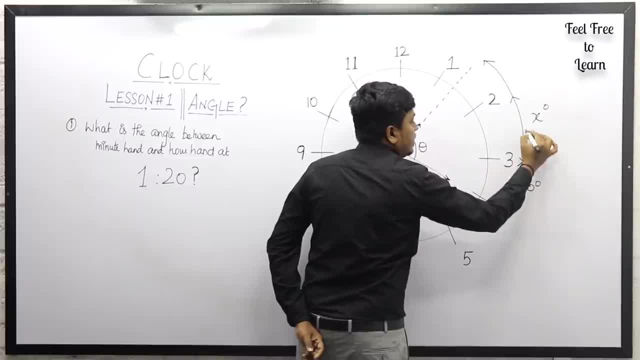 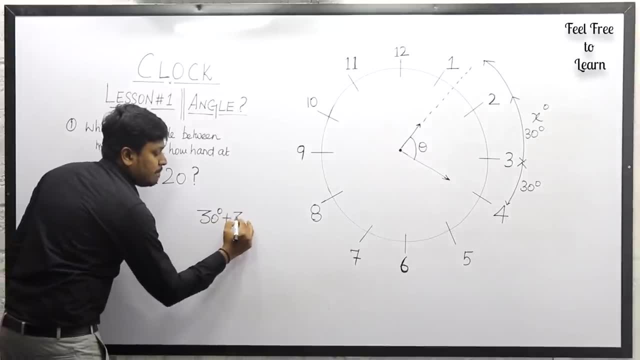 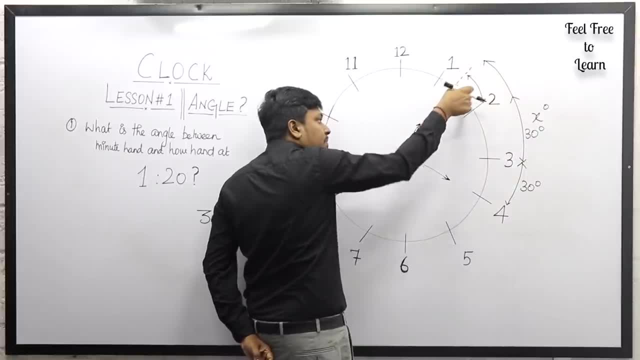 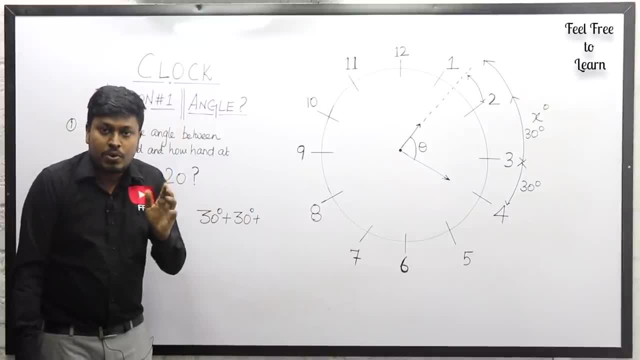 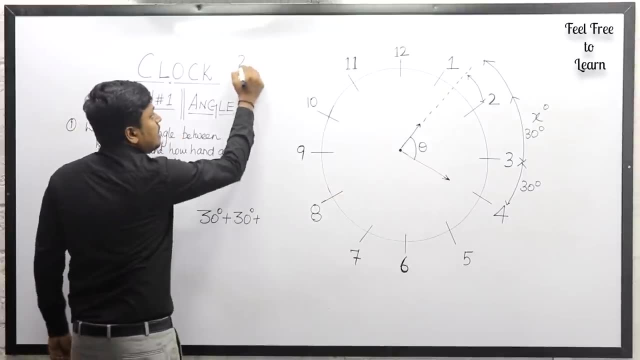 check how much this r and moves from point one. just now i have told you, according to note number two, target the minute and how much the minute and moves. here 20 minutes. so 20 minutes, where the minute and moves is equal to half the minute, will be the degree that was moved by the rn. so what is the half of this number is 10.. 0.148. so i just want to check that. i think it should be at normal. it should be construction time. it should be half Celsius. 40 000, which is sogenan d數 60ми of 90 m 93m. 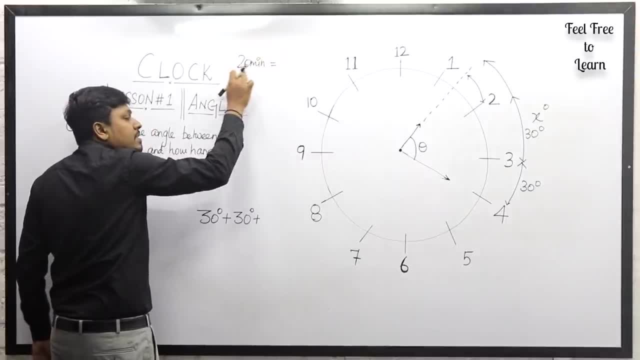 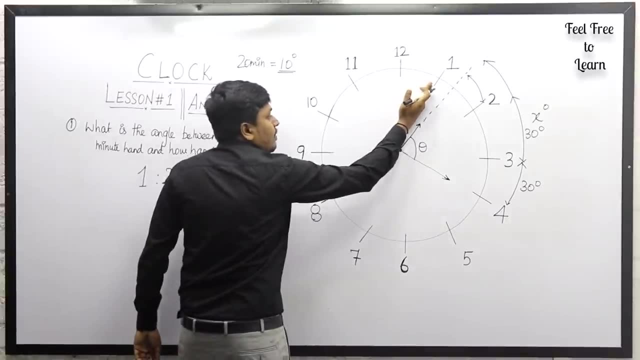 so that is what we are going to get in light of that. so that means that rnd in this range of this angle can towards moved by the r and so what is? the half of this number is 10, so 10 degree where the r and moves from number 1, so from 1, where this r and moves 10 degree. so if this is 10 degree, then this: 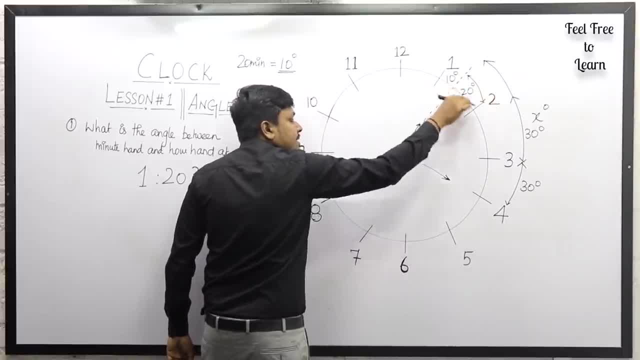 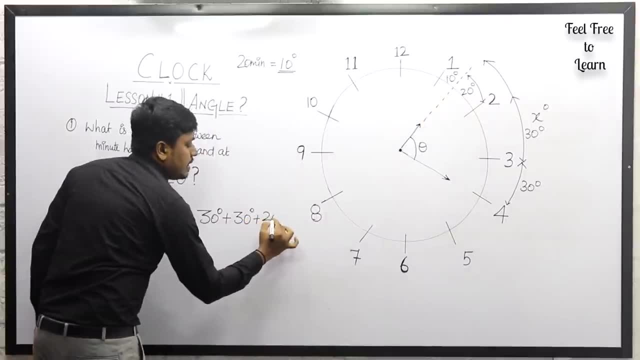 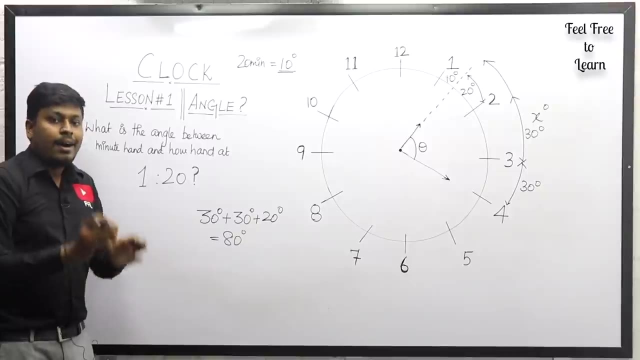 will be 20 degree, understood, because the total degree is 30. so we can say: if this angle is 10 degree, then the remaining will be 20 degree. so we can say 30 degree, 30 degree plus 20 degree, so resultant will be 80 degree. so now the angle between the r and and the minute, and at the time. 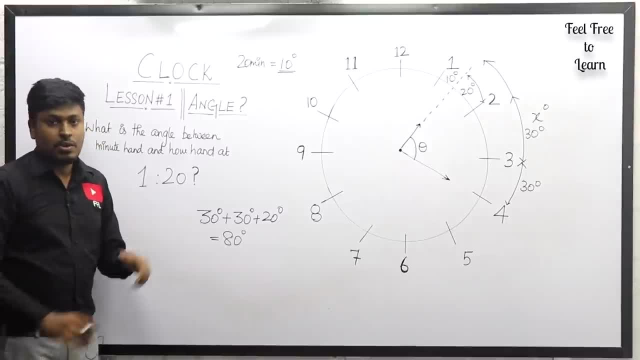 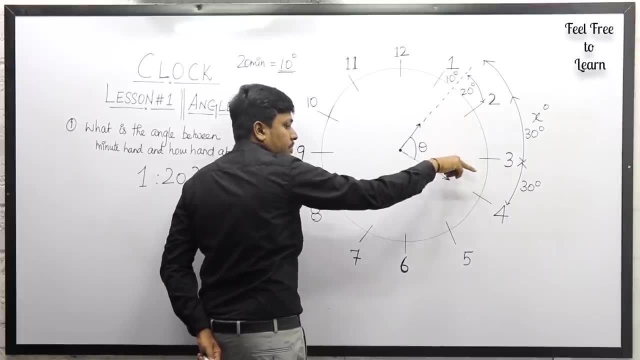 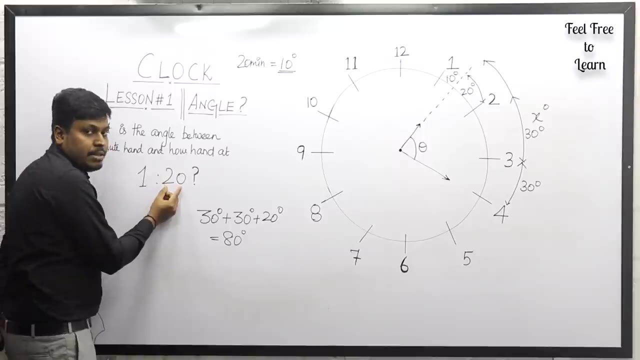 of 120 is 80 degree, understood or not? because our target to find the total angle right, so 30, 30 plus 20, so the total angle will be 80 degree. understood how i found it is 10? so just listen carefully. we know that the minute and moves 20 minutes. so, according to note number 2, what i have said is: 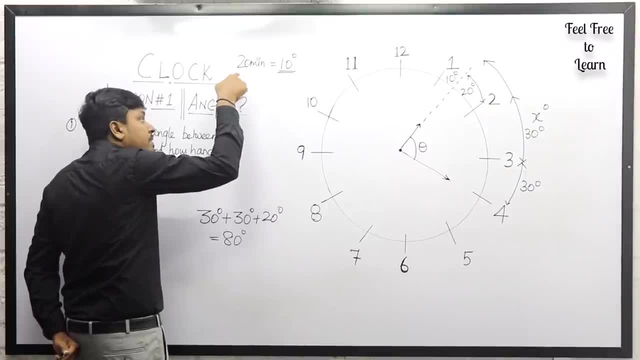 if a minute and moves 20 degrees, then the total angle will be 80 degree, so the total angle will be 20 degree. so if a minute and moves 20 minutes, half the minute will be the degree that was traveled by the r, and so half of 20 will be 10. so 10 degree r and moves from number 1, so from 1. 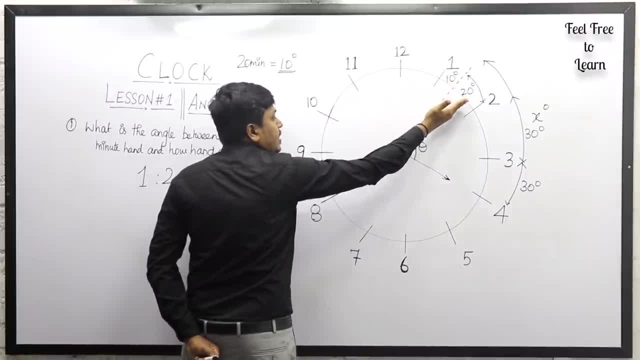 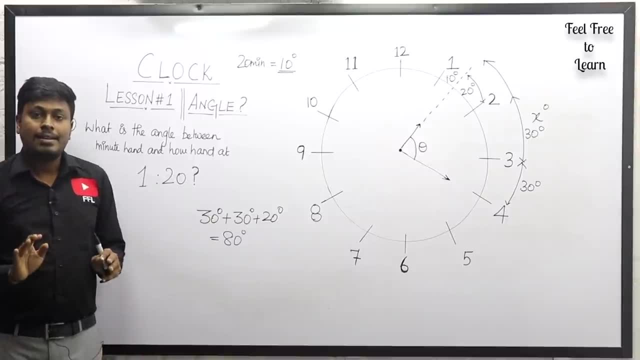 it moves 10 degree, so the remaining will be 20 degree, so 20, 30, 30. so the angle between r and and a minute and is 80 degree. so this will be the answer for question number 1. understood? so a beginners. okay, if you can't able to understand it, just try to understand, or else. 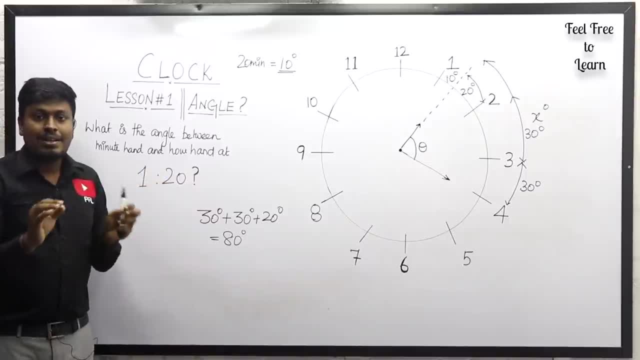 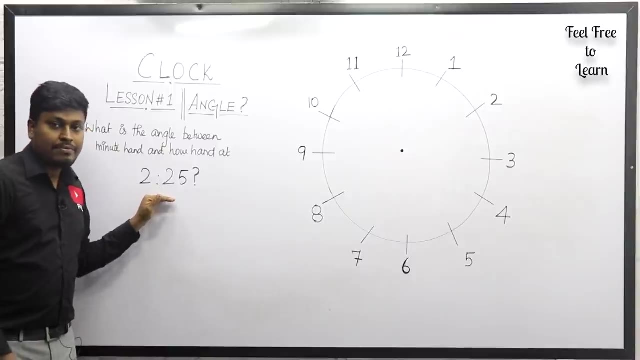 i'm going to solve a remaining 5 to 6 question. surely after watching all the 5 to 6 question you can able to understand it right. so finally, answer for question number 1 is 80 degree. question number 2: so what is the angle between minute and and r and at a time of 225? so our target to find 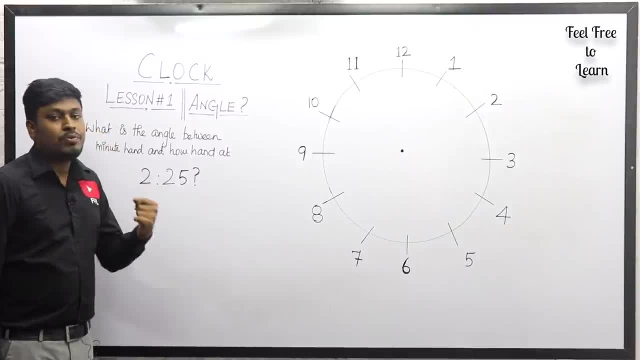 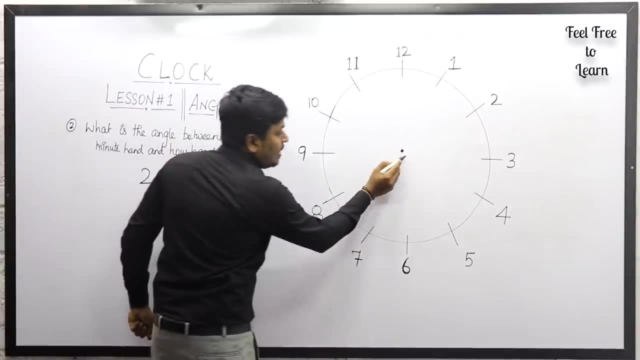 what is the angle between r and and a minute, and at a time of 225. so first try to draw a diagram, right so in 225, where you can say where the minute and will exactly be the angle between r and and exactly points at number 5, why? because it is 25 minutes, right? so, because of 25 minutes where we 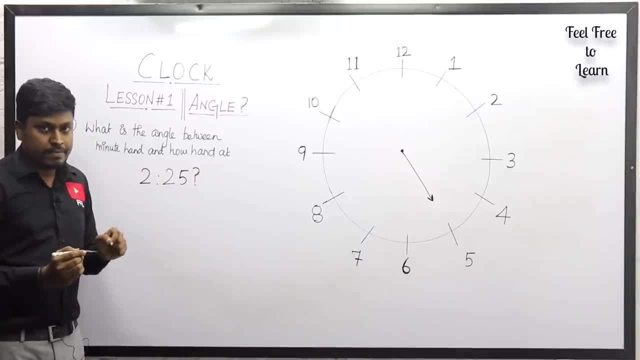 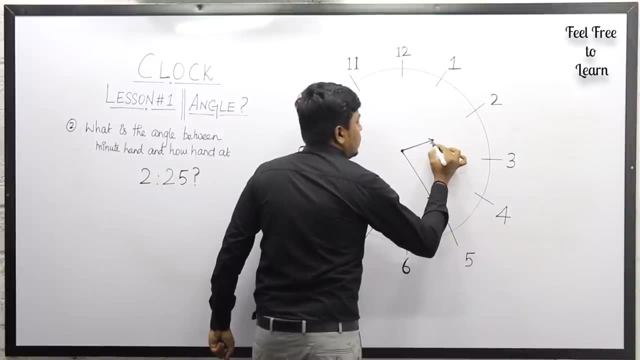 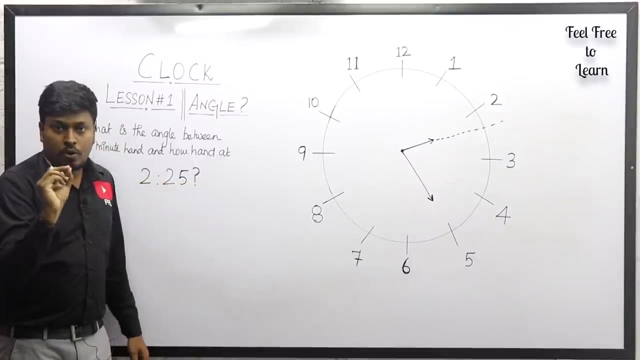 can say minute and will exactly points at 5, but r and will not exactly points at number 2. it it's like points somewhere between 2 and 3. we don't know where it points, but it it points somewhere between 2 to 3- understood only at 2 o'clock- where we can say the r and will points exactly at number. 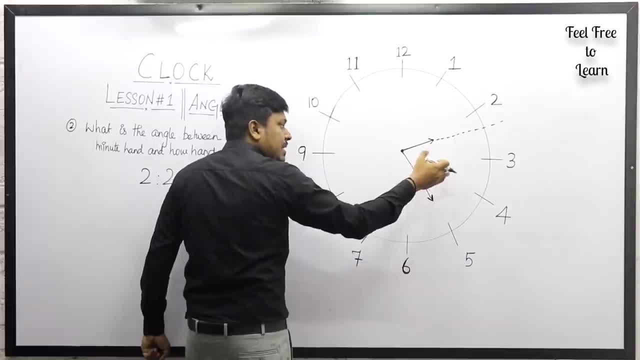 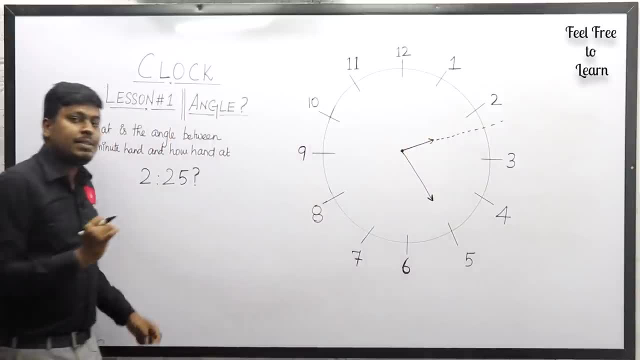 2, but here the time is 225, so definitely we can say r and will not exactly points at number 2, it's somewhere between 2 to 3. so now our target: to find what is the angle between r and and a minute. and so this angle, our 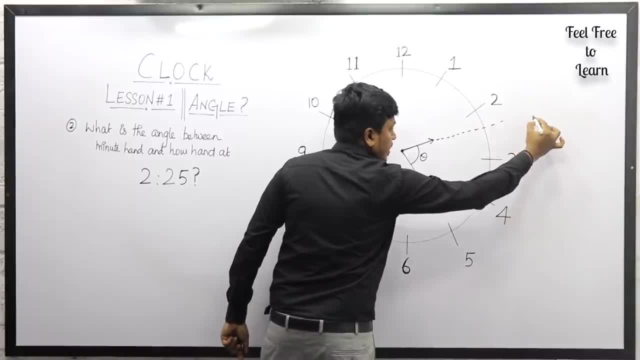 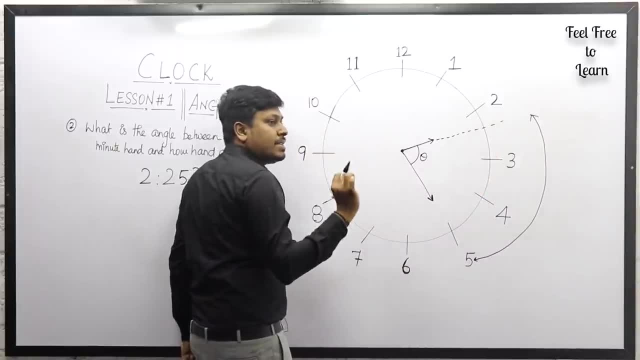 target to find. so just listen here from this area, our target to find this complete angle. so, according to note number 1, what i have said is each gap is 30 degree. so here 4 to 5 is one complete gap, so we can say it's 30 degree again. 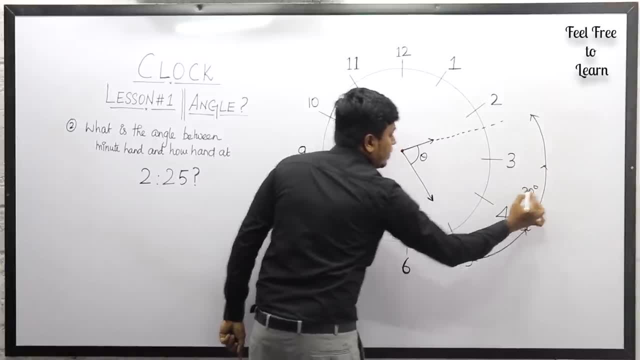 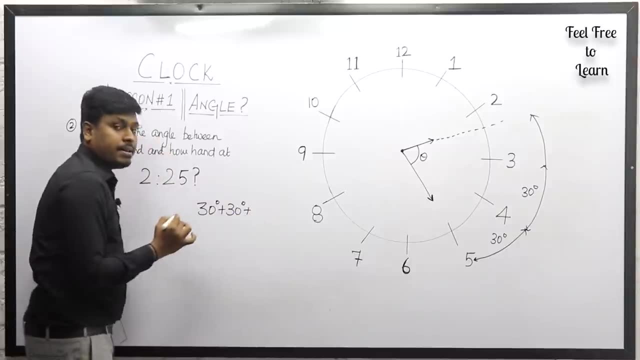 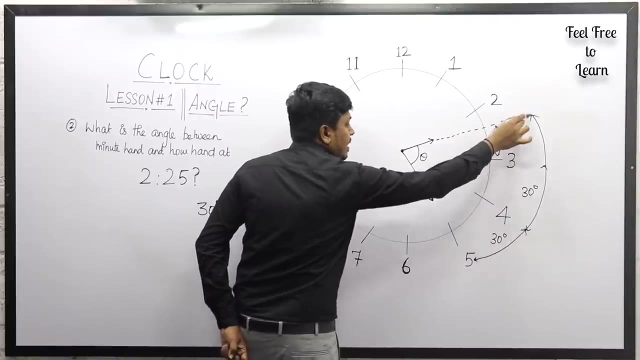 3 to 4 is another complete gap. it's 30 degree, so 30 degree. first is 30 degree and the second gap is another 30 degree and the last part, so last part. our target to find what is this angle is, so only then we can able to see what is the total angle between r and and the minute and 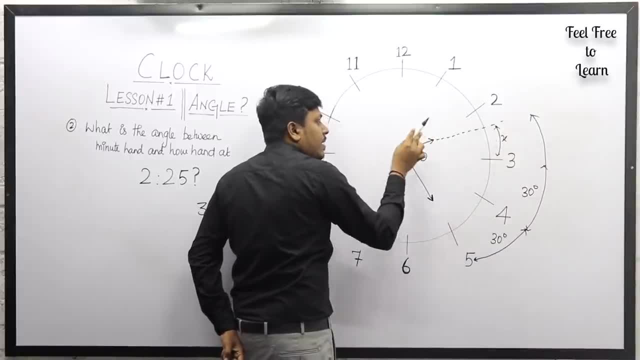 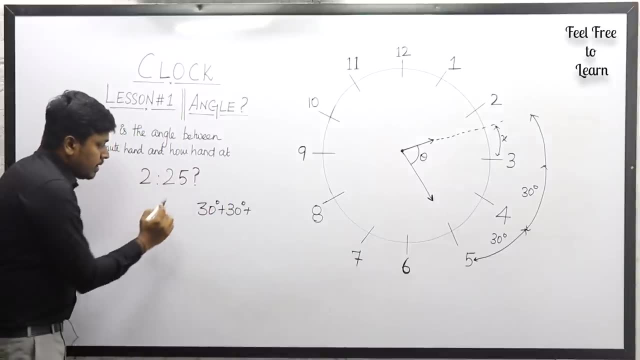 so, in order to find this angle, first we need to check r and from to how much distance it moves. so, in order to find that what i have told you, according to the total angle of the angle between, to note number 2, you can able to see the minute and travels how much minute, 25 minutes, so 25. 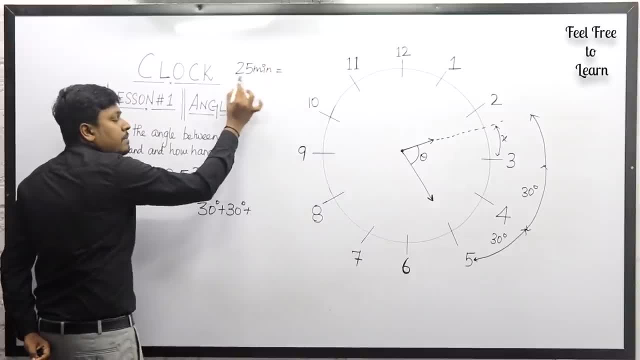 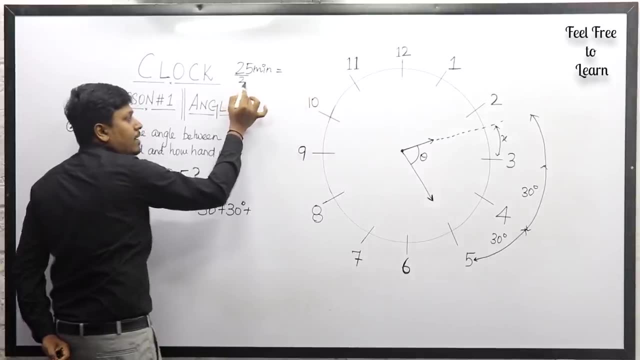 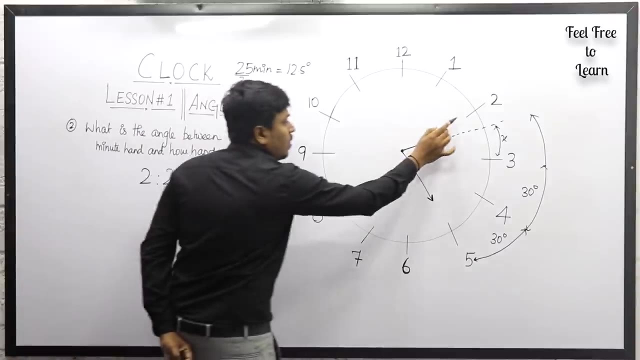 so here you can say: half the minute will be the degree that was traveled by the r, and so half the minute, what is half of this number is 12.5. so we can say: 12.5 degree is the r and which moves from 2, so from 2 o'clock where the r and moves 12.5 degree. understood. so now we can. 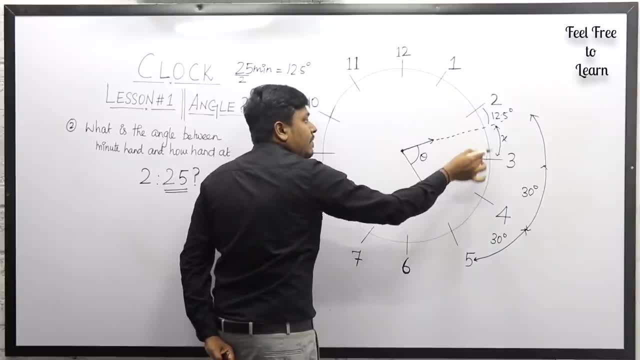 say the total gap is 30 degree from this 30 degree where the r and moves 12.5 degree from 2. so we can say the remaining value is 30 degree minus 12.5 degree will be 17.5 degree. so finally, 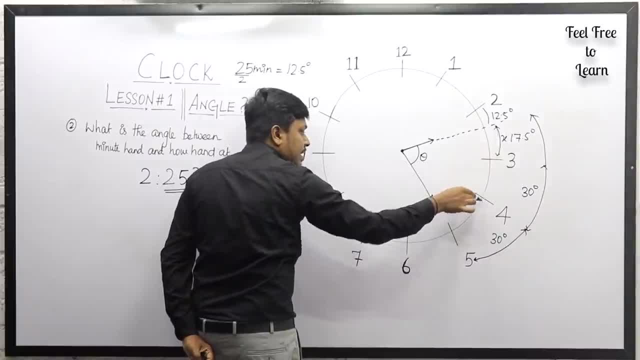 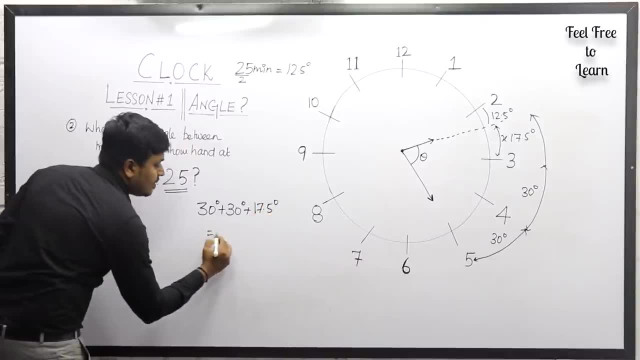 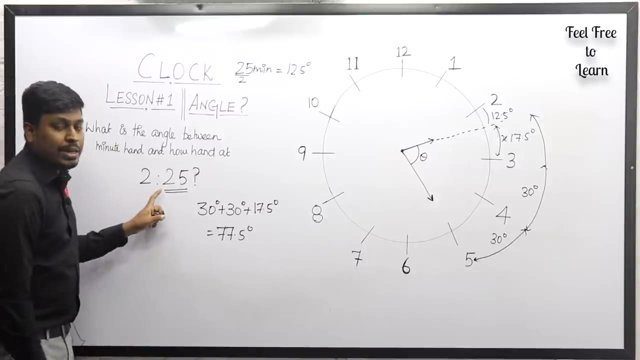 we can say 17.5 degree plus 30 degree plus 30 degree, so 30 degree, 30 degree plus 17.5 degree. so resultant will be 77.5 degree. so angle between r and and the minute and at a time of 225 is 77.5 degree. so, friends understood. so each gap is 30 degree according to note number. 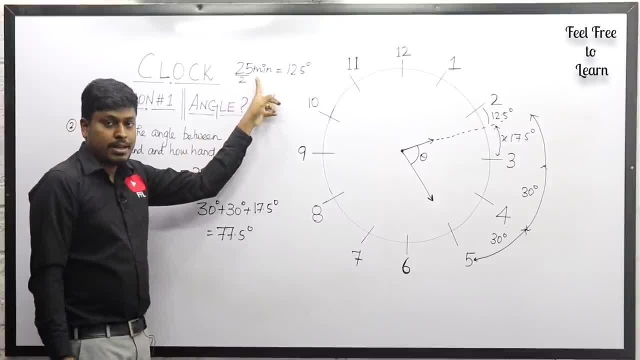 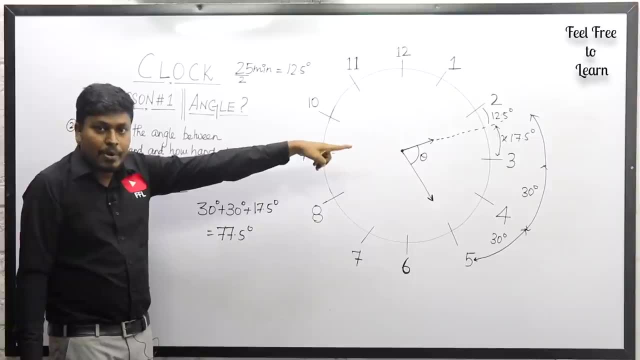 1 and according to note number 2, you need to check the minutes right. so half the minute that was the degree traveled by the r and so from 2 o'clock you can see it traveled 12.5 degree. so now we can say the time of the minute that was the degree traveled by the r and so 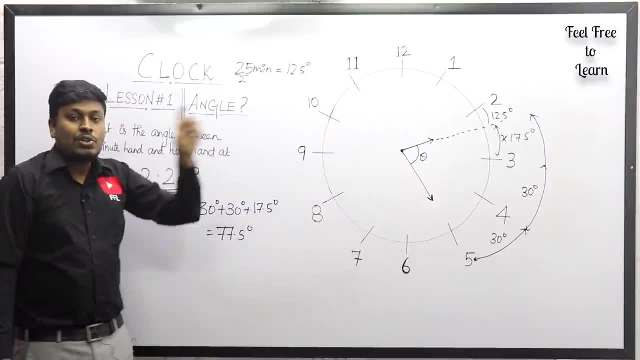 degree. So if r and moves 12.5 degree, then the total gap is 30 degree. So 30 degree total minus 12.5, the resultant will be 17.5.. So 17.5 degree plus 30 degree plus 30 degree, So resultant will: 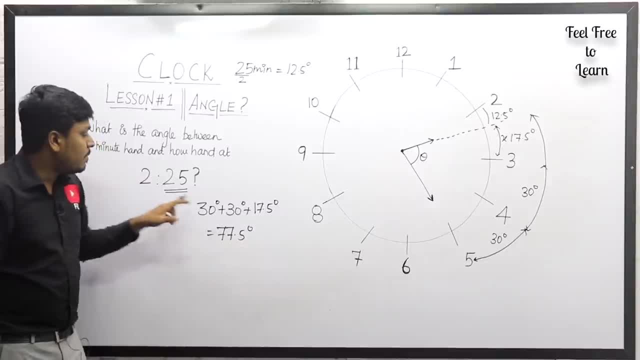 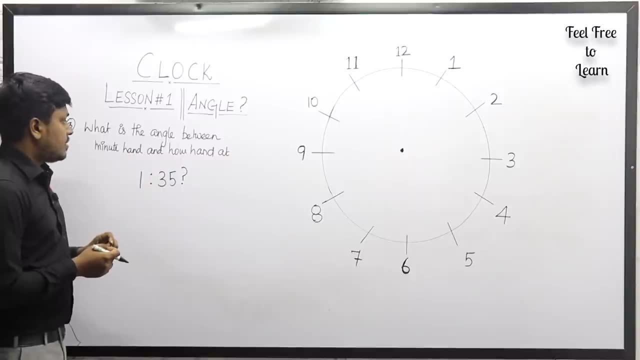 be the angle between r and and a minute and at a time of 225.. So answer for the second question is 77.5 degree, Question number 3.. So what is the angle between minute and and an r and at a time of 135.. So at 135 our target to find what is the angle between both the ands? First let me draw a. 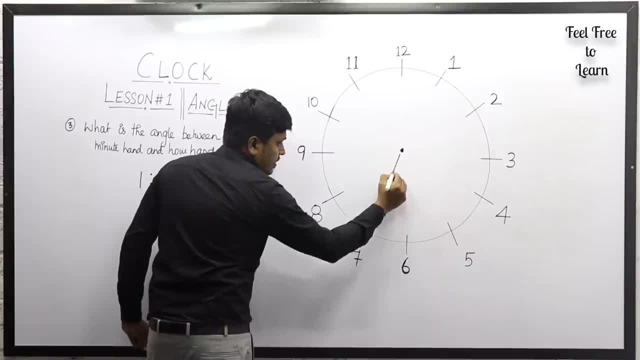 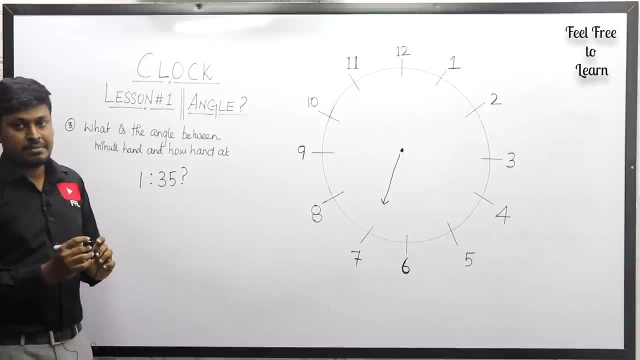 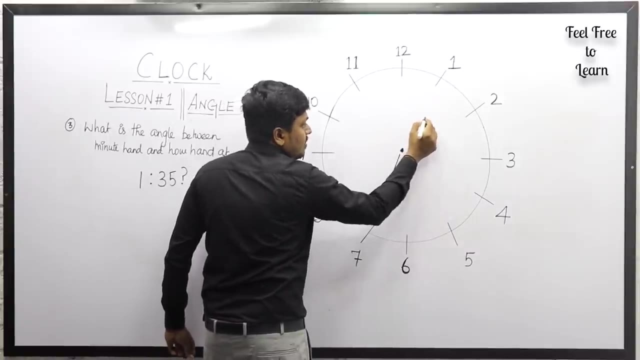 diagram, So 135, where you can say this minute and will exactly points at number 7 because it's 35, right? So we can say it exactly points at number 7.. But r? and will not exactly points at number 1 because it slightly move towards between 1 and 2.. So we can say this r? and will be somewhere. 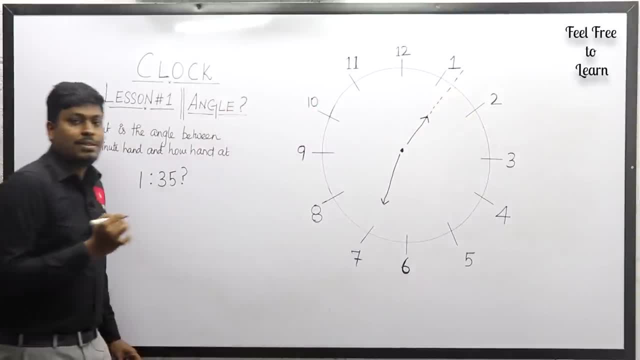 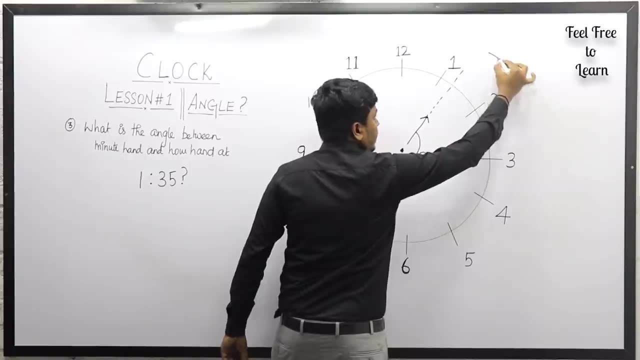 between 1 and 2.. So we can say this: r and will be somewhere between 1 and 2.. So we can say this: r 2 understood this logic. so our target to find what is the total angle between r and at the minute, which means, from this point, our target to find till 7 what is the complete angle. 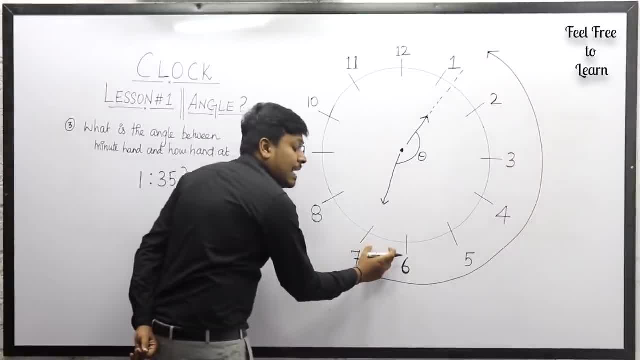 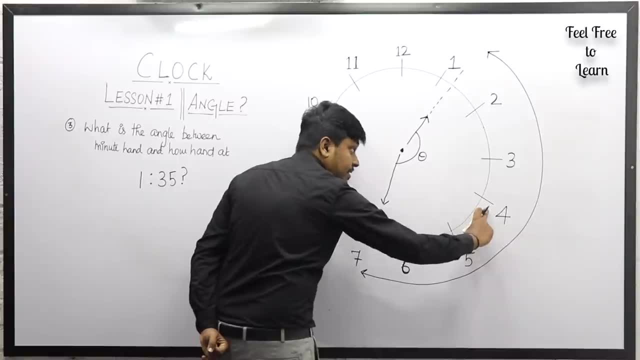 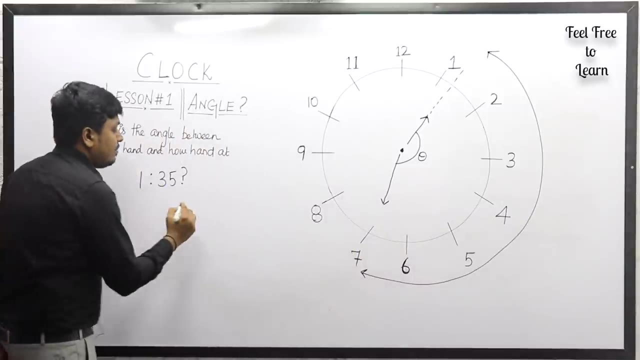 according to note number 1, we know that each gap is how much degree? 30 degree, so first gap is 30 degree, 1. 30 degree, 2. 30 degree, 3, 4, 5. so total 30, 30, 30, 30, 30, 5 gaps. so 30 into 5 will be 150 degree. 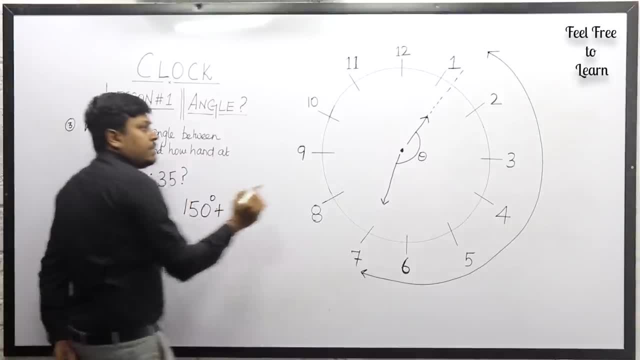 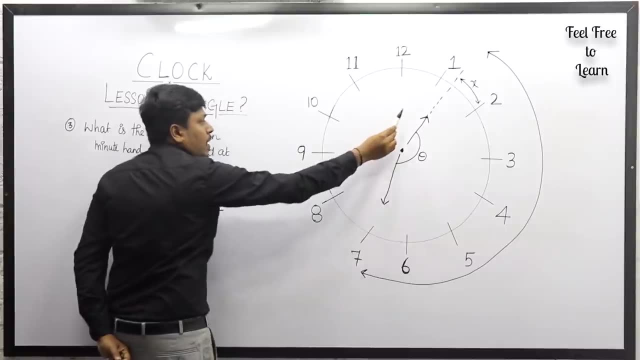 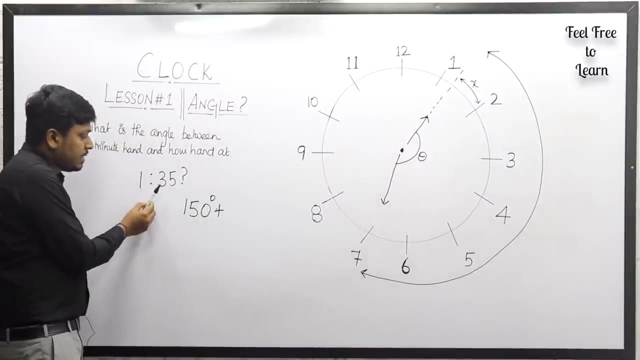 so the total is 150 degree plus and the final is our target to find this remaining degree. just listen here, from 1, where the r and moves. how much degree? how will you find this? in order to find this, our target should be on the minute and we are the minute, and 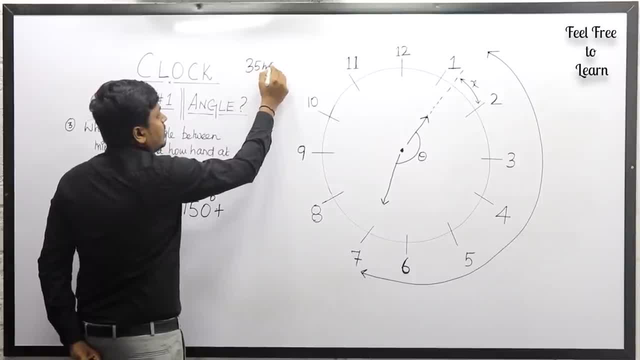 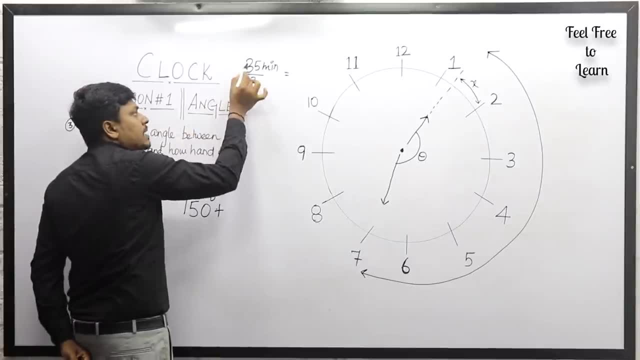 travels 35 minutes. so 35 minute. so half the minute will be the degree that was moved by the arrogant. so half of 35. so 35 divided by 2 will be 17 point 5, so we can say 17 point 5 degree. 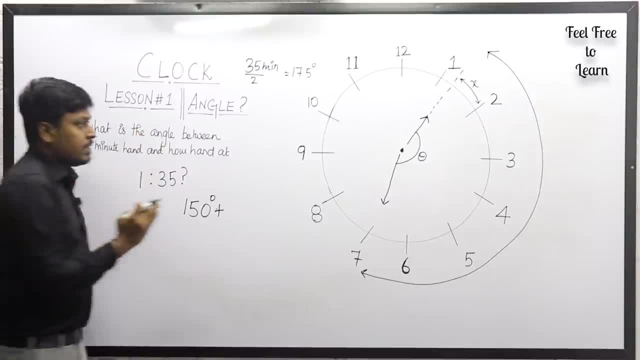 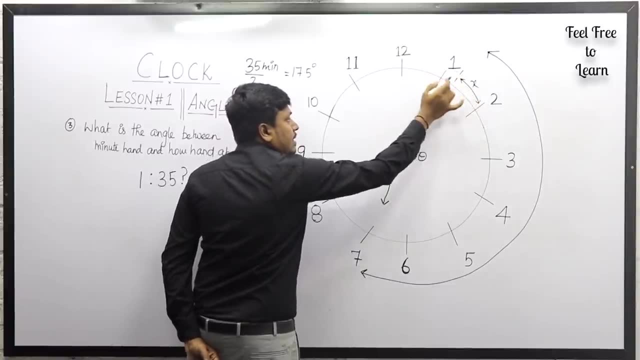 verter are: and moves from 0.1. so from 0.1, where r, or, and move 17.5 degree. so the total is 30 degree and this is 17 point 5 degree. so what? only the remaining distance, 30 degree minus 17.5 degree, will be 12.5. so this angle is 12.5. so finally, we 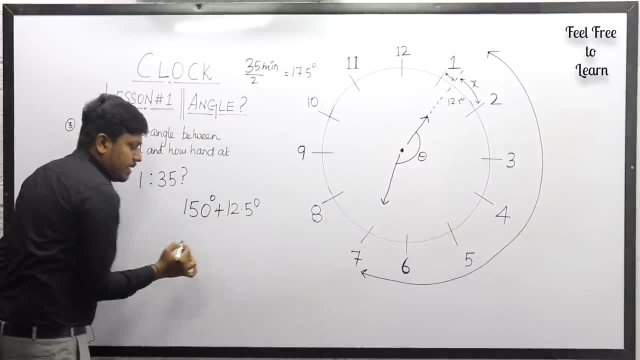 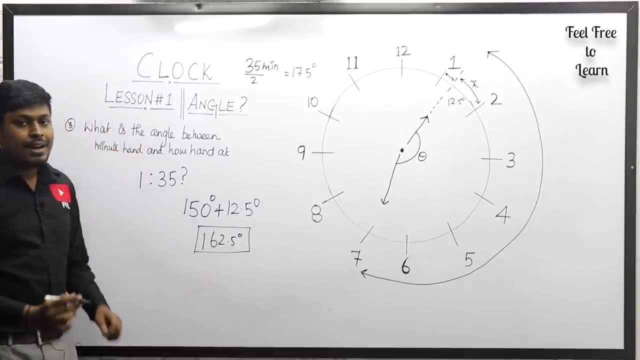 can say 150 degree plus 12.5 degree will be 162.5 degree. so finally we can say that angle between hour and and minute and at a time of 135 is 162.5 degree. understood, so it's completely i've written. 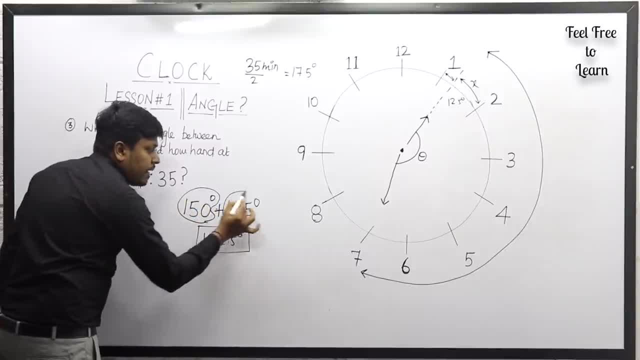 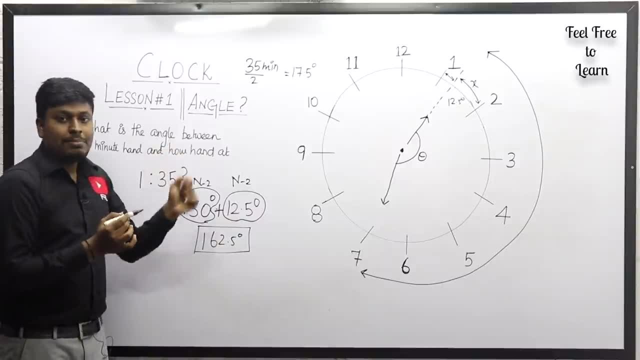 based on note number one what i said and this 12.5 i've written based on note two. so this is note one understood. so half the minute will be the degree that was traveled by the r hat. so once you understand both the notes clearly, then solving an entire question is easy understood. so this will. 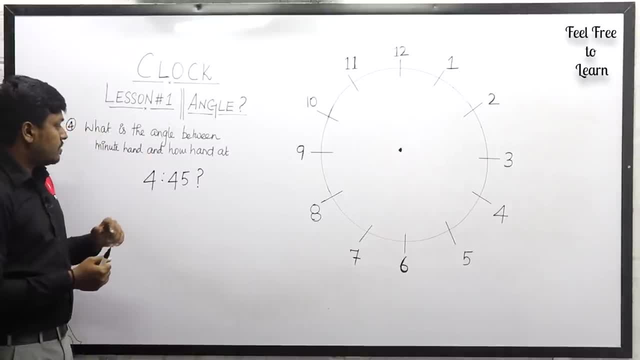 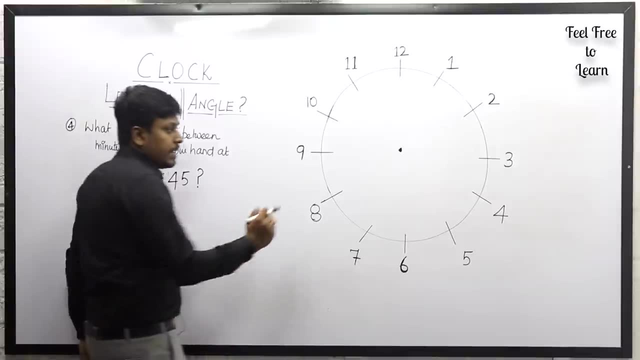 be the answer for question number three. question number four. so our target: to find what is the angle between hour and and a minute and at a time of 445. so let me draw a diagram here, so 445, where you can see the minute and will exactly points at number. 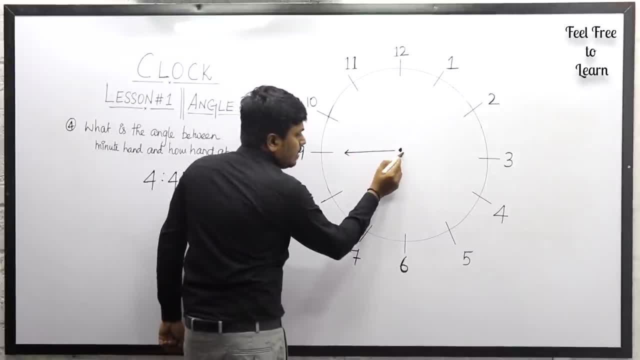 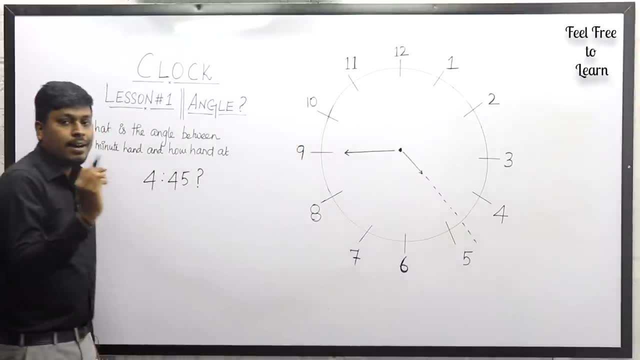 nine, but our and will not exactly at points at number four. it's somewhere between four to five, right? because only at four o'clock you can say the hour and will point exactly at number four. so here the time is 445, so definitely it will not points at four, somewhere between four to five. so 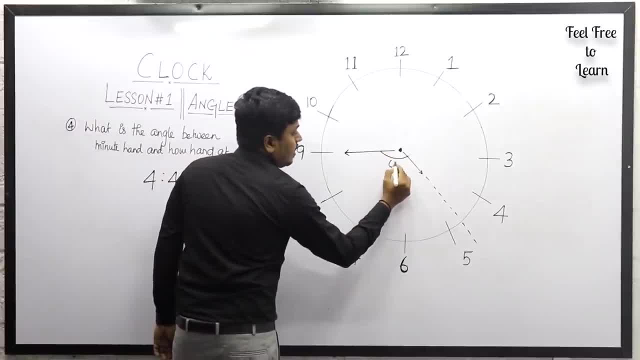 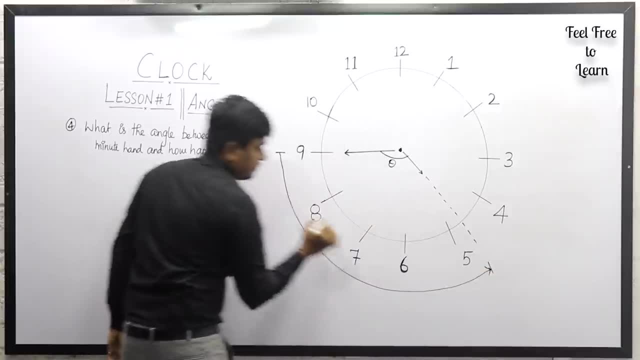 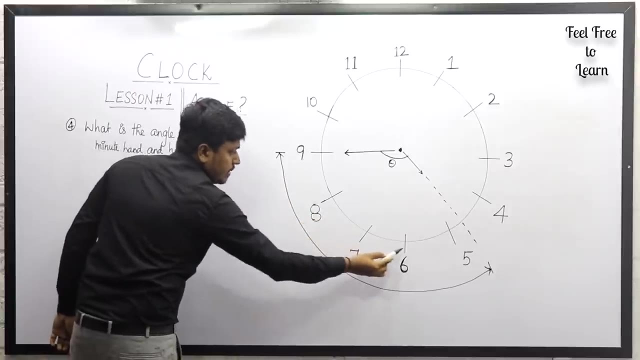 now our target to find what is the angle between hour and and a minute, and which means, from this point, right. so our target to find what is the angle till this. so just listen here, how many gaps are there? so, first gap: eight to nine, thirty degree, thirty degree, thirty degree and thirty. 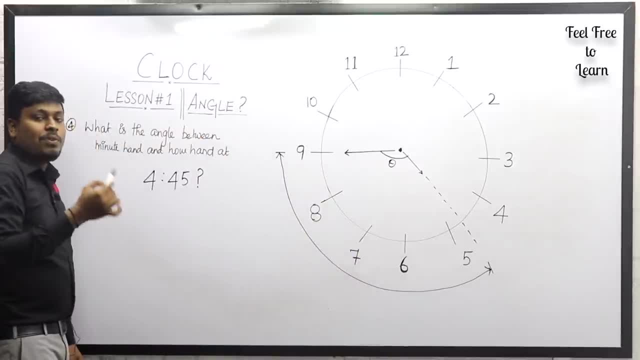 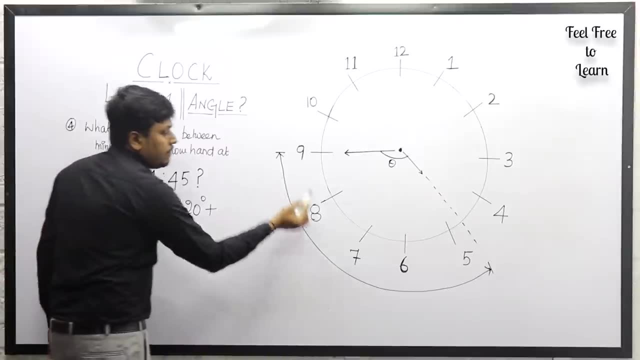 degree, so one, two, three, four, so four thirty degree. that is, four into thirty will be one twenty degree. so according to note number one i have written, each gap is thirty degree. so totally i have four gaps total. so we can say: four into thirty degree will be one twenty degree. and the next step: 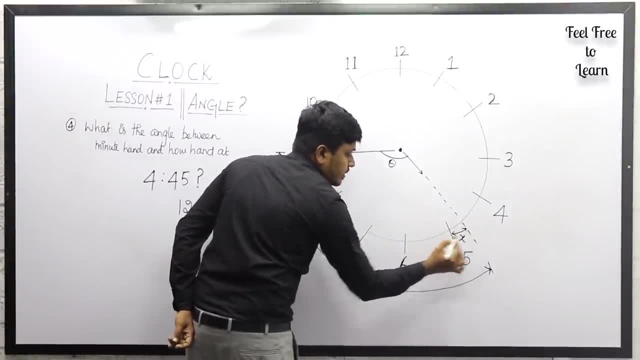 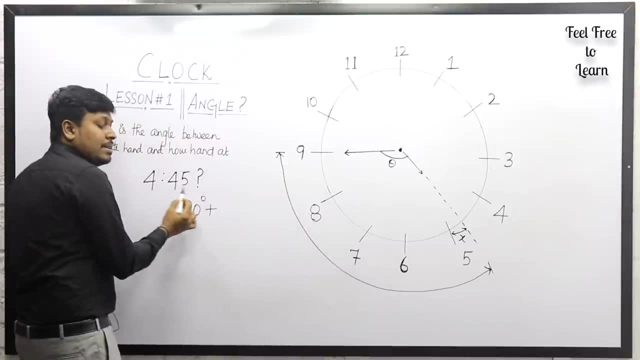 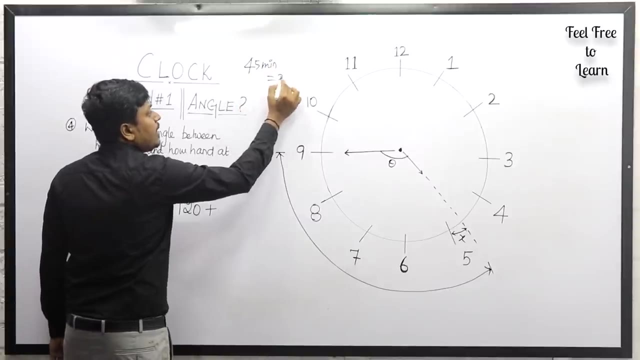 our target to find what is this remaining angle? so first we need to check how much this hour and moves from four. so for this what you need to do is how much the minute and most forty five minutes. so forty five minutes, so half the minute. so half the minute will be twenty two point five, so half. 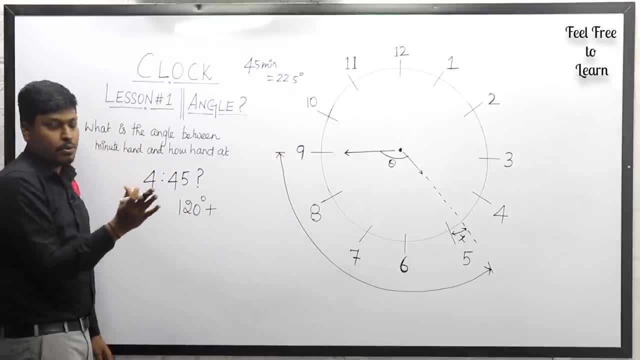 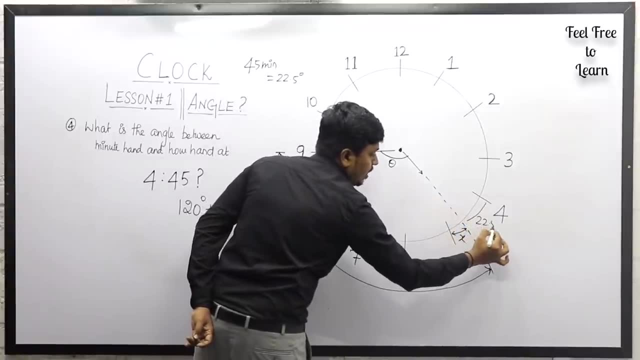 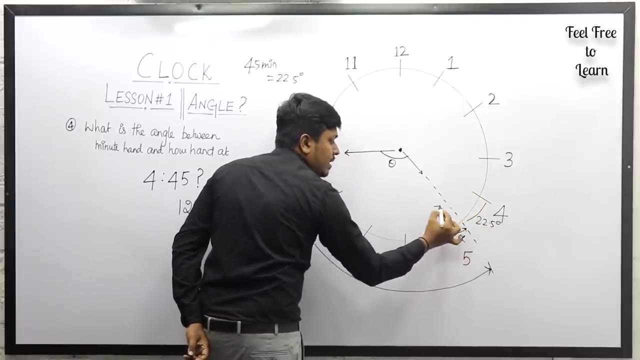 the minute will be the degree that was moved by the hour, and from four, so from four, it had travels 22.5 degree. So we can say this distance is 22.5 degree and the total gap is 30 degree. So total 30 degree minus 22.5 degree and the remaining will be 7.5.. So finally, we can say: 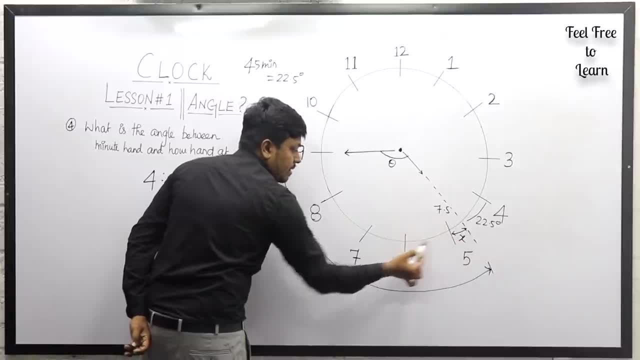 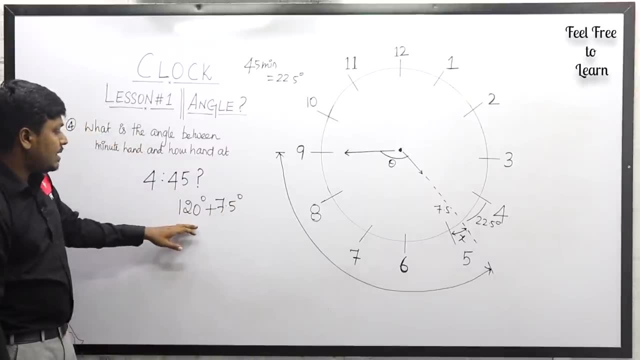 the value of x is 7.5.. So 7.5, 30,, 30,, 30,, 30. So we can say this: plus 7.5. So add all the values, So 120 plus 7.5 will be 127.5 degree. So finally we can say that angle between r and and a minute. 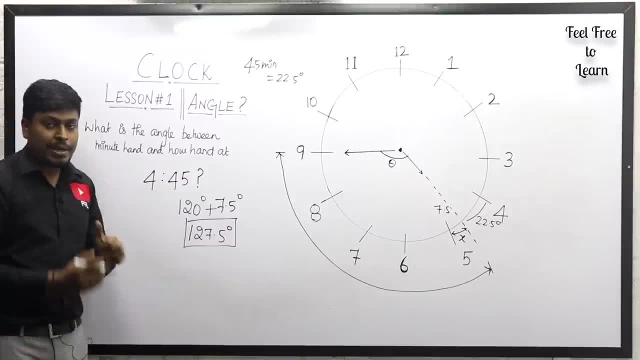 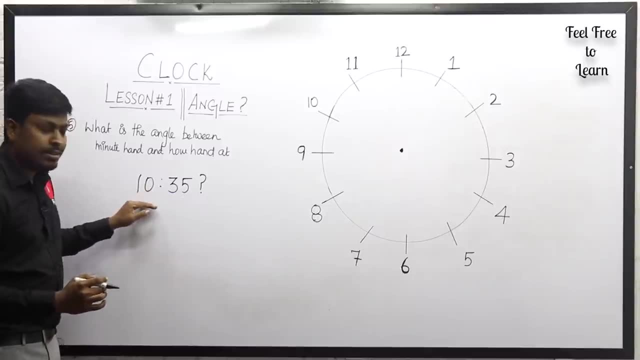 and at a time of 445 is 127.5 degree. Question number 5.. So our target to find what is the angle between r, and and a minute and at a time of 1035.. So 1035 where you can say the minute and. 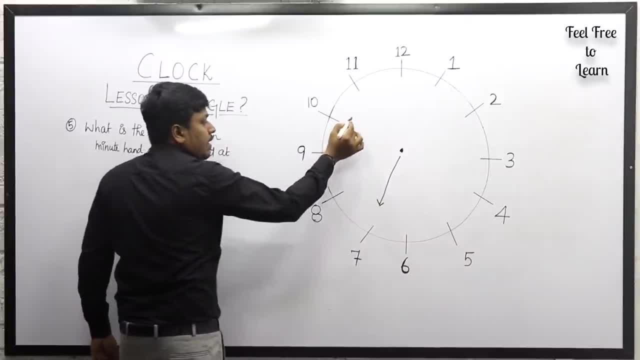 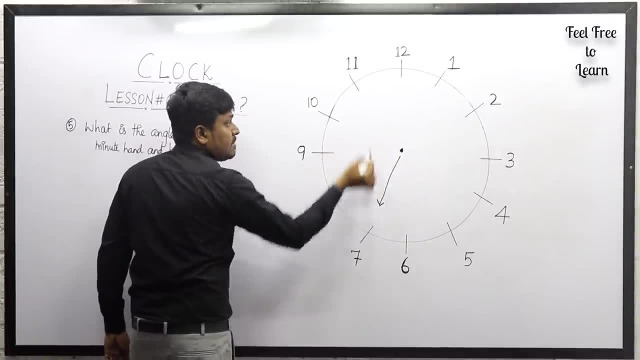 will exactly points at number 7.. And this r? and will be the angle between r and and a minute and will not exactly points at number 10, because only at 10 o'clock you can say r? and will points at 10.. So now the time is 1045.. So we can say it will be pointing somewhere between 10 to 11.. 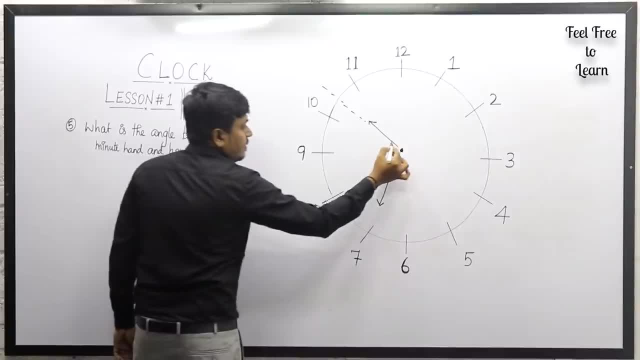 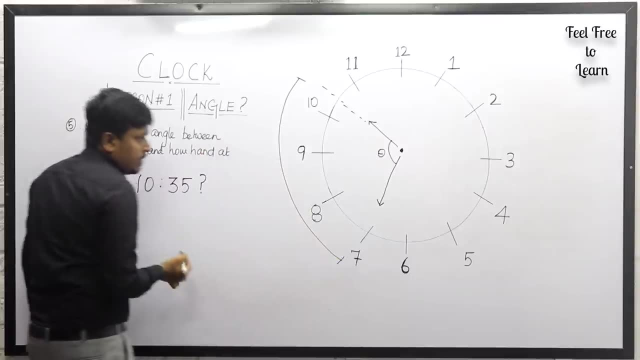 So our target to find what is this angle, So angle between r and and a minute, and which means from this point, our target to find what is this total angle, So according to note number 1.. So try to check how many gaps are there. So 8 to 7 is one gap 30 degree. So 8 to 7 is one gap 30. 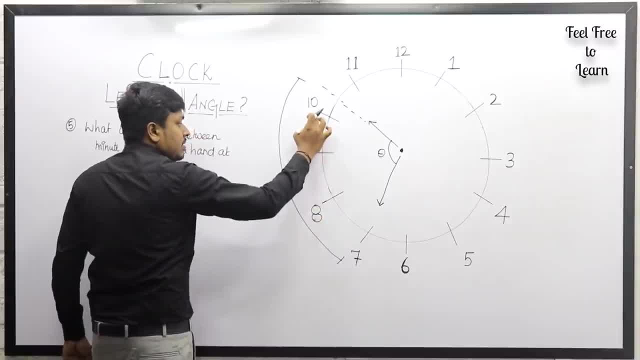 degree. So according to note number 1.. So try to check how many gaps are there. So 8 to 7 is one gap, 30 degree. 9 to 8 is another gap, 30 degree. So 10 to 9 is another gap: 30, 30, 30 will be 90. 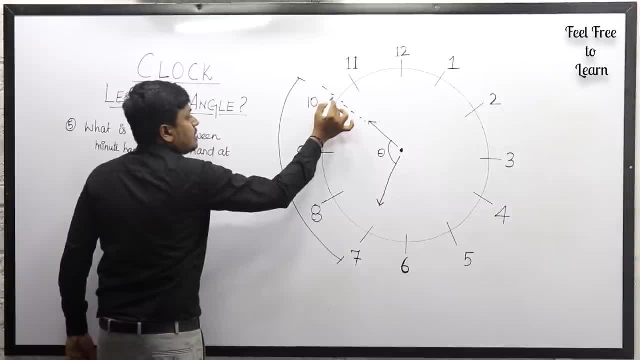 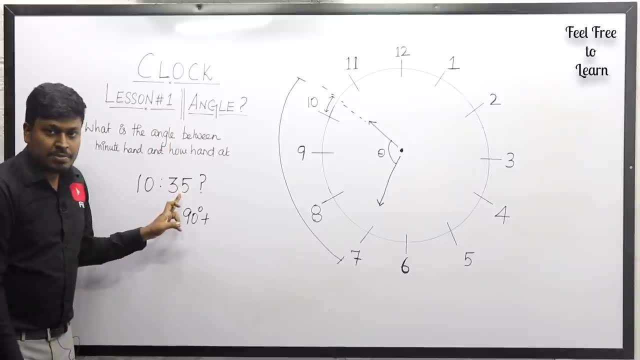 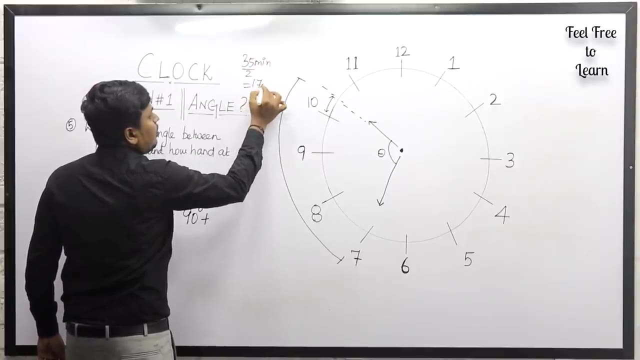 degree initially, So plus and the remaining last, this angle, Just see here we know that where the minute and travels how much minutes? 35 minutes. So from 0 it moves 35 minutes. So half the minute will be 17.5 degree, So this 17.5 degree will the time will be 20 minutes. So this is the time that 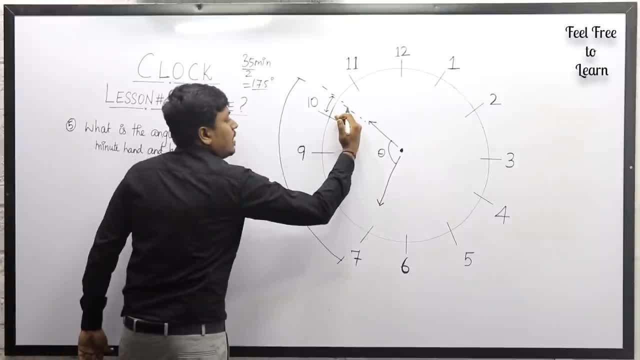 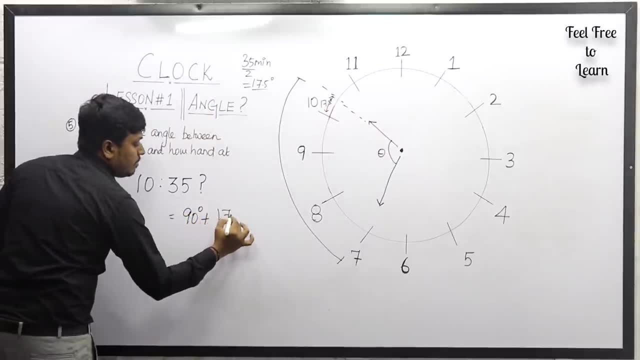 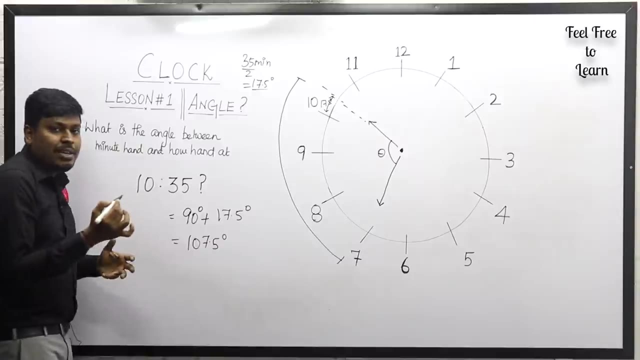 r and moves from 10, so from 10, where r and moves 17.5 degree. so we can say this distance is 17.5 degree, so at 17.5 degree, so resultant will be 107.5 degree. just listen carefully in all the. 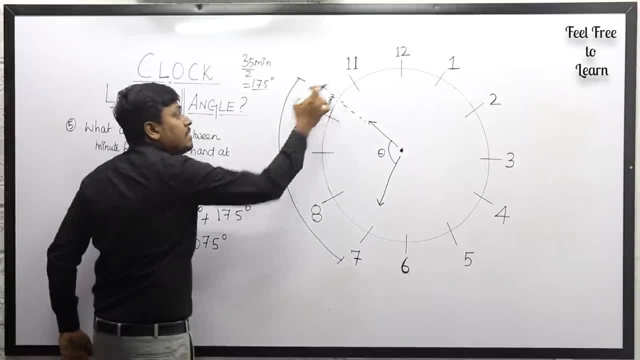 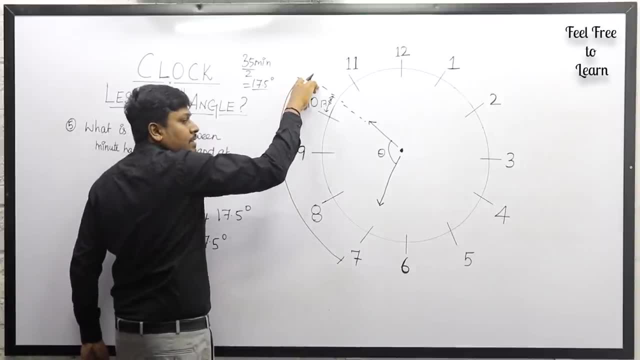 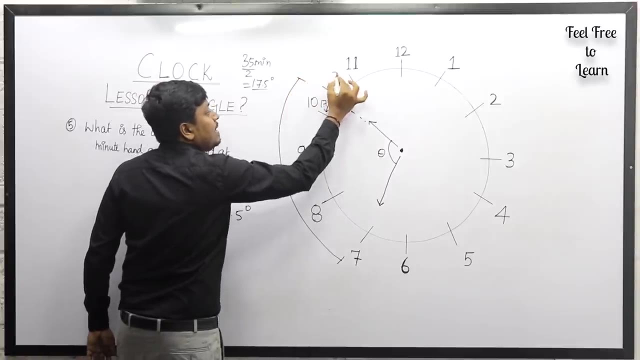 previous question, all the four question, i have subtracted with 30. why? because in this question i have not subtracted with 30? why? because our target to find only this angle, so i can easily find that half the minute will be the degree that was traveled by the r and in case, if i need this, 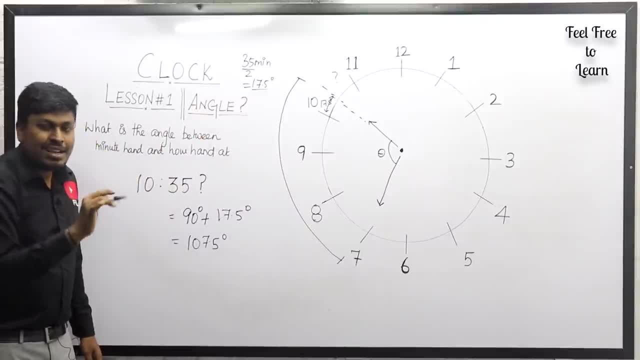 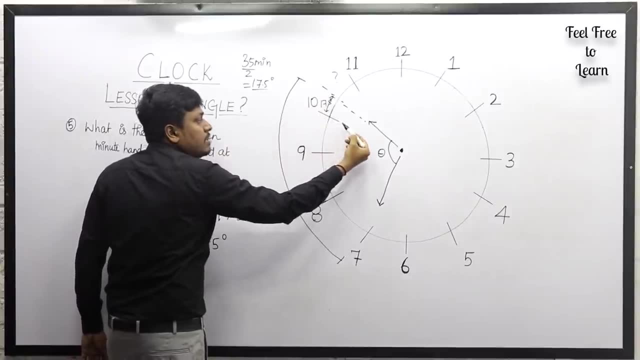 angle, i need to subtract with total 30 degree, but here i don't want to subtract with 30 degree because my target is to find this so directly. i'm getting a value that is from this point r and moves only 17.5 degree, so we can say this: 17.5 degree is a required angle, so we can say 17.5. 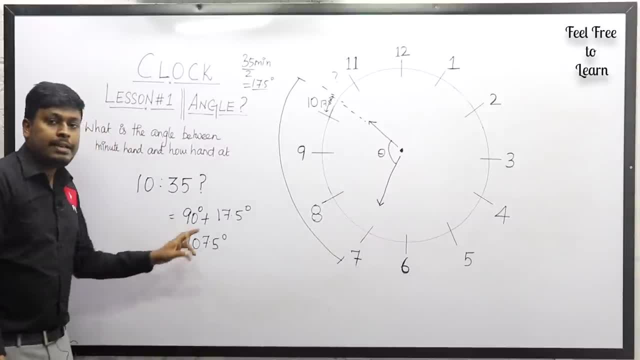 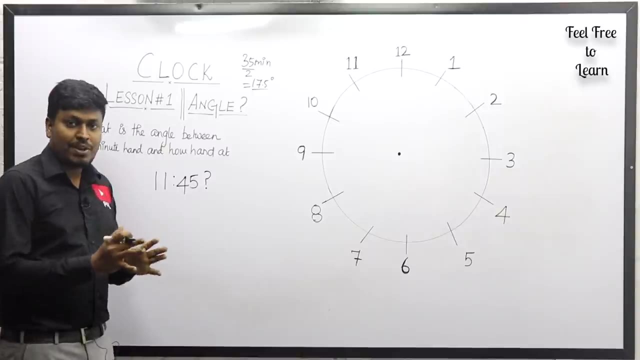 degree, 30 degree, 30 degree, 30 degree. so total 90 plus 17.5. so resultant will be 107.5 degree, understood. so answer for fifth equation is 107.5 degree at a time of 1035. so last sixth equation. so our target, to find what is the angle between: 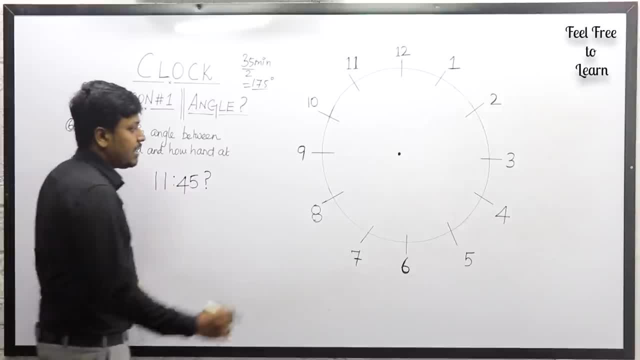 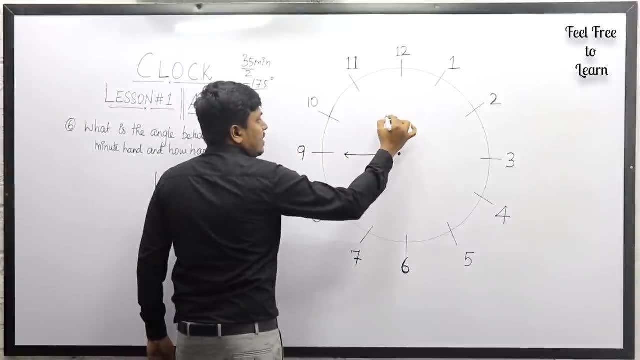 r, and and a minute and at a time of 1145, so we can say 1145, so minute and will exactly points at 9 and r and will not exactly points at 11. it points somewhere between 11 to 12, right? so what is our target? our target: to find this angle. so which means, from this point, our target? 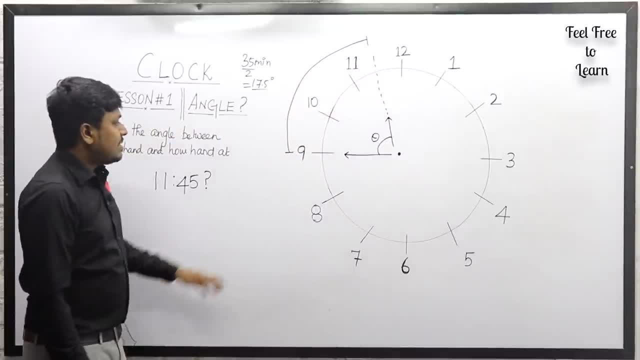 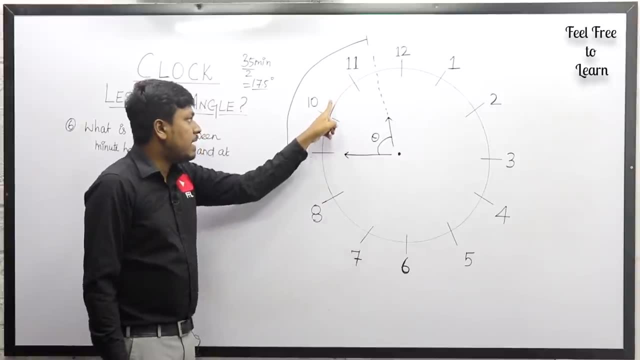 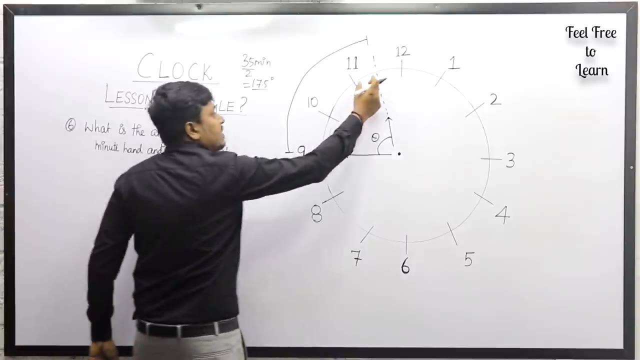 to find what is the total angle, right? so just listen carefully. we know that, according to note number one, the complete gap will be 30 degree, so this is 30 degree, and this will be another 30 degree, so 30 plus 30 degree will be 60 degree, so plus. and now our target: to find how. 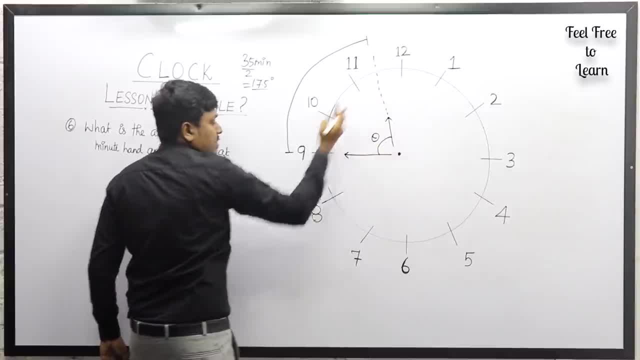 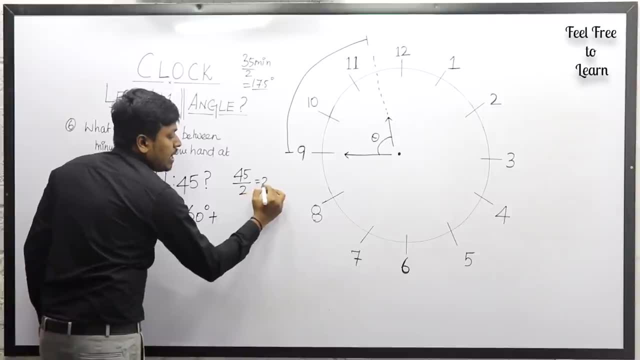 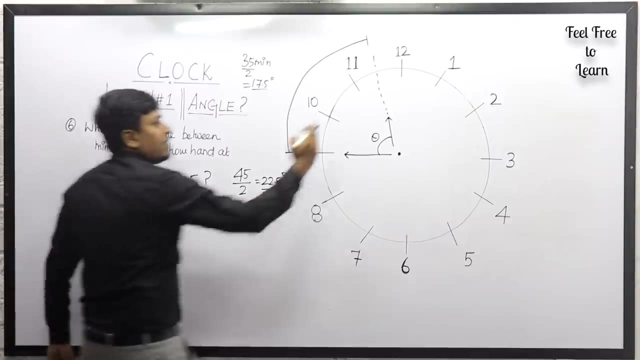 much degree the r and moves from this point to this point. so we can say where the minute and moves 45 minutes. so 45 minutes divided by 2 will be 22.5 degree. so 22.5 degree will the distance that was moved by the r and from 11, so from 11 it moves 22.5 degree. so we can say our. 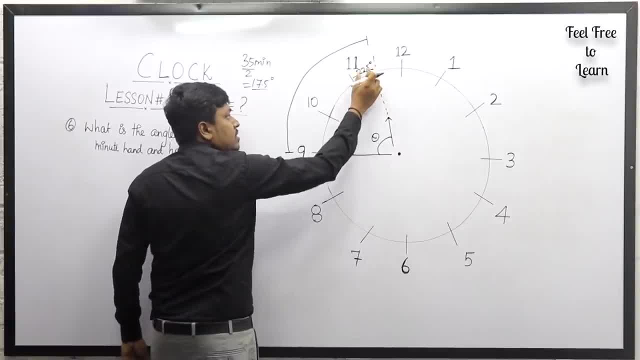 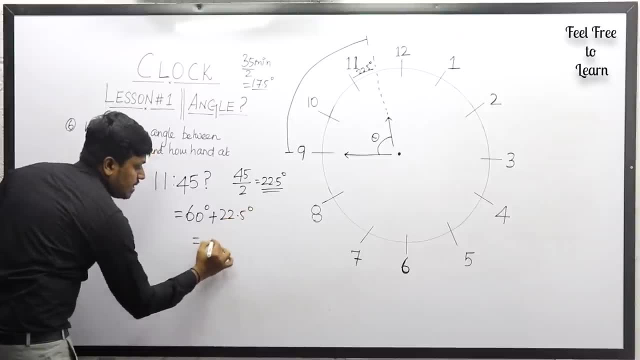 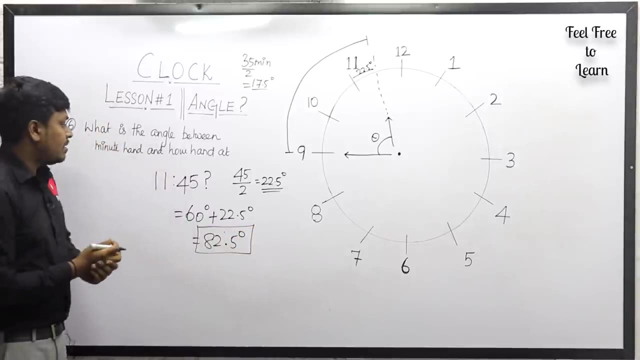 required target is this. so we do not want to subtract with 30 right. so 22.5 degree plus 30 degree plus 30 degree, so 60 plus 22.5 degree will be 82.5 degree. that's it. so this will be the answer for the last question, that is 1145. 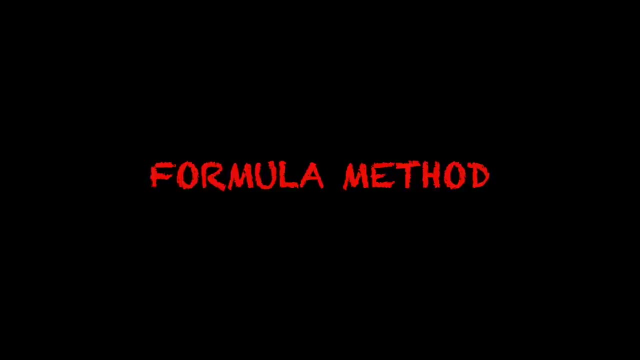 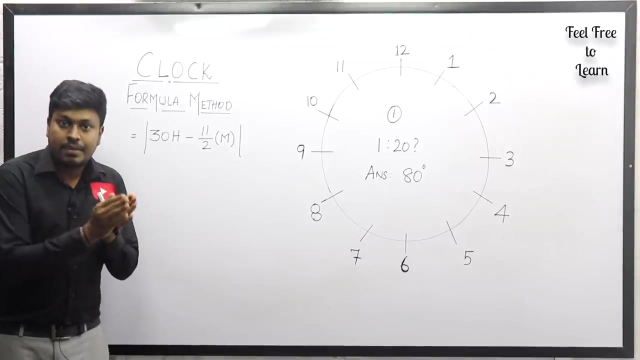 so now we can solve all the six question by a formula method. so in the beginning of this video itself, i have told you two things. every question can be solved by a formula method as well as by a traditional method, but remember that always you should know how to solve each and every question. 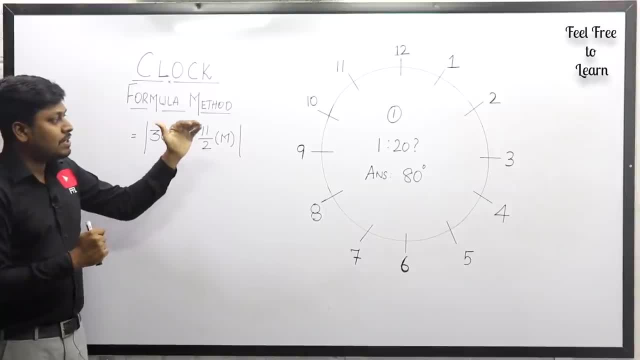 in a clock by a traditional method. right? so initially you should know how to solve each and every question in a clock by a traditional method, right? so initially we have learned all the six question how to solve in a normal traditional method. so now we can solve the same six question. 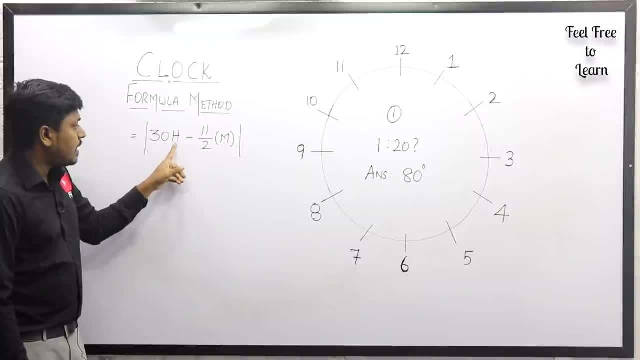 by a formula method. so this is the formula. so 30 h minus of 11 by 2 into m. so here h represent r and m represent 4 minutes. so this line indicates that in case if you are getting an answer in negative, we should always take it as a positive value, right? so just listen here. first equation: 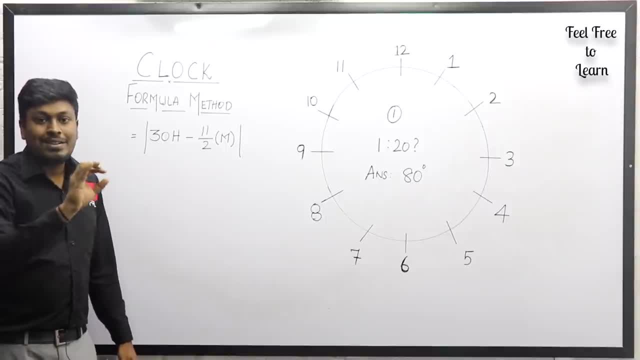 that we have solved in a traditional method is 30 h minus of 11 by 2 into m. so here h represents that is, in order to find what is the angle between r and and minute and for the time of 120, and we got an answer: 80 degree. so now what you need to do is just substitute all the values in 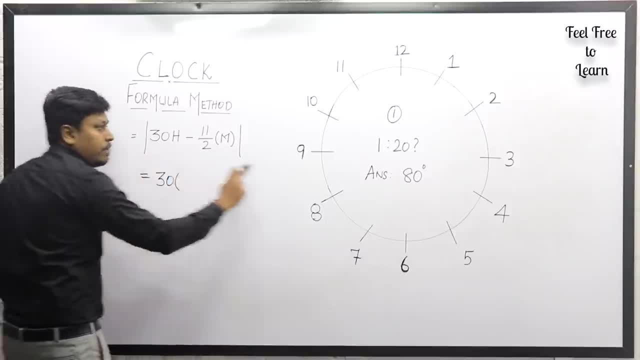 a formula. so 30 h represent r, right, how many are here? 1 r, so 30 into 1. minus of 11 by 2 m is 4 minutes. so how many minutes? 20 minutes. that's it. you can directly substitute the value for r and minute. you will get the answer right. if you cancel one, twos are two. 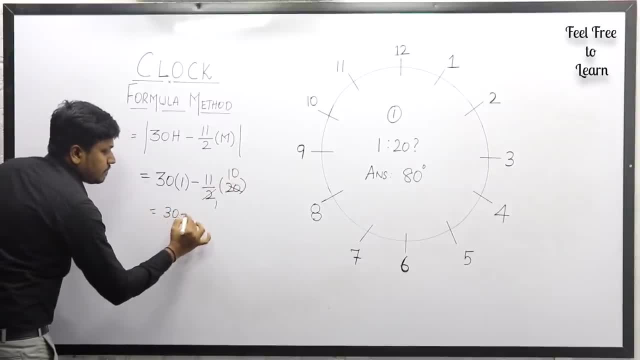 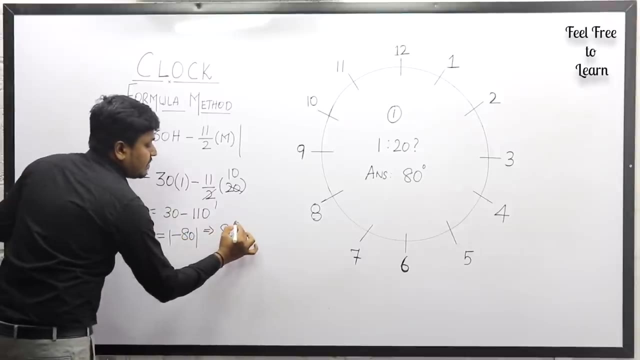 times here. so 30 into 1 will be 30. under 11 into 10 will be 110. so we are getting an answer as minus 80. just know i have told you these two line indicates that even if we are getting a negative value, we should take it as a positive. so answer for this first equation, that is, angle between: 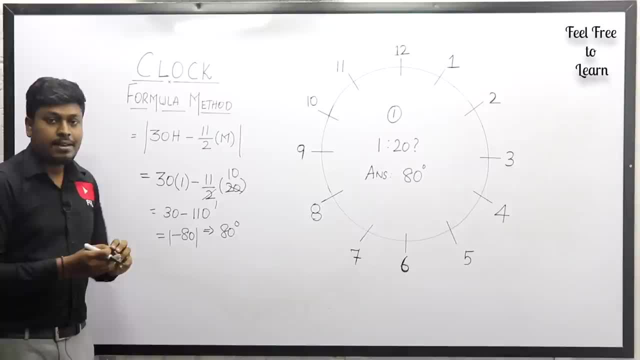 r and and a minute and at a time of 120 is 80 degree. understood. it's easy or not very easy, right? so finally, we got an answer that is 80 degree. just listen here. don't forget to watch the complete video, right? there are some exceptional cases where you should. 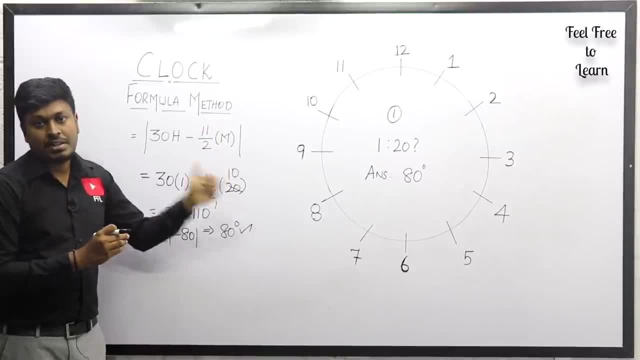 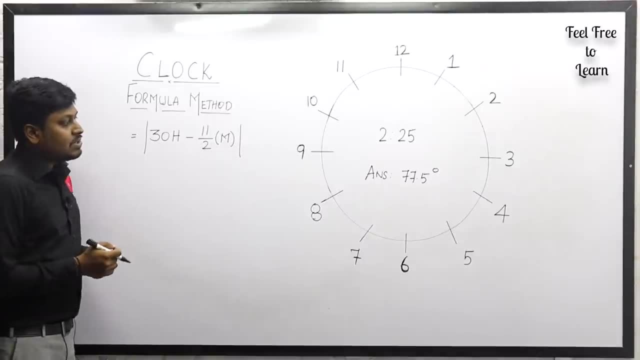 not make a mistake. so initially i will solve all the six questions in a formula method. so finally, answer for first equation by a formula method is 80 degree. so second question, that is 225 and we got an answer as 77.5 degree. so here in a formula method. so 30 into h. so h here to us. 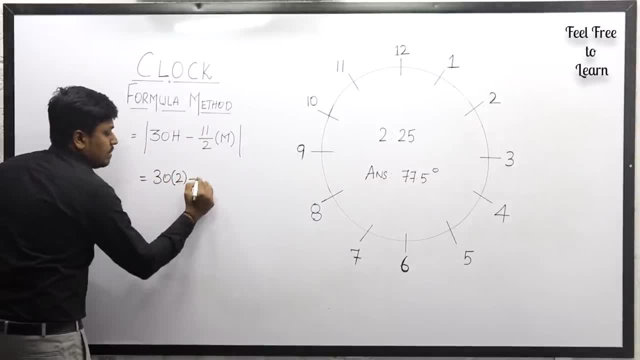 so for instead of h we need to write 2 here, so minus of 11 by 2. and instead of minute, here you can see 25 minutes. so instead of m, right, 25 here is equals to 60 minus of. just listen here. either you can cancel 225 as 12.5, or else you can multiply both the numbers and finally divide by 2: it's your. 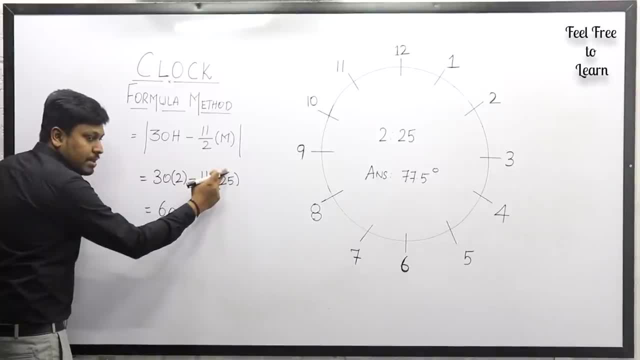 wish, right? so what i'm going to do is i'm going going to multiply both the numbers after getting an answer. i'm going to divide by 2, so this will be 5 7- 2, so 275 divided by 2. so 60 minus 1, 2s are. 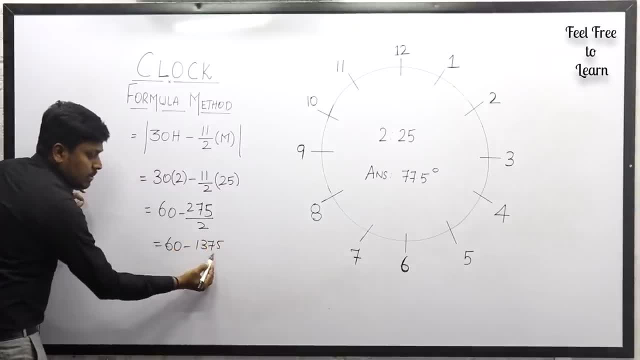 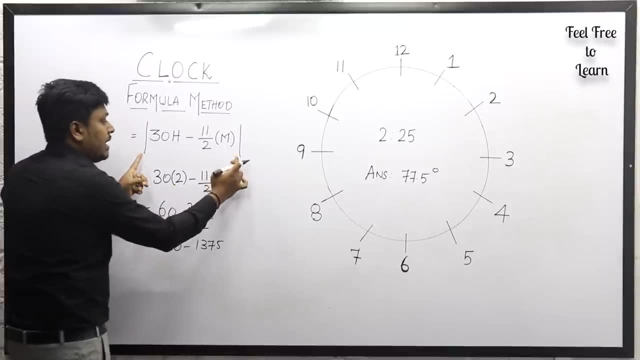 2, 3, 2s are 6, 7, 2s are 14. 0.5. so 60 minus 137.5 will be 77.5 minus 77.5. just now i have told you these two line indicates: 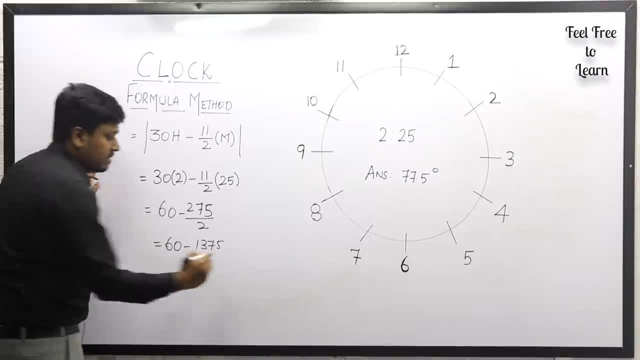 that even if you get an answer negative, we should take it as a positive value. so answer will be 77.5 degree. so this will be the answer for question number 2 in a formula method. here is the last question that we solved in a traditional method, so try to solve the remaining questions right. 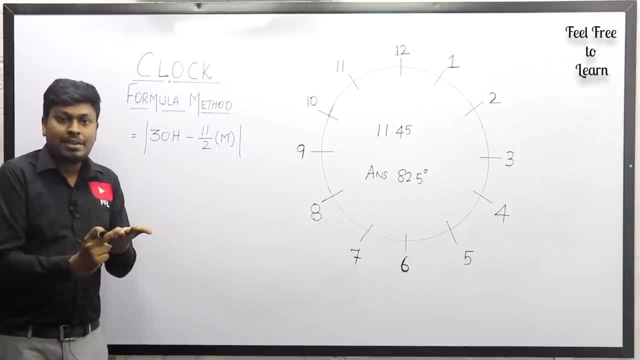 three, third question remaining. fourth question remaining. fifth question remaining, so 211.. try to solve all this, all those numbers, by a formula method. right, i'm just going to solve another, only one question here. the last equation is 11 is to 45, so for that in a traditional method. 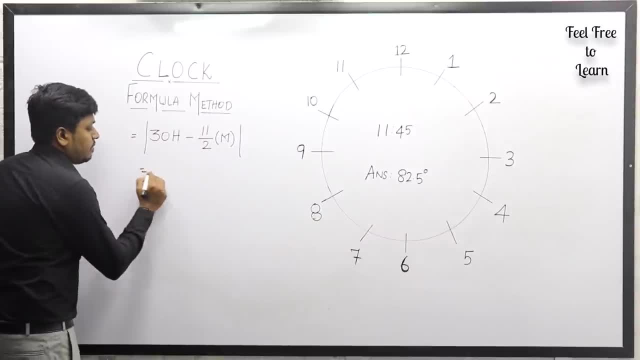 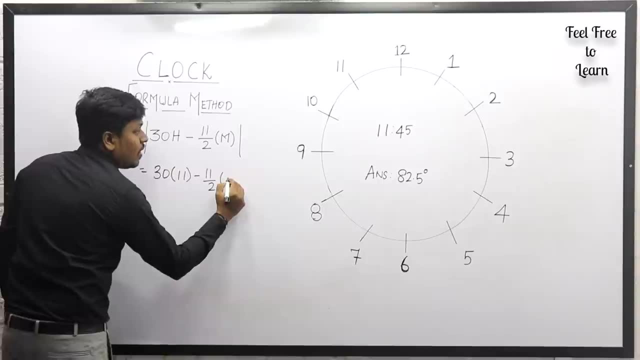 we got an answer 82.5. so now substitute in a formula: so 30 into h, so for h, 11 as minus of 11 by 2 for a minute. we got 45 minutes right, so 30 into 11 will be 330. so minus of 11 into 45. so 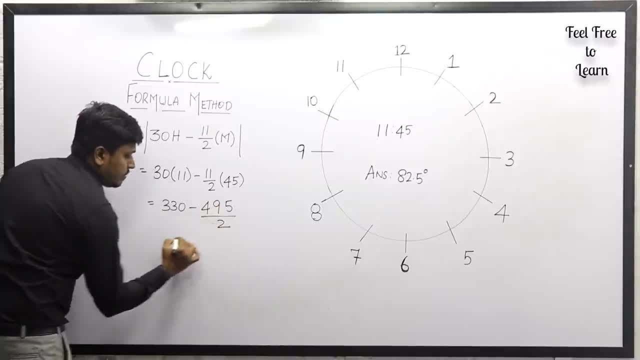 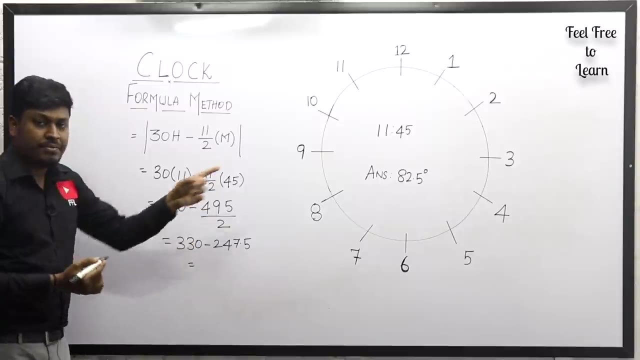 this will be 5, 9, 4, 95 divided by 2, so 330 minus of. so. 2, 2s are 4, 4, 2s are 8, so remaining will be 1, 7, 2s are 14.5. so if you subtract 2 330 minus 247.5, you will get 82.5. so this will be the. 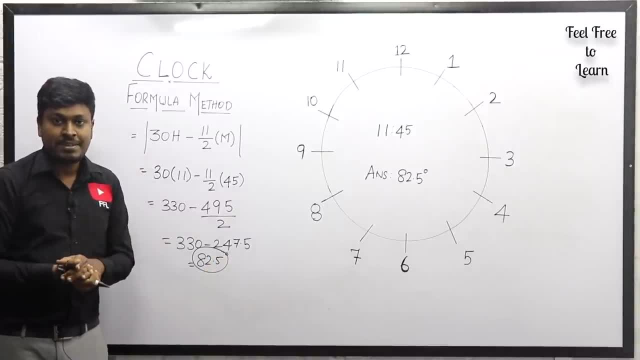 answer for the last sixth question in a formula method. right, so just listen here you can, you can. you can solve in case in the exams if they ask what is the angle between r and and a minute, and you can always go with the formula method, no problem, because we are getting an answer correctly. 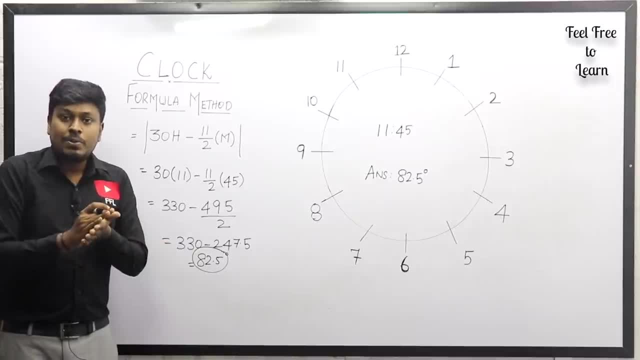 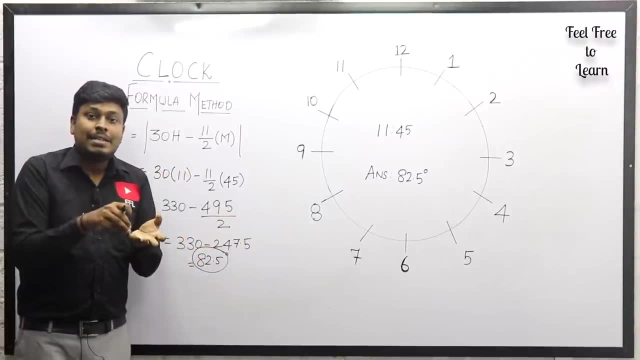 so we can go with the formula method always. and also, you have learned the traditional method. yes, from the beginning i have taught you what is a traditional method. so if you learn the traditional method for solving third lesson in clock, fourth lesson in clock will be very easy for you. so 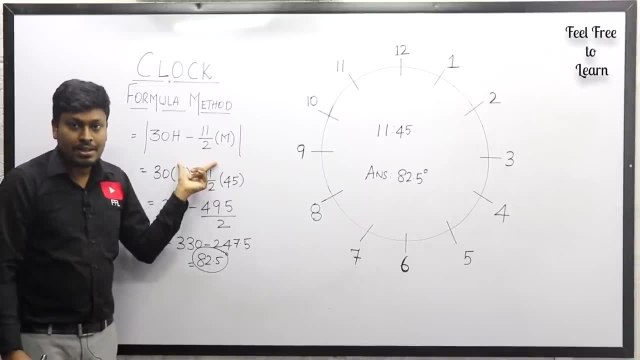 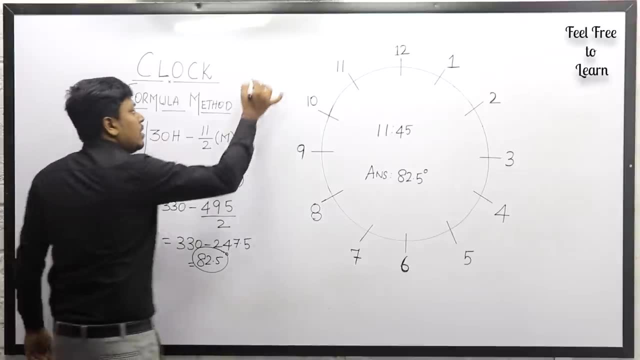 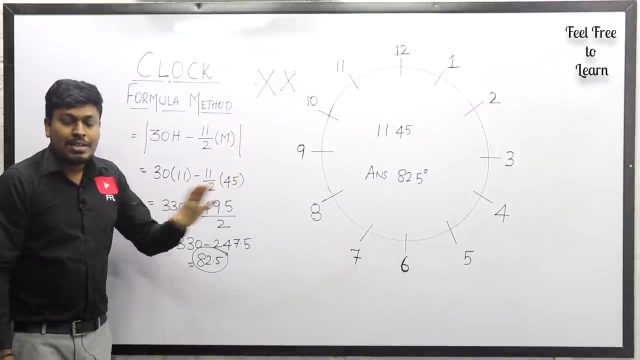 students, those who learn only the formula method without knowing the logic. they can't able to solve the medium and high level question in the exams. so next important thing in the video is most, most most important concept where many students will make a mistake. just see here: what i'm going to teach you now is most important in the topic clock. so never forget this, take it as a proper note, or else you will surely make a mistake in the exams, right? so now let me move on to the one of the most important note in the clock. so let me take one timing as 12.5.. 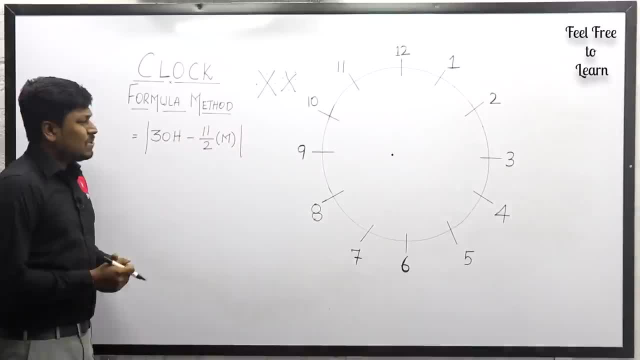 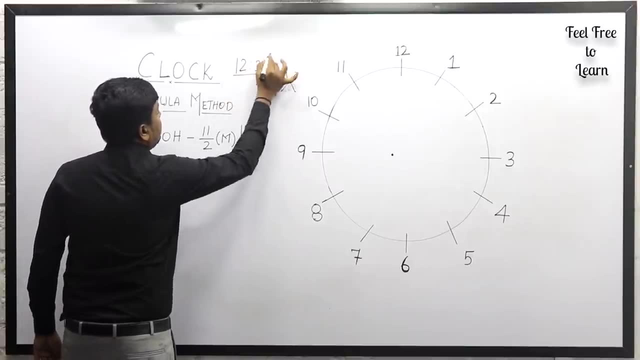 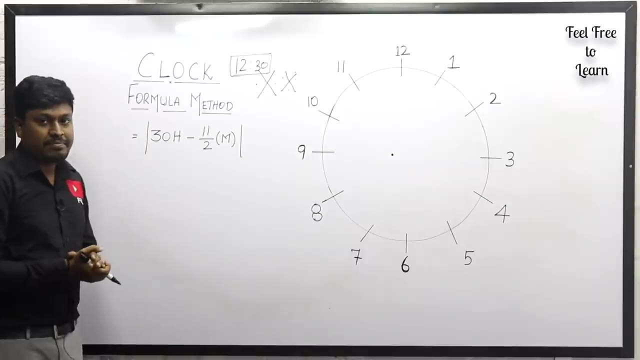 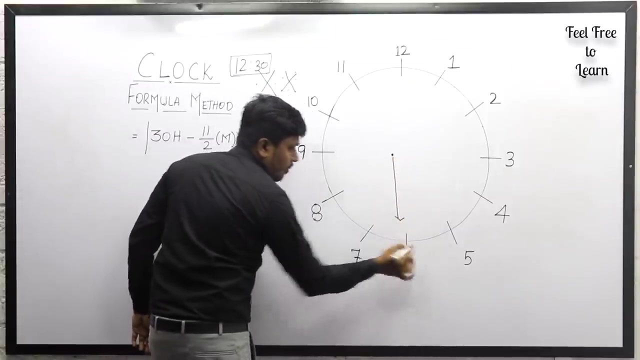 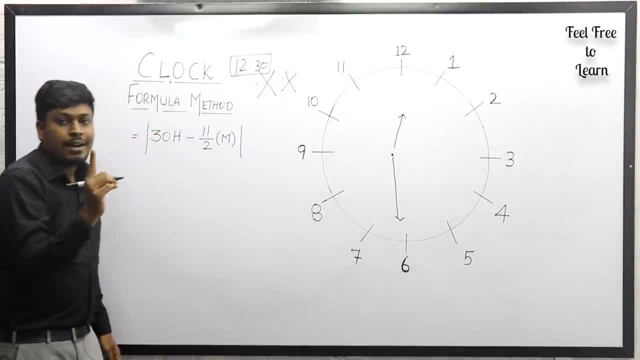 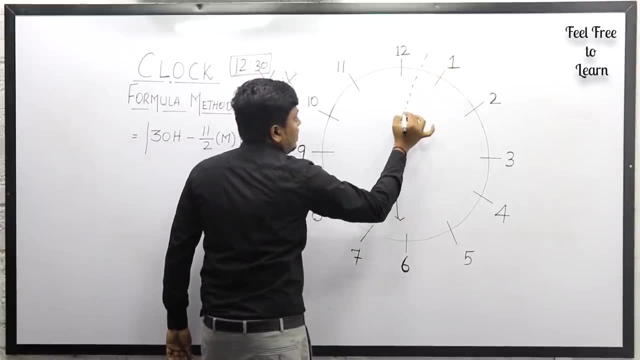 because only at the time of 12 o'clock, where the Rn will points exactly at 12 because of 12.30, it will be somewhere between 12 to 1, right? so now our target: to find what is the angle between Rn and the minute. 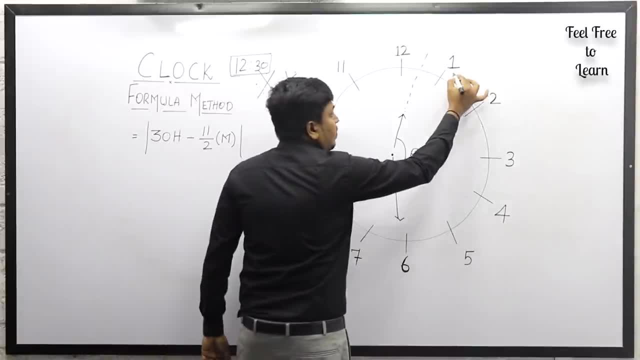 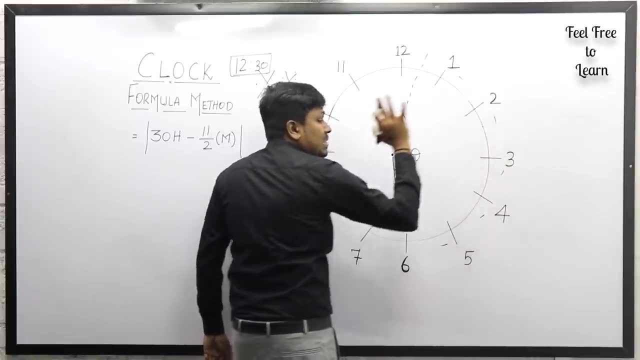 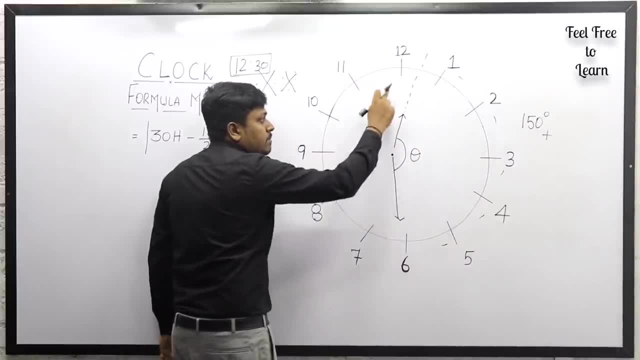 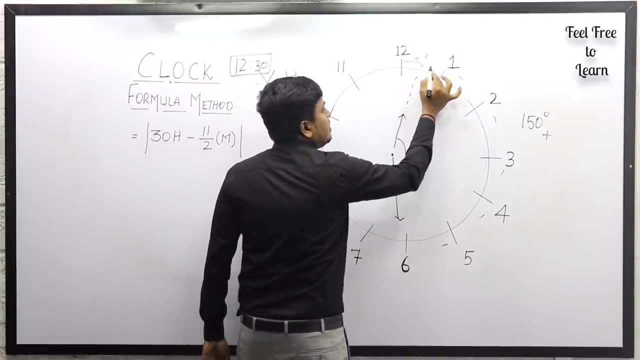 so plus- and here you can see the minute and moves, 30 minutes. so 30 minutes divided by 2 will be 15. so we can say this angle is 15 degree, so this will be remaining 15 degree. so 30, 30, 30, 30, 30 plus 15. 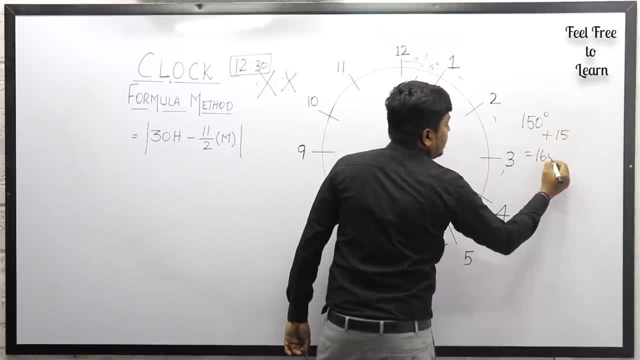 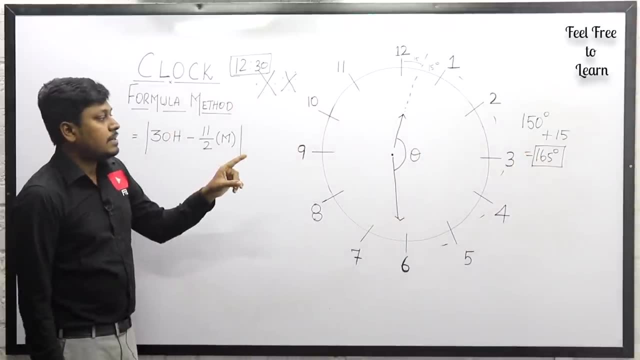 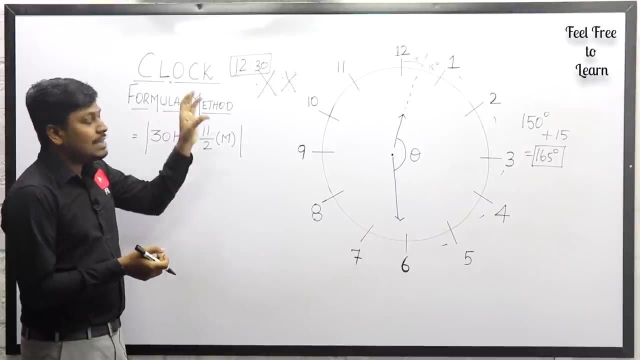 so add 15 here, so resultant will be 165 degree. so just listen carefully. in a normal traditional method in a clock we got a answer that is for angle between Rn and a minute and is 165 degree. so now we can solve the same question in a formula method. just see here. 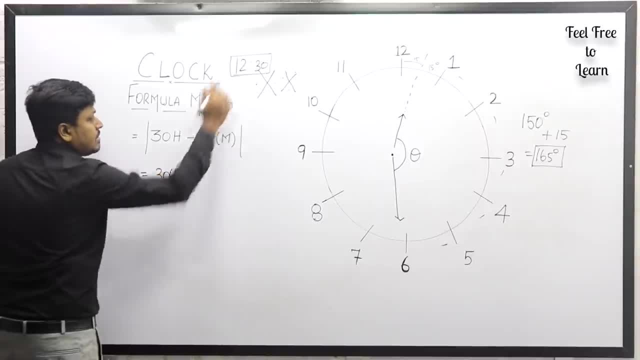 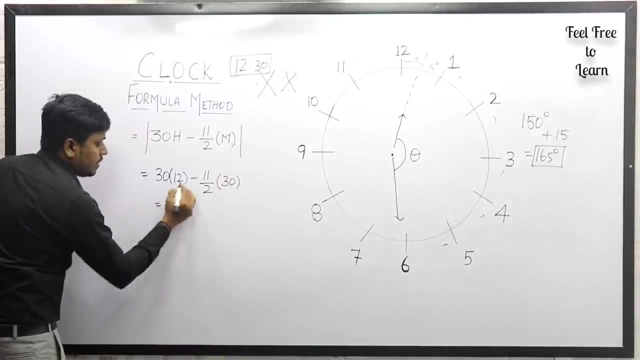 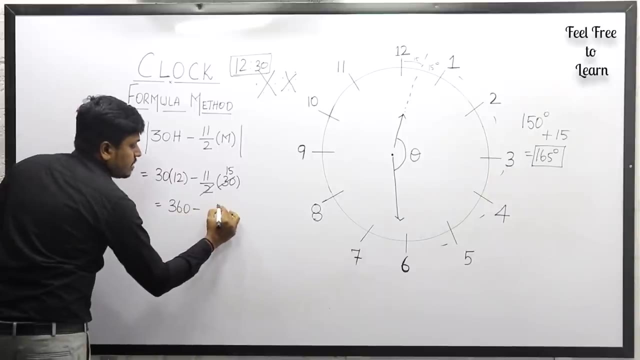 so 30 into R. so for R we can say: 12 minus of 11 by 2 minute will be 30, so cancel it. 12 into 2 will be 360, so minus of its even number, so better. we can cancel it. so 5 times, 6 times, 1 times. 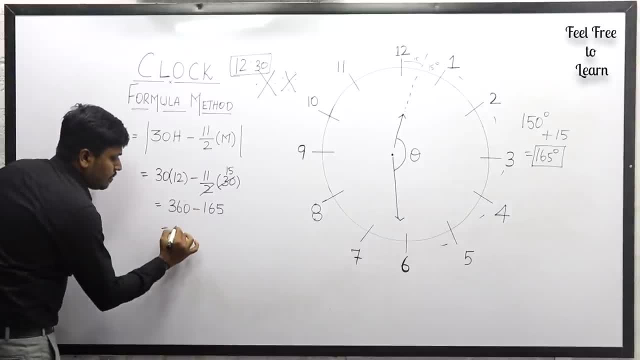 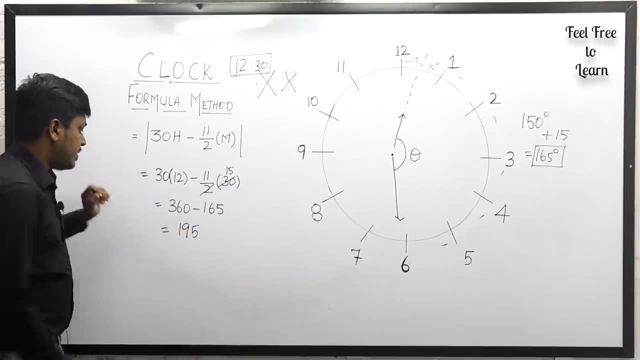 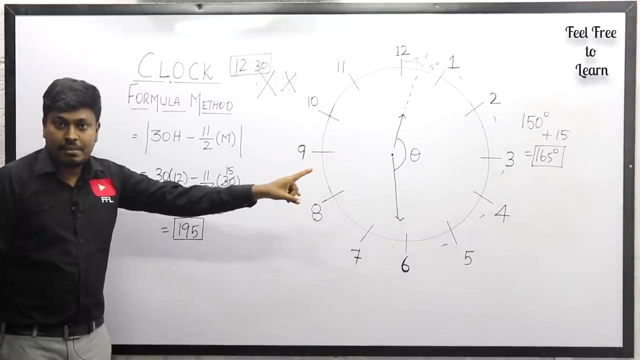 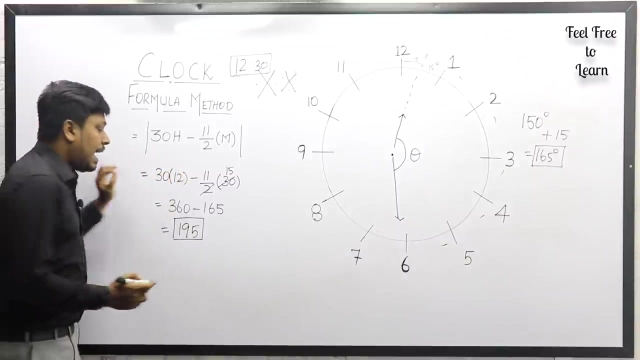 so 360 minus 165 will be 195. things was so: 195, 950, 60, 195. just listen carefully. while solving a question in a normal traditional method, I got an answer as 165. the same question if I solve in a formula method, I'm getting an answer as 195. whether I should go with the traditional method. 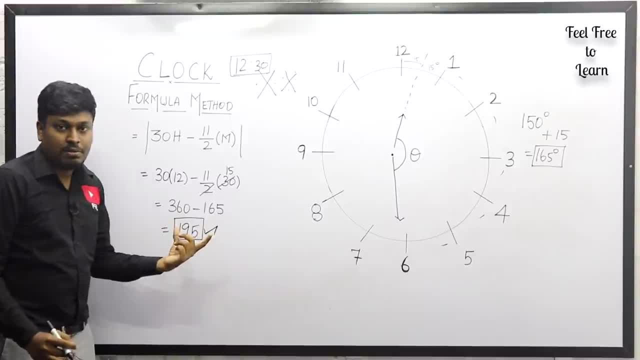 always, or I should go with the formula method, always. this was the major doubt of a student, even for my friends. they usually ask this doubt in case, in the option, if I have 165. in the option, if I have 195, what should I mark? just listen carefully, friends. in the clock there are two angles right. 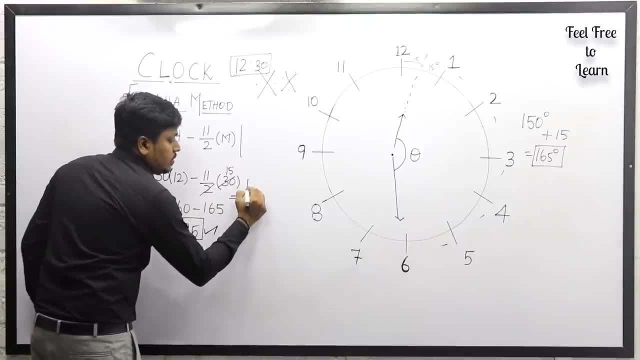 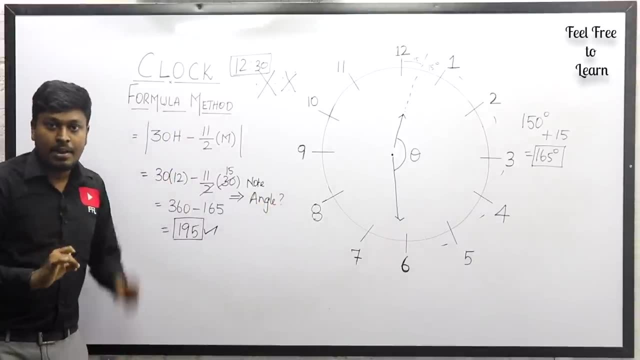 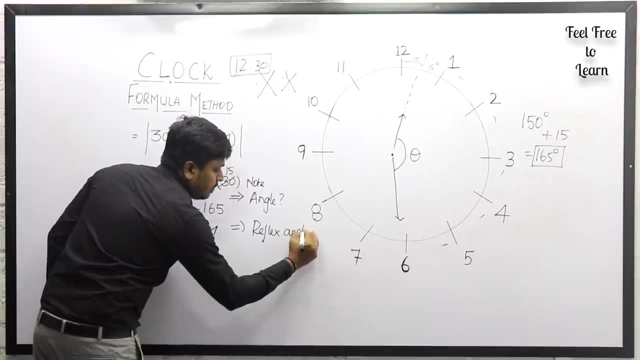 usually the question will ask you like note one, only to find the angle. just find the angle between Rn and a minute, and that's it one based question. and the second based logic question is find the reflex angle. the same question can be asked like: find the. 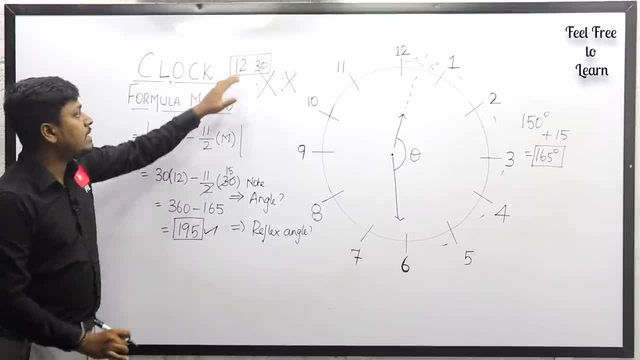 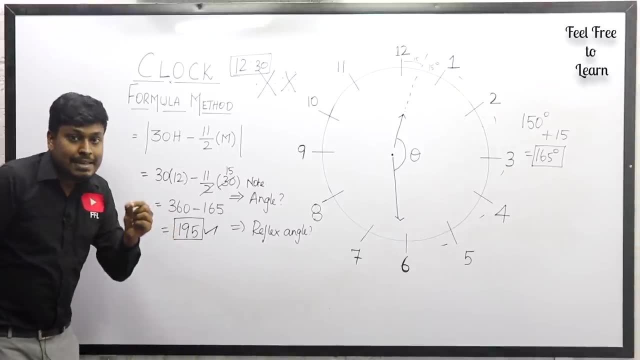 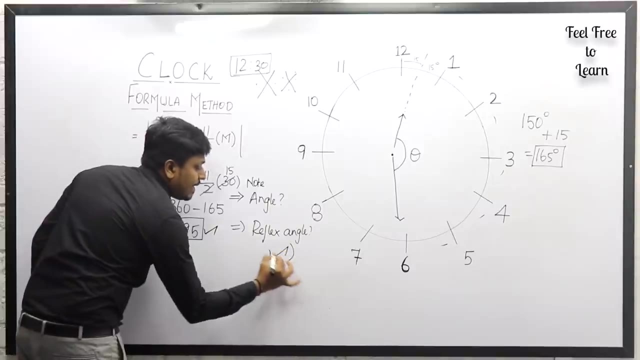 reflex angle for an Rn and a minute and at a time of 1230. just listen carefully. if you are getting an answer more than 180, like more than 180. if you got an answer more than 180, then it is called as a reflex angle, not the angle between Rn and a minute. 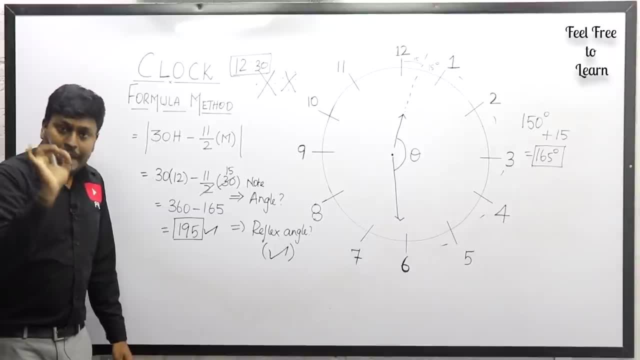 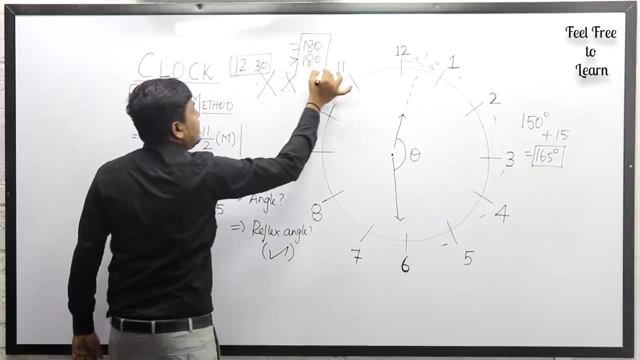 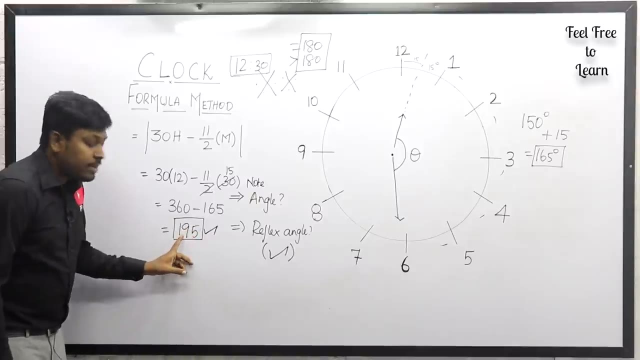 and only if you get an answer equal to 180 or less than 180, then only we can say: it will be the answer for angle between Rn and a minute. and so, friends, understood. here you are getting in a formula, method 195, there you are getting in a traditional method 165. but if you only follow the 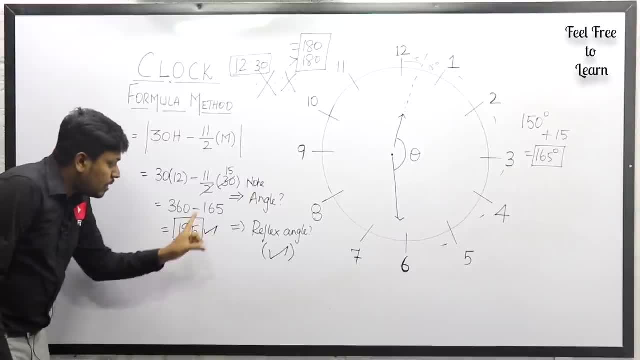 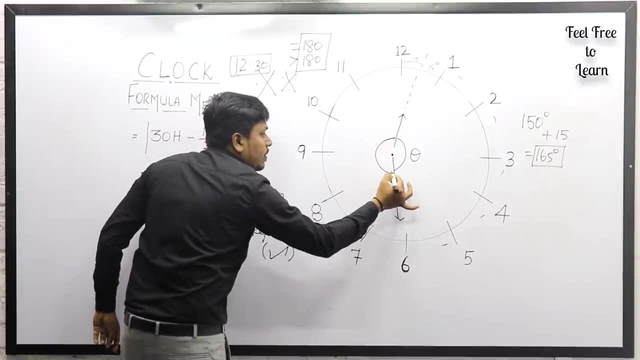 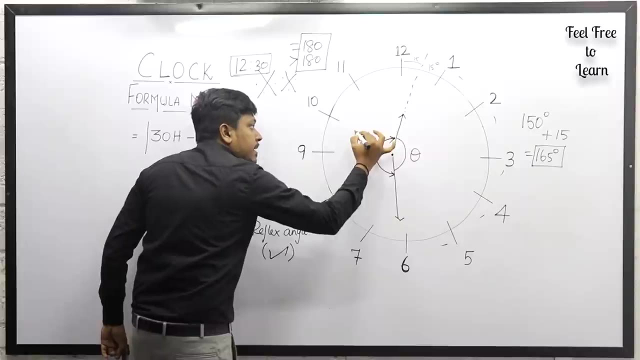 formula method. what you need to do is you should not mark the answer as 195 in the exam, because this 195 is the angle for it. we found this angle 195 in a formula, but our target- to find only this, why I am not marking the answer in the exam- is: 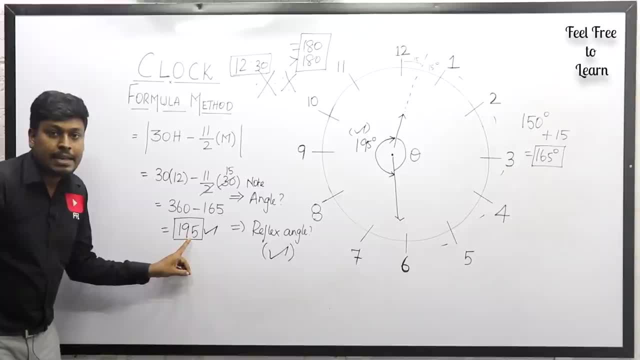 because I am getting an answer more than 180. if it is more than 180, then we should not mark the answer. so what you need to do is you need to subtract with 360. so 360 minus 195, the resultant will be 165. so this will be the angle between Rn and a minute and at a time of 1230. 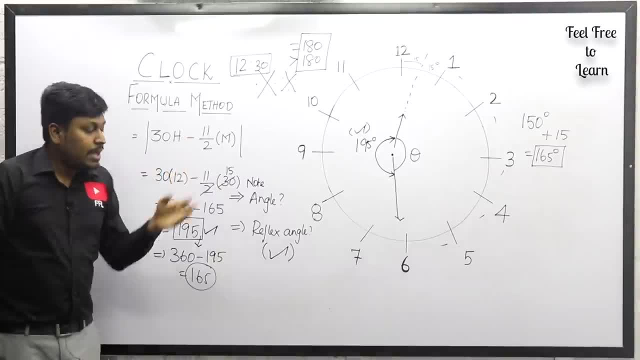 so in all the previous question that we solved, we directly got the answer, but some scenarios we won't get the answer in a formula method. why? because we are getting an answer that is more than 180. if we got a number more than 180, then it is not the angle between Rn and a minute and 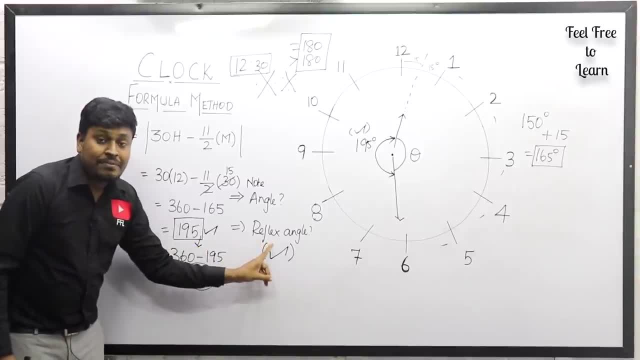 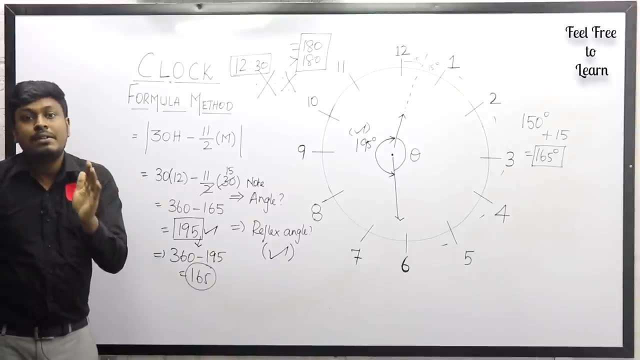 it is called as a reflex angle. so reflex angle is called. reflex. angle is nothing, but if you find an angle more than 180 degree or less than 360 degree, it is called as a reflex angle. so, in case, if you get an answer more than 180, what you need to do is you need to subtract with 360. 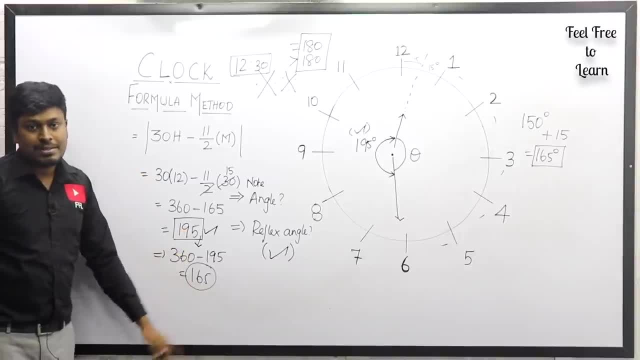 so 360 minus 195 resultant will be 165. so finally you can say, even in a formula method you will get a correct answer: 165. that's it got the logic. or else I can solve another one example question so that you can easily able to understand the question. 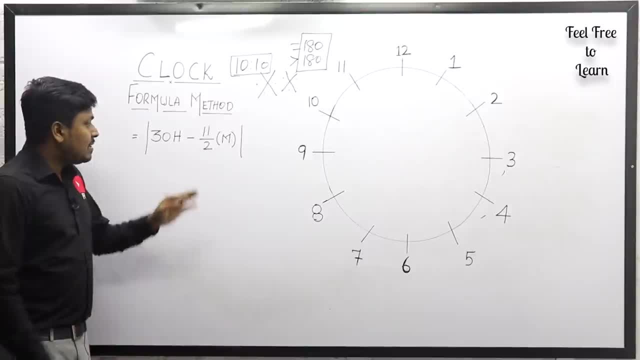 so let me take an another important example question. so our target to find what is the angle between Rn and a minute and at a time of 1010, just listen here. let me initially go with the traditional method. so traditional method, where you can see the minute and will exactly points at number 2. 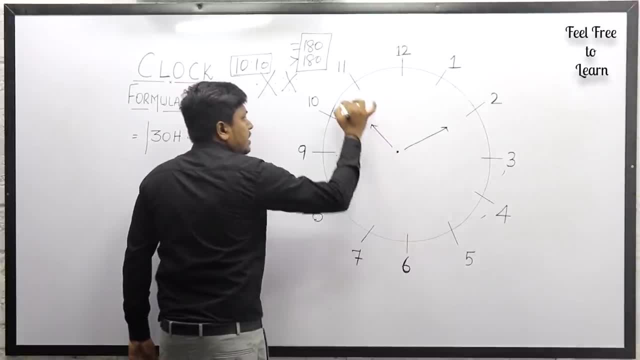 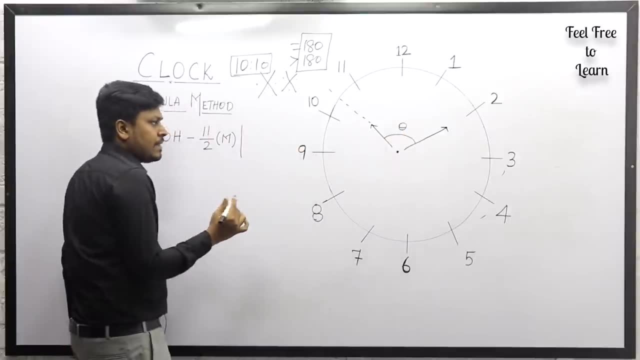 but this Rn will not exactly points at number 10. it will be somewhere between 10 to 11. so our target- to find what is the angle between Rn and a minute and so what usually we will do in a table- is that what traditional method is? we will check the gap. 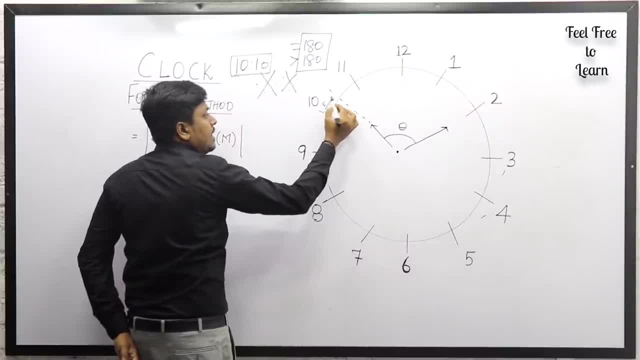 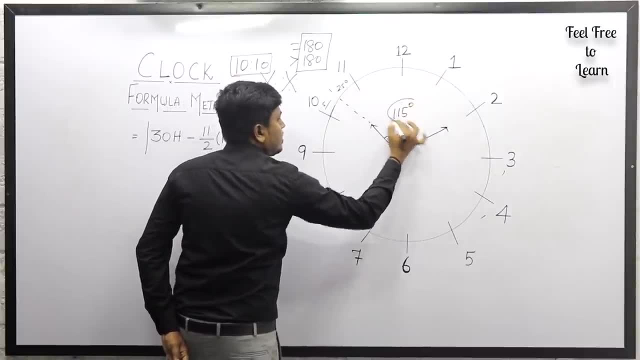 so 30, 30, 30, 90, so this will be 5 degree. so this will be 25 degree. so 25 plus 30 plus 30 plus 30 will be 115 degree. so this is the way we found the answer in a normal traditional method. 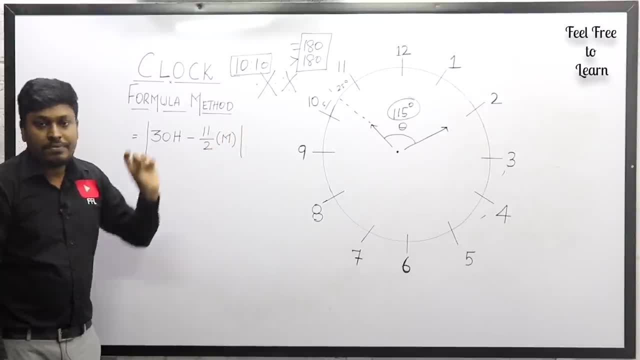 so I would say the answer for this question is: 115 degree is the angle between Rn and a minute. and so now let me move on to the formula method. see here: so 30 into H, so here H is 14, now 10 as minus 11 by 2 minute. 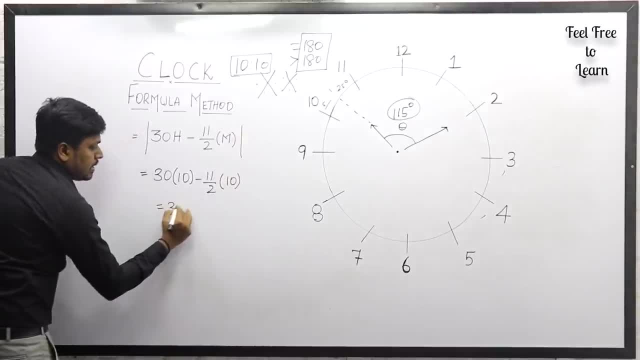 so minute will be another 10, so 300 minus of cancel this 5 times its 55, so 245. just see here, in a formula method, right in a formula method, I am getting an answer as 245. whether you should say the answer for this question is 245. 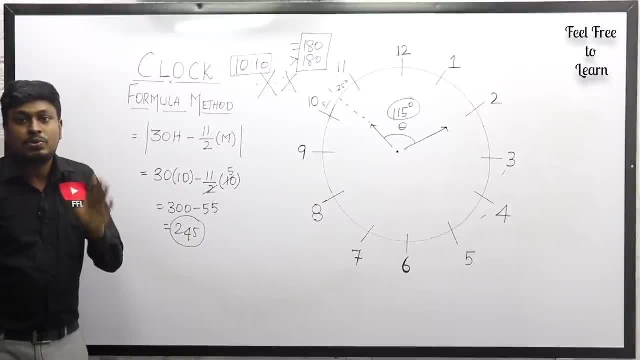 no, just now I have told you should not say the answer 245 degree. why? because the answer that we are getting is more than 180. if it is more than 180, then it is not an angle. it is called as a reflex angle. just see, here we got an answer: 245 degree. 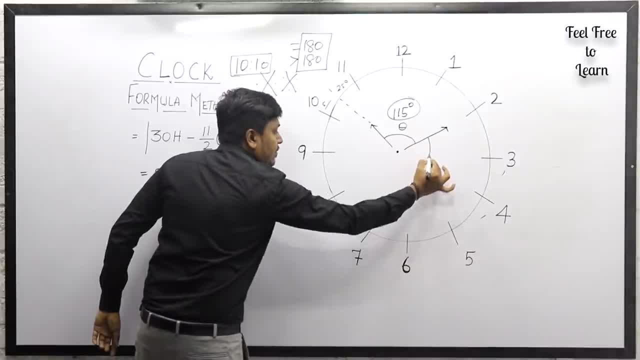 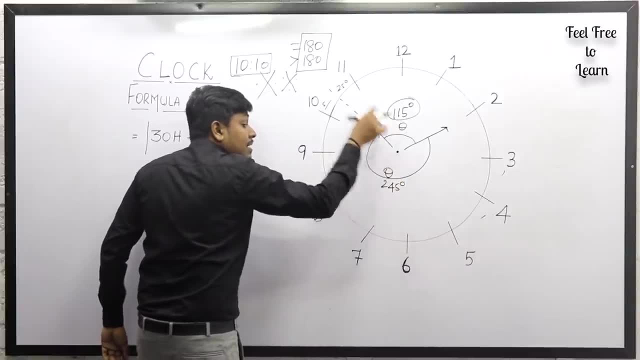 so this 245 degree is for this, understood by using a formula. we found the answer for this. that is 245 degree, but our target to get a shorter angle that is less than 180 degree. so what you need to do is: after getting this. you are not wrong, you are right. ok. 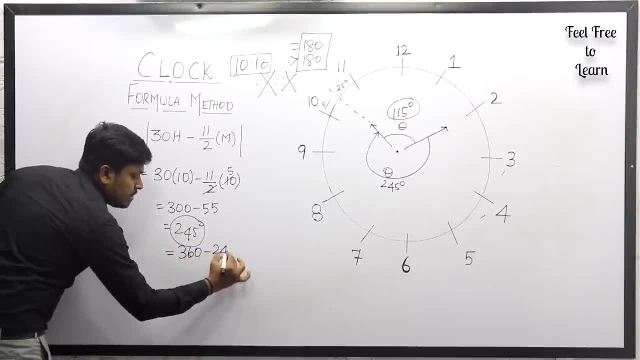 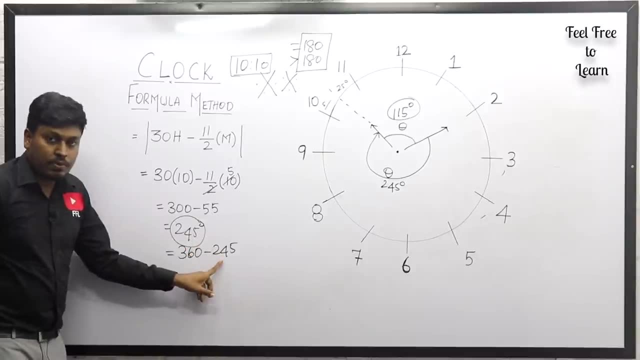 just subtract in 360. so 360 minus 245, always subtract with 360. if you got an answer more than 180, so 360 minus 245, so the resultant answer will be 115 degree. so finally you can say: answer for this question is 115 degree. 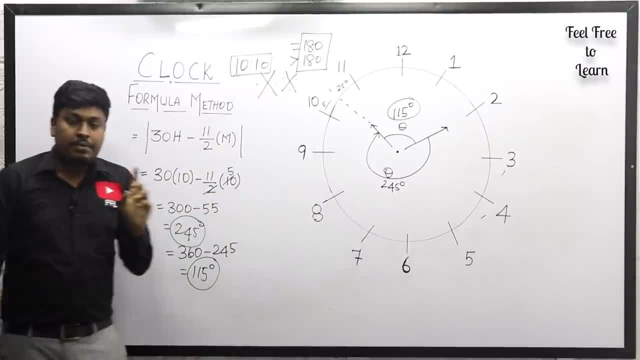 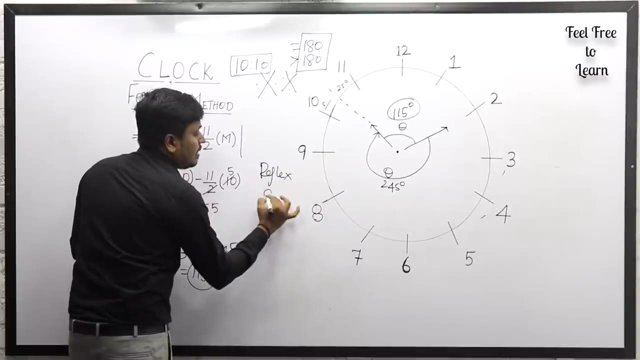 understood friends for the same question: 10, 10. if they ask what is the angle between R and and a minute, and you should say the answer is 115 degree, in case, if they ask what is the reflex angle, just see here reflex angle. so what is the reflex angle for R and and a minute and at a time of 10, 10? 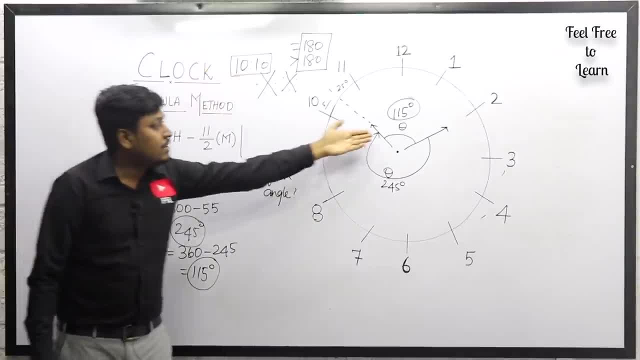 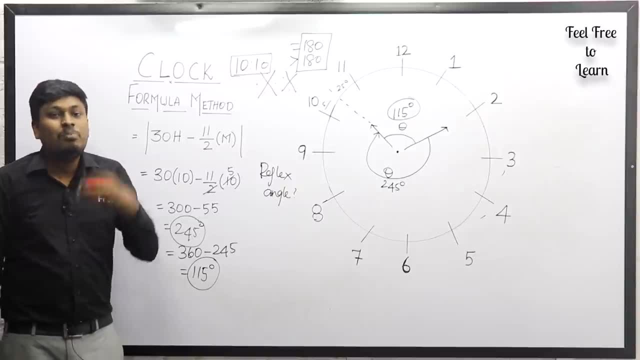 what you need to do is and what you should say: the answer. reflex angle is not this. reflex angle will be this 245 degree, so reflex angle will always be more than 180, which is called as a reflex angle, right. so reflex angle is reflex region, right? 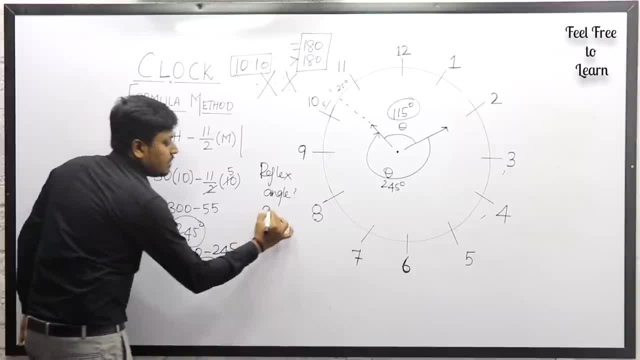 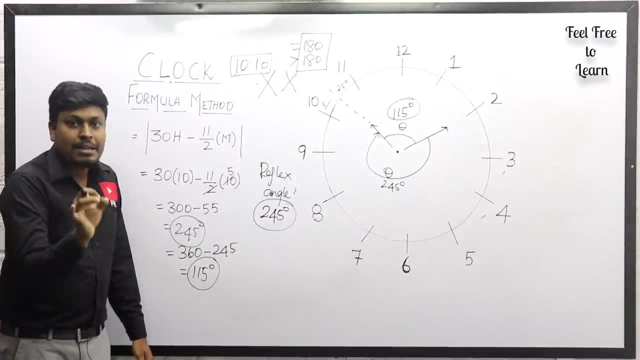 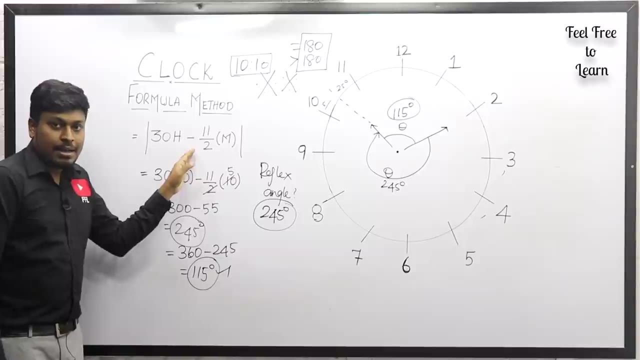 so this region angle will be 245. so answer for reflex angle is 245 degree. so only if they ask what is the angle between R and and a minute, and answer is 115 degree. so every question can be solved by a formula method. right, but only thing is the answer should be equal to 180. 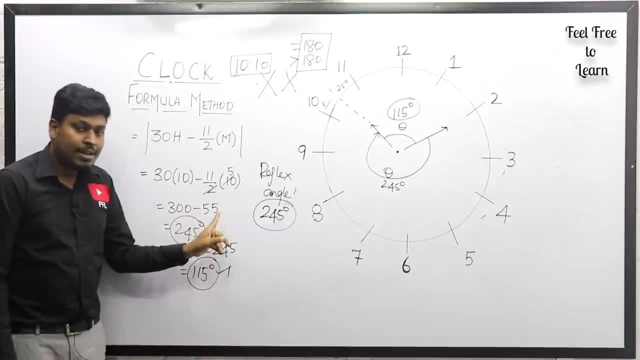 or it should be less than 180. only then you should say the answer for this question, in case, if they ask a reflex angle, always the reflex angle should be more than 180. the same question: if they ask what is the reflex angle, then the answer is not 115. 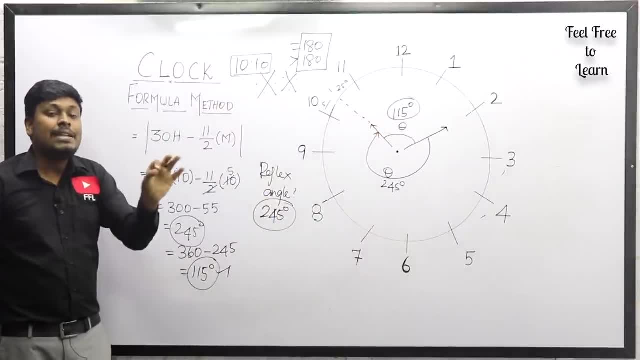 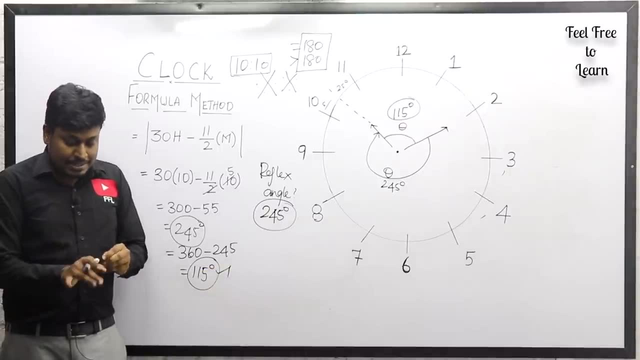 the answer is 245 if they ask only the angle between R and and a minute and the answer is 115 degree. understood, friends, clear? so that's it. in this lesson number 1. I think we have solved 5 to 6 question in a traditional method. 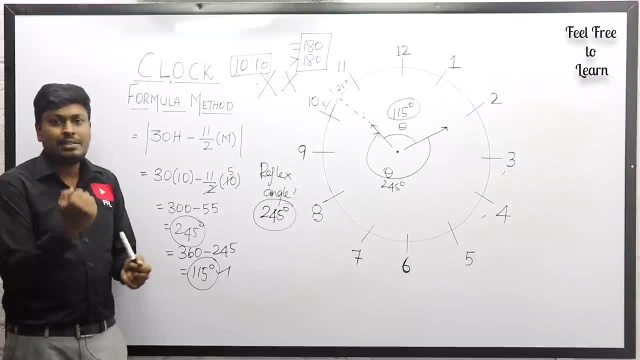 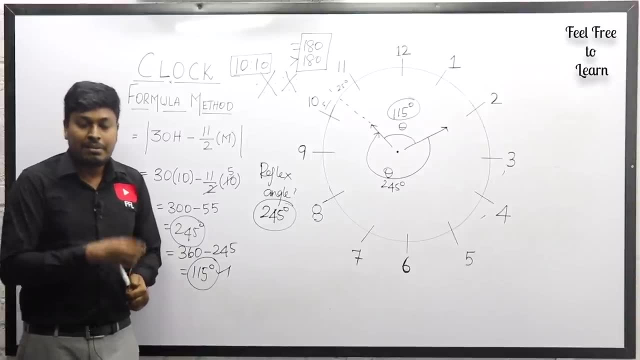 as well as I have solved that 6 question, I have picked only 3 question I have solved in a formula method and also I have explained you there are 2 important concepts where many students will make a mistake, right, because most of the students will ask me. 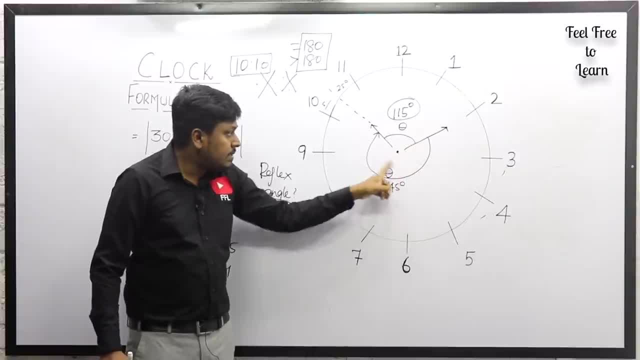 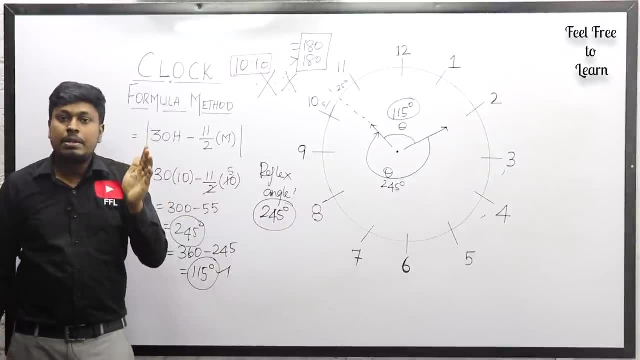 why you are taking this angle. should I consider this as an angle between R and and a minute? and just now I have told you. just keep that in mind, or take it as a small note in a paper and, before going for every exam, remember one thing: if they ask only an angle between R and and a minute and 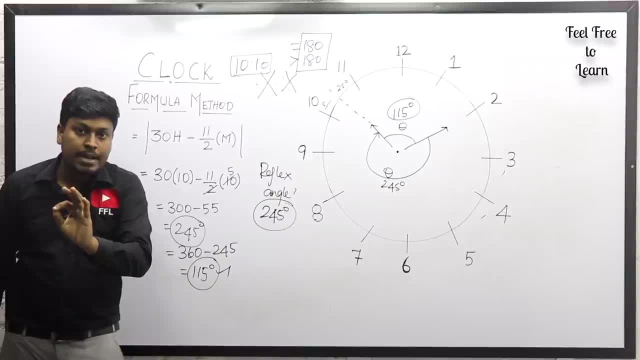 so, remember, the angle should be equal to 180, or the angle should be less than 180, in case if they ask a reflex angle between R and and a minute, and so the answer should be more than 180 degree. understood while substituting in a values in a formula. 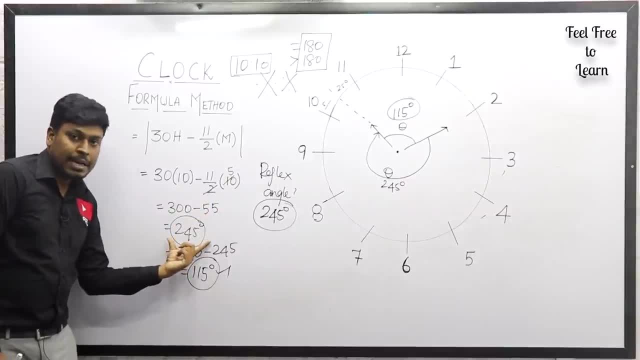 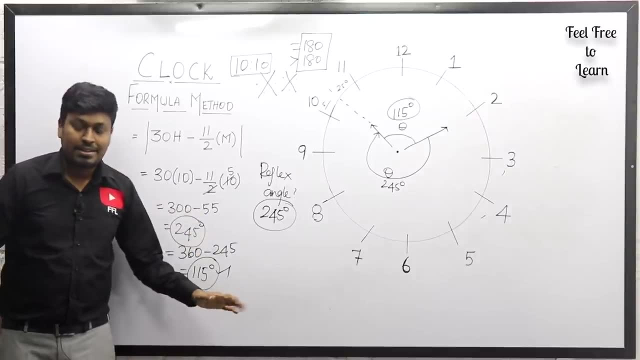 if you are getting an answer that is more than 180 degree, what you need to do is you need to subtract with 360, so resultant will be the final answer. understood, friends? so finally, thank you so much for watching this video and, if you like it, try to share the video to your friends. 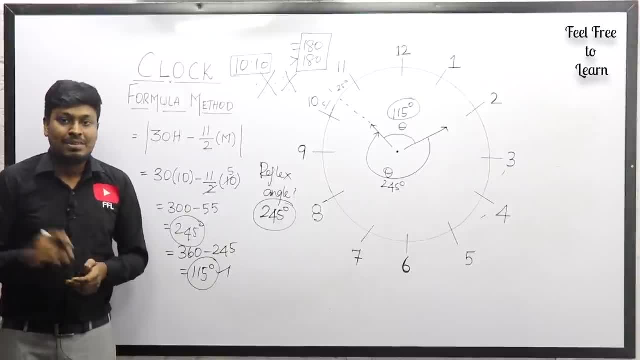 those are preparing for the competitive exams. thank you so much, bye.